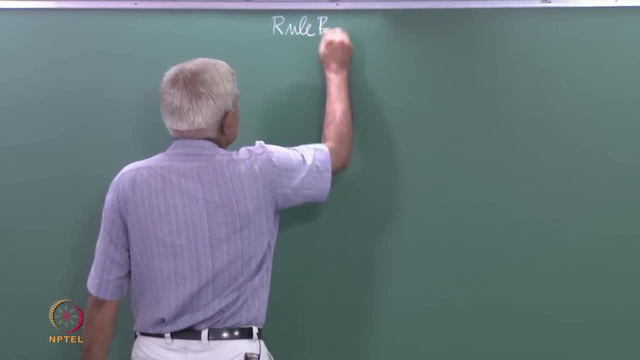 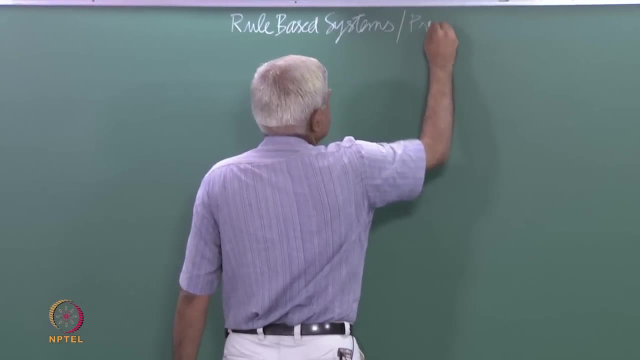 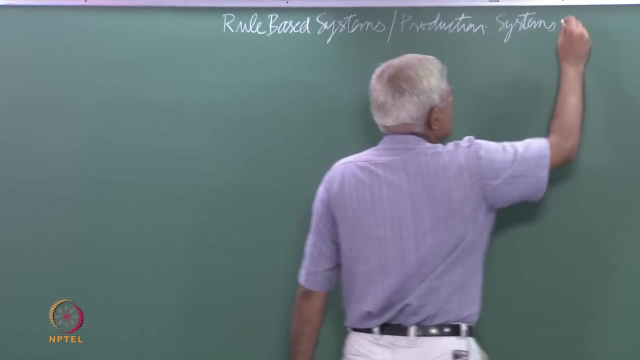 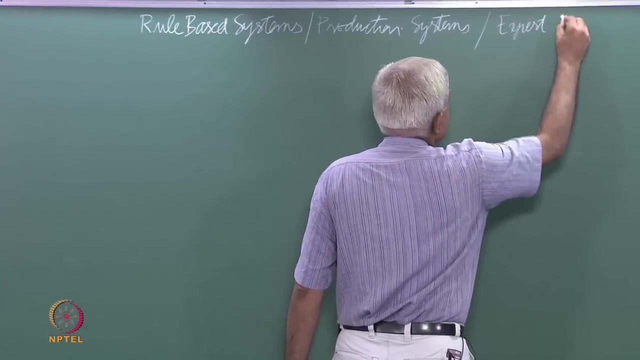 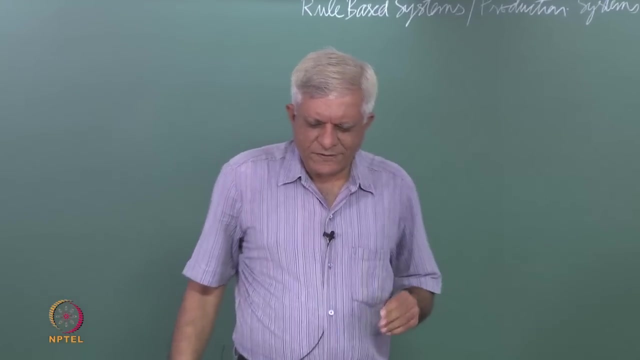 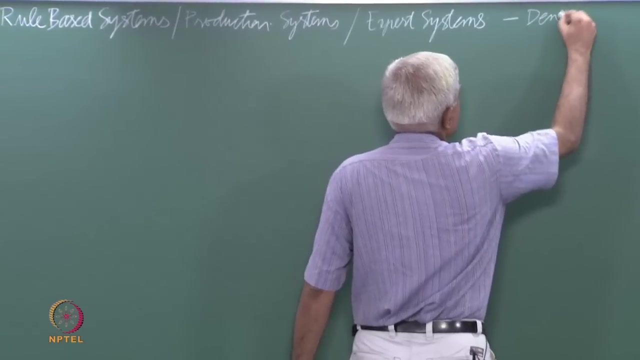 called rule based systems, also known as production systems, also somewhat ambitiously known as expert systems. So so far in our discussions we have already mentioned two systems: One is Dendrol and the other one is R 1, also known as Xcon. 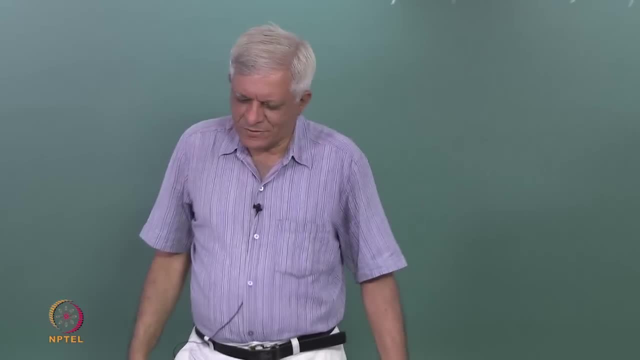 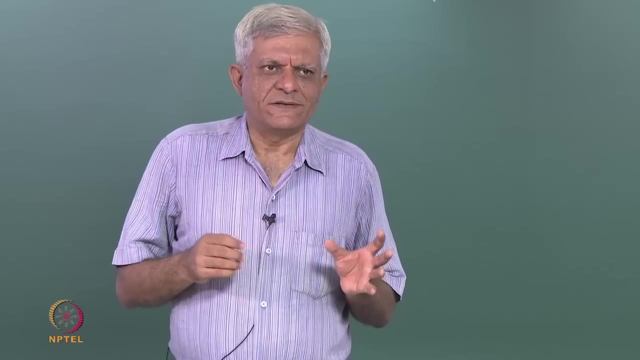 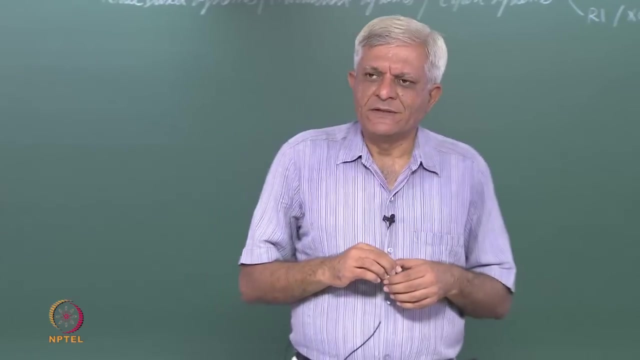 which were supposed to be two of the first so called expert systems, and by this we mean that programs which harnessed the knowledge of human experts and use that for solving problems. essentially, So, this knowledge of that we get from human experts in this form that we are talking about, was. 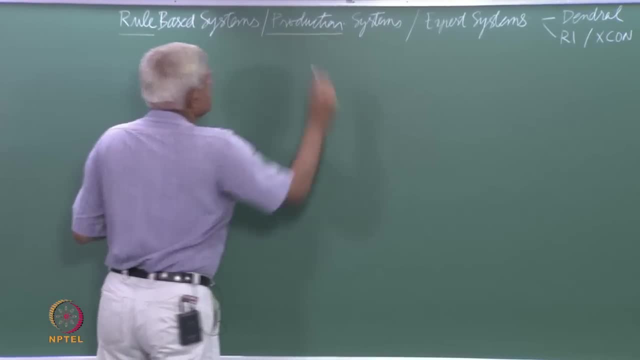 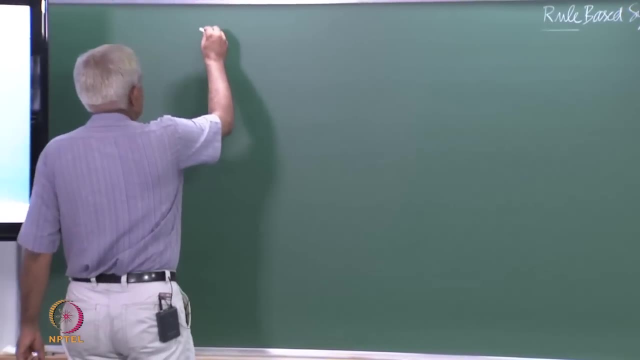 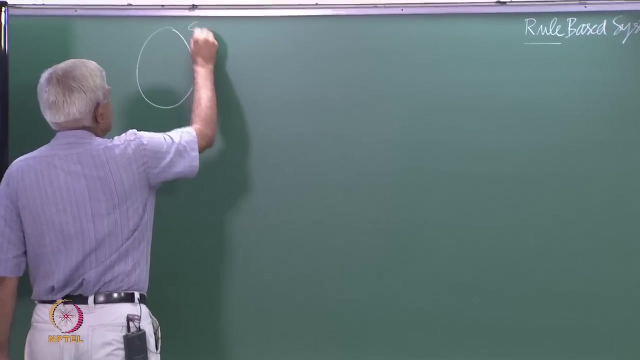 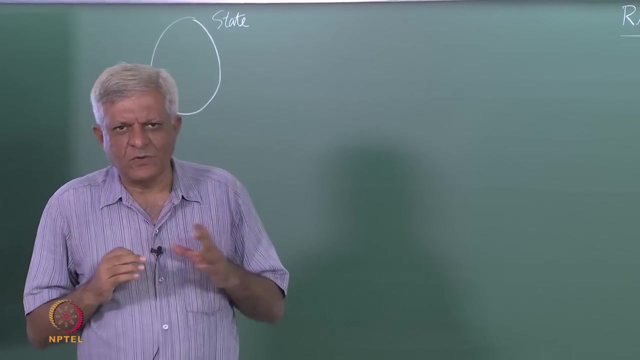 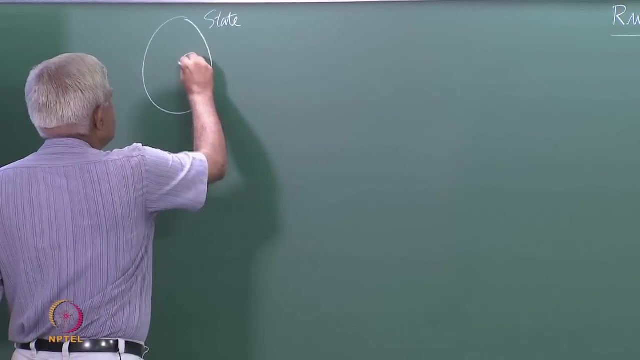 generally in the form of rules or productions, essentially, and the idea is that if you have, for example, a state description, then instead of devising a move gen function which gives, takes one state and gives you another state, what we do is we look at some part of the. 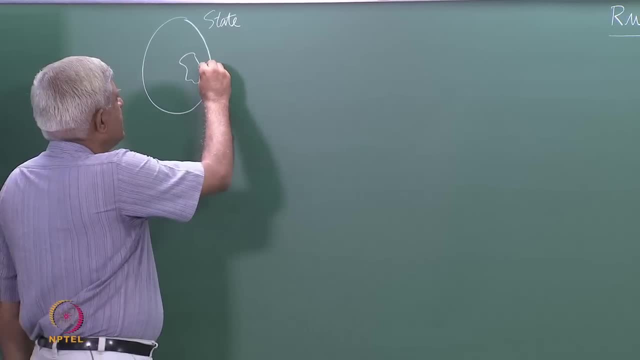 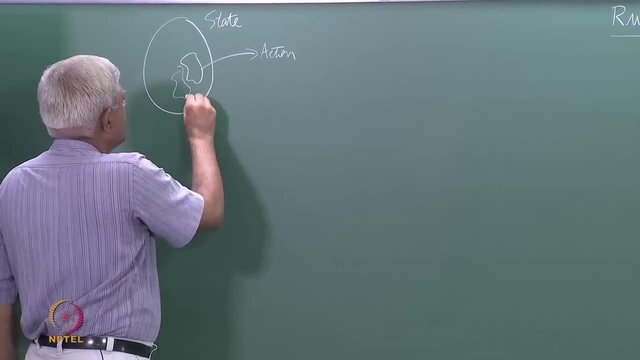 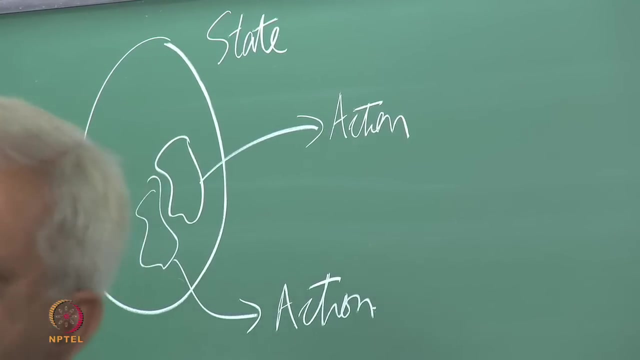 state and based on this part of the state, we devise, let us say, action one or another action one. So another part of the state we look at, we devise another action. So in some sense we are not looking at the complete state, but we are looking at what we call as a pattern. 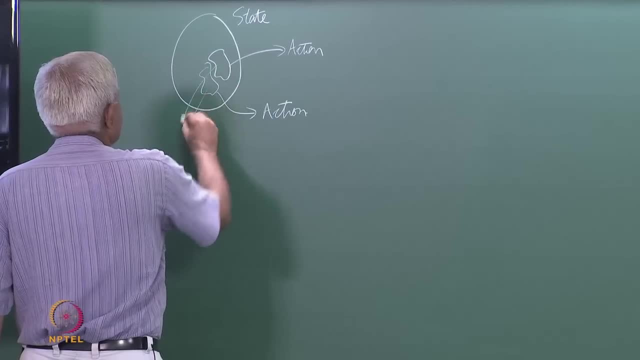 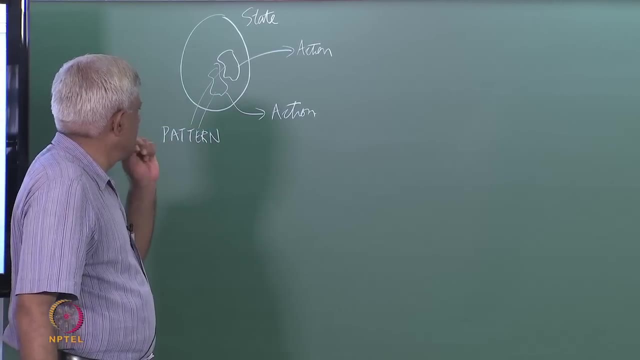 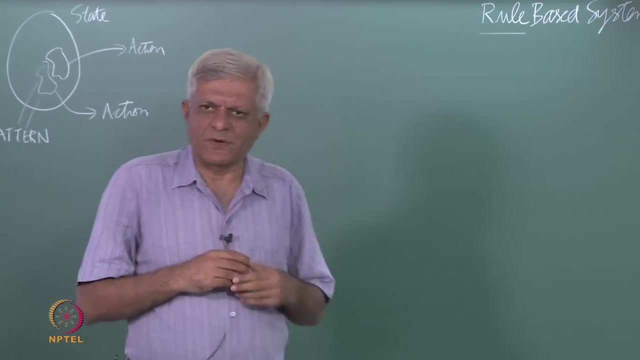 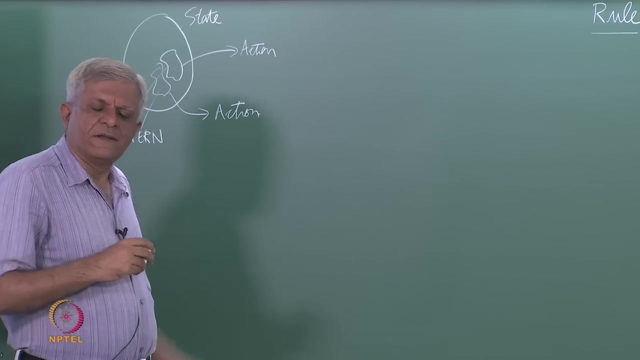 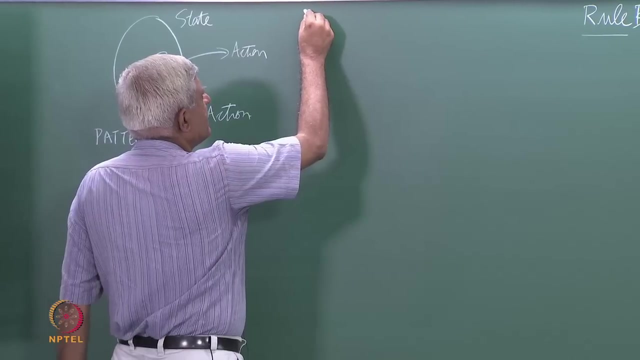 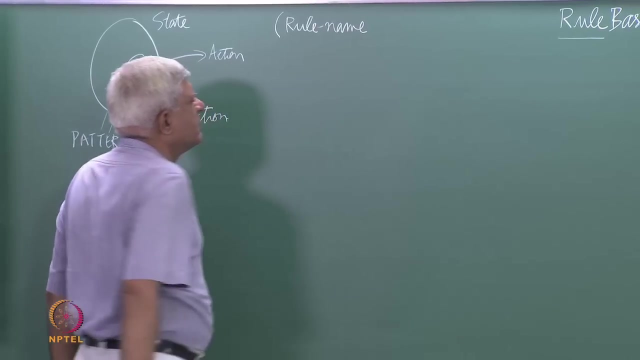 in the state. So these things are patterns. Now, this pattern is typically described in the form of a production or the rule, And I will use the syntax of a language called OPSY, which I will shortly tell you, but the basic idea is that the structure is as follows: So you have a rule name and 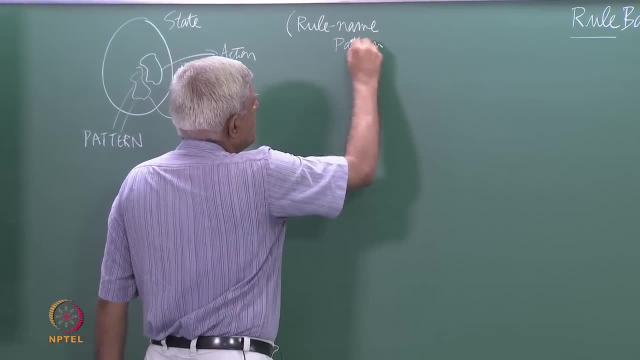 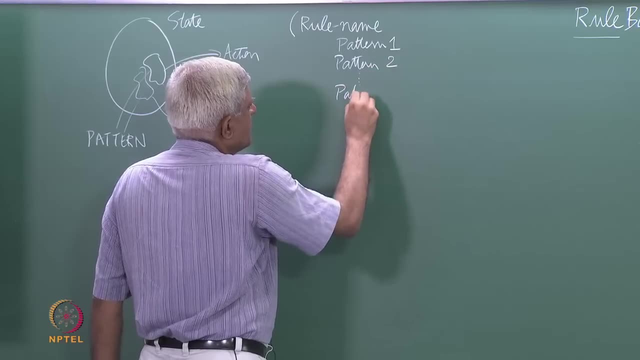 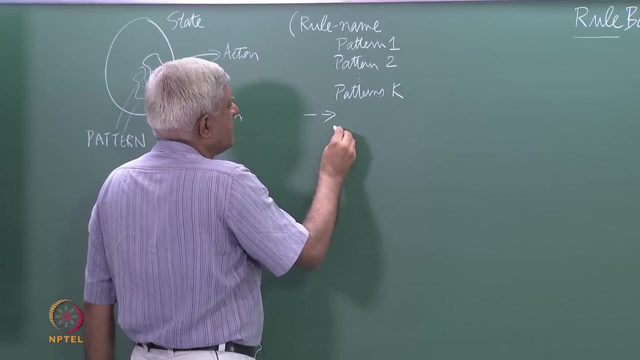 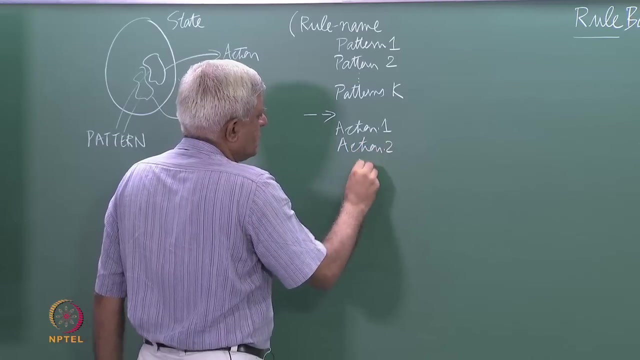 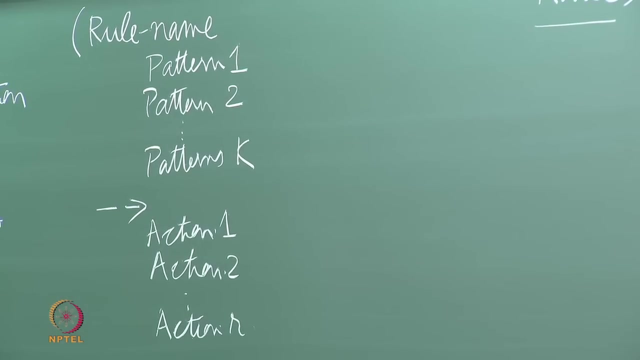 you have pattern 1, then pattern 2, then pattern 3, then pattern 4, then pattern 5, then pattern 2, and so on, some number of patterns, And I will shortly describe what these are, followed by action 1, action 2, some number of actions, essentially. So this is the structure of 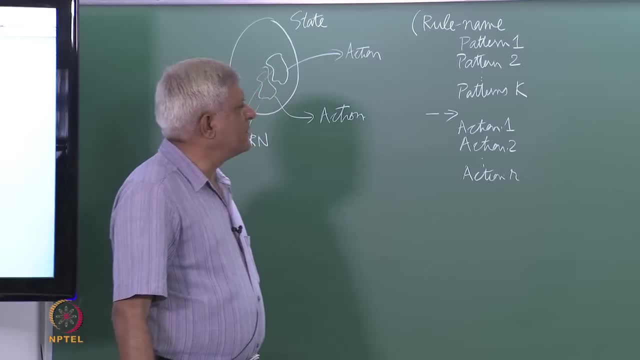 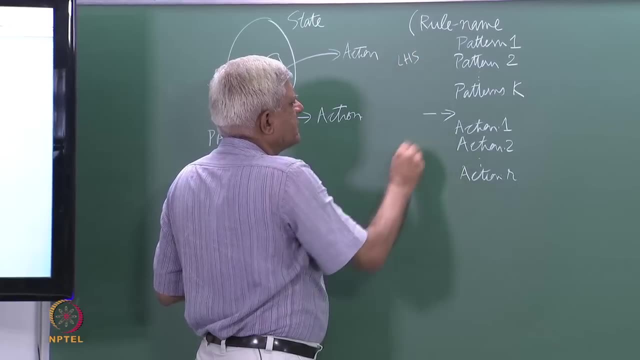 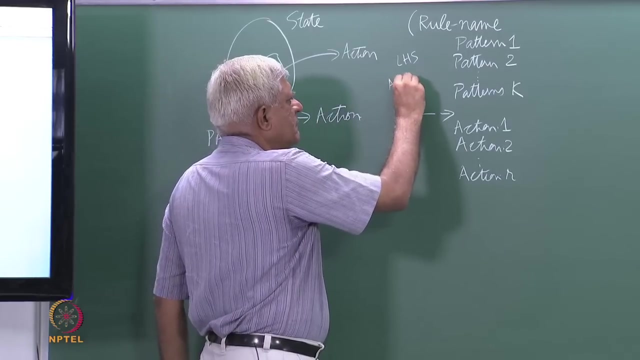 a rule, or also known as a production, And the basic idea is that this is called the left hand side. this is called the right hand side because of the arrow here. This is also called the antecedents, and we can. 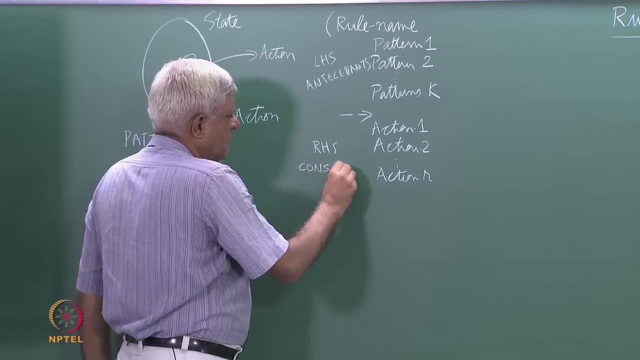 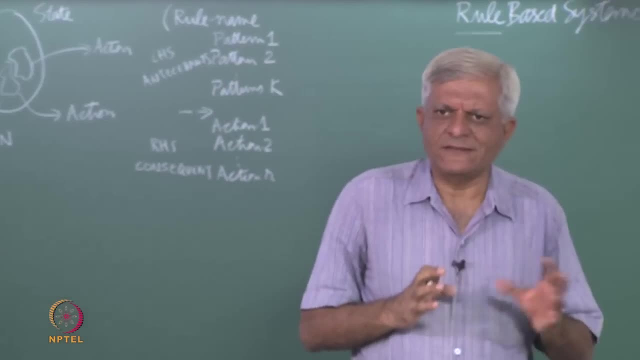 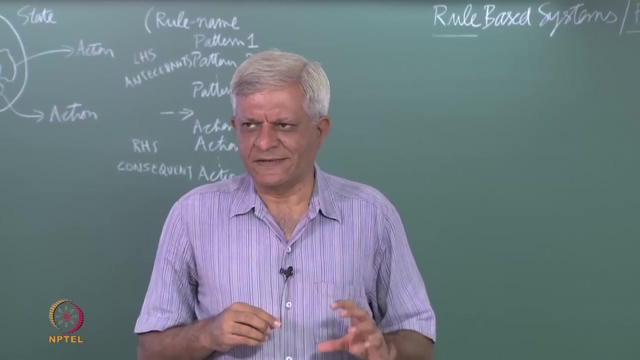 think of this as a consequent. So a rule is basically a set of antecedents followed by a set of actions or consequence, and it is a very modular form of knowledge representation. We have so far not used the word knowledge representation at all in this course. We have 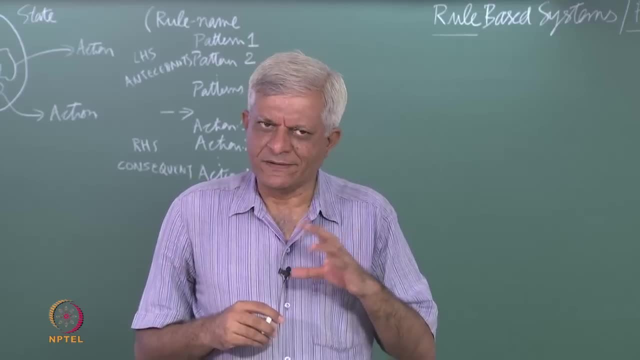 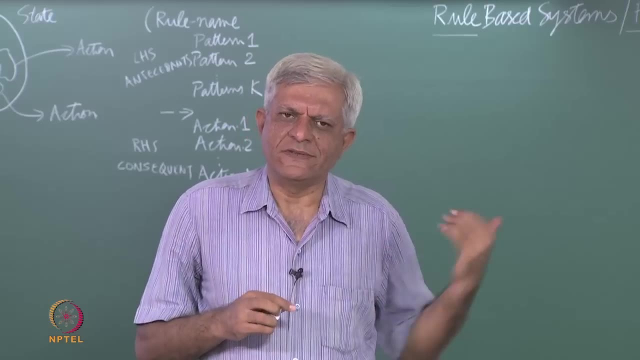 assumed that somehow you will have a state representation and somehow you will have a move gen function which will move from one state to another. Now, with this, for the first time, we are talking about how do we actually represent things? 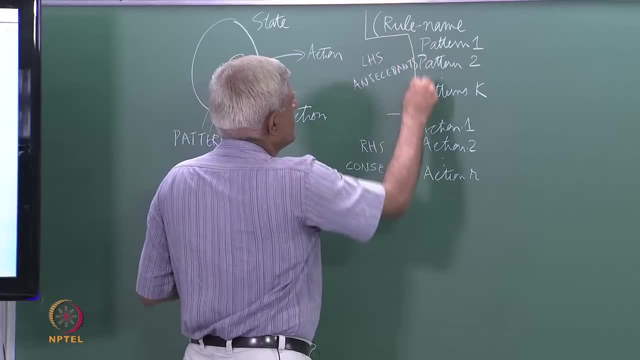 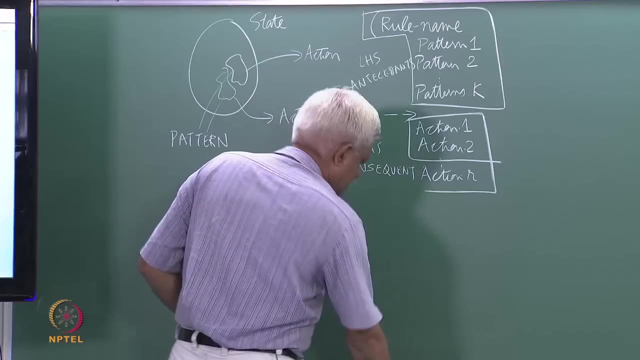 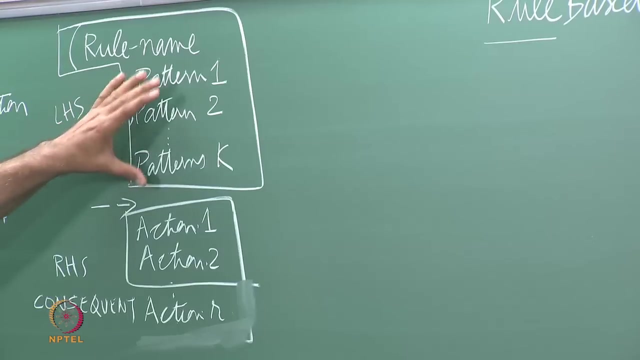 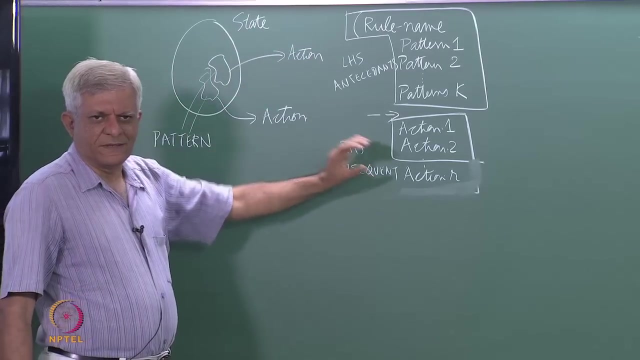 So the rule is that knowledge is represented in the form of rules. So where you have the left hand side followed by the right hand side here. So the left hand side that we are talking about here is essentially the pattern that we are looking at, and if the pattern matches, then the action can be done. So 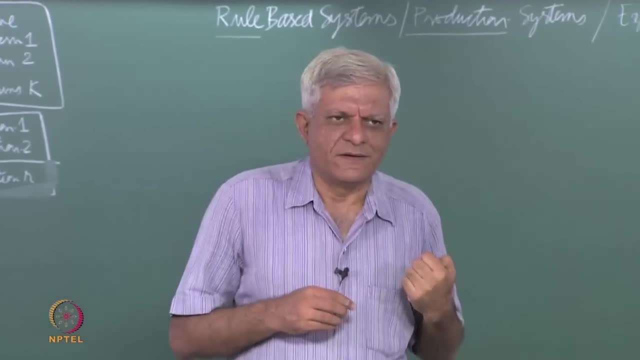 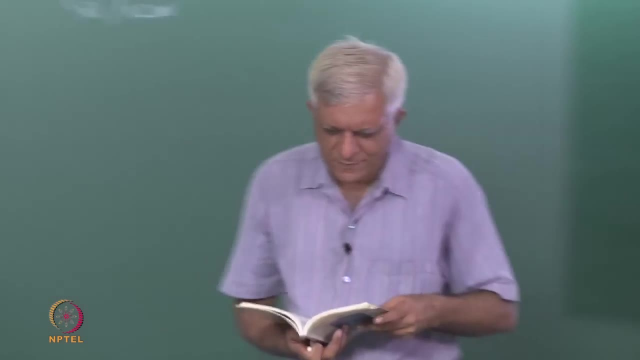 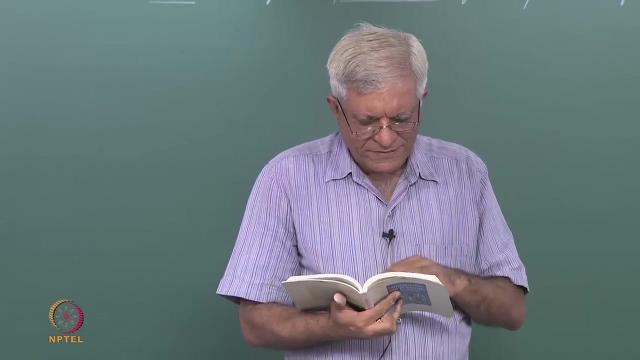 for example, the system R 1, had rules like: so you should look up the actual rule in x con or may be. I can just read out a rule from here. This says: this is a rule from R 1,. its rule name is distribute m b device. 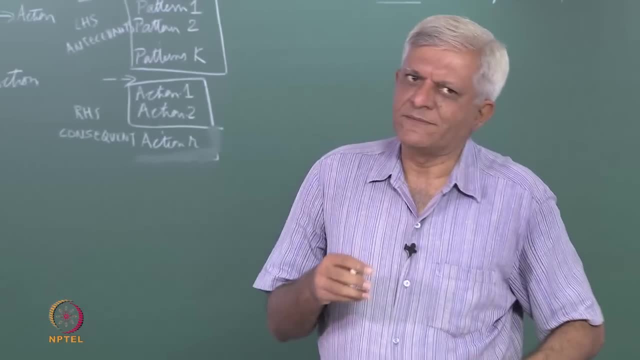 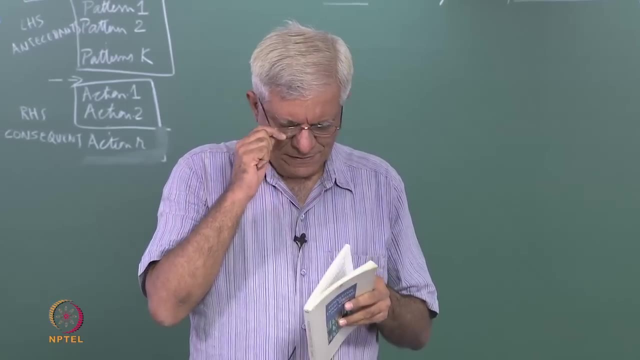 3.. So remember, R 1 was a system which was used to configure wax machines, deck wax machines, which were some of the most advanced computing systems at that time, which was in the late 70s, And this rule reads the following: 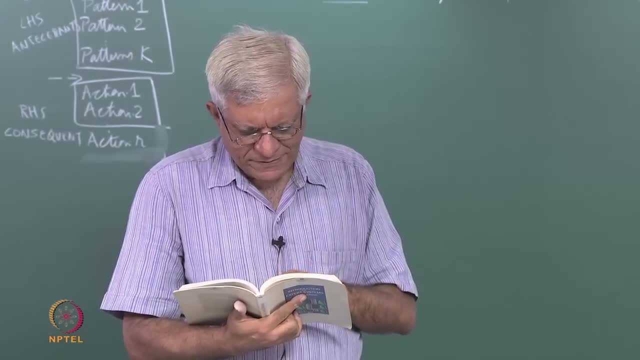 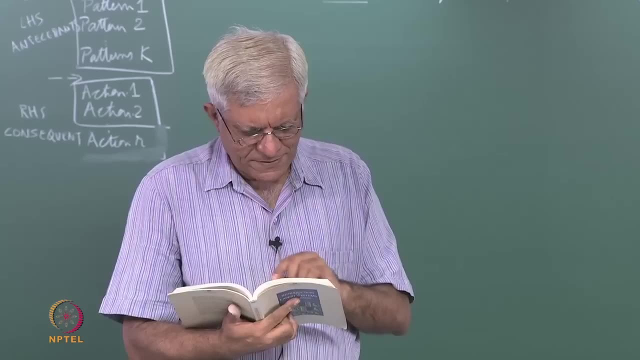 if that is the left hand side, the most current active context is distributing mass bus devices, and there is a single port disk drive that has not been assigned to a mass bus and there are no unassigned dual port disk drives, and so on and so forth. And then the 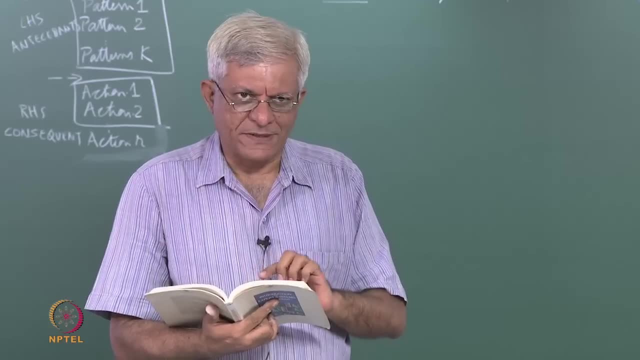 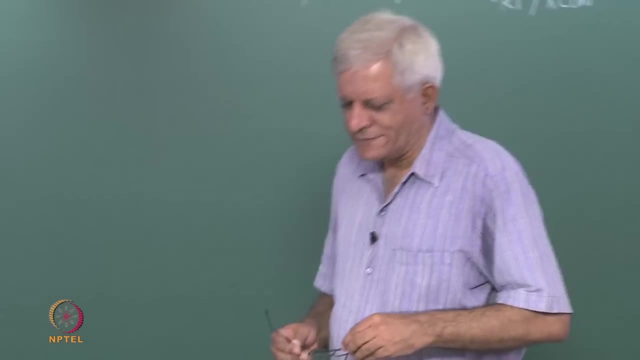 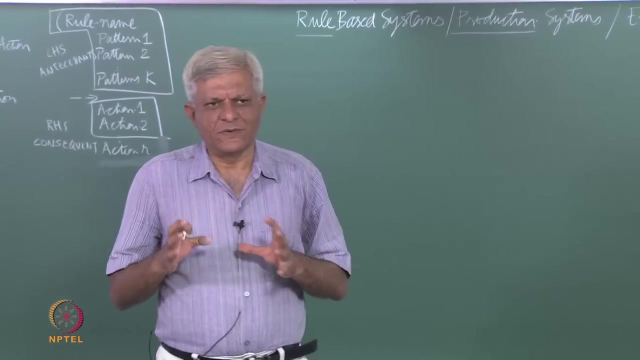 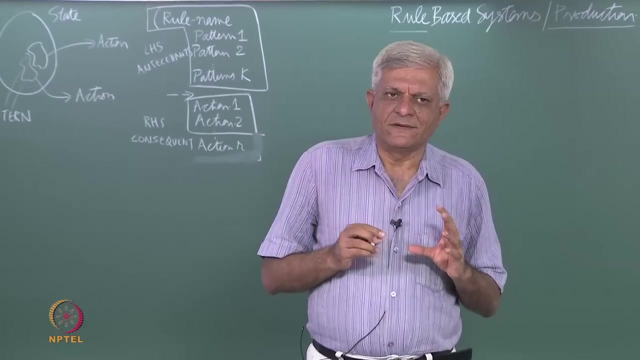 action is then assign the disk drive to the mass bus, So it has a set of conditions on the left hand side and, in this example, only one action on the right hand side. essentially So, the idea is to capture knowledge of a human in this form and use this knowledge. 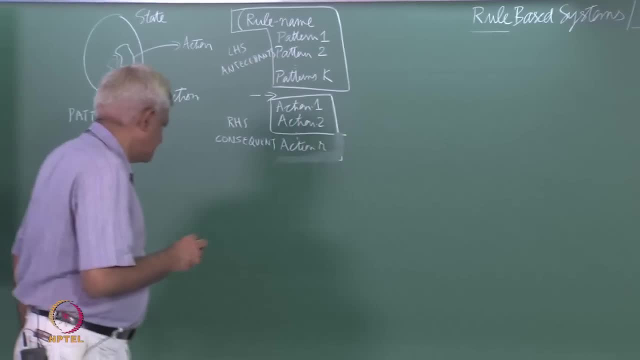 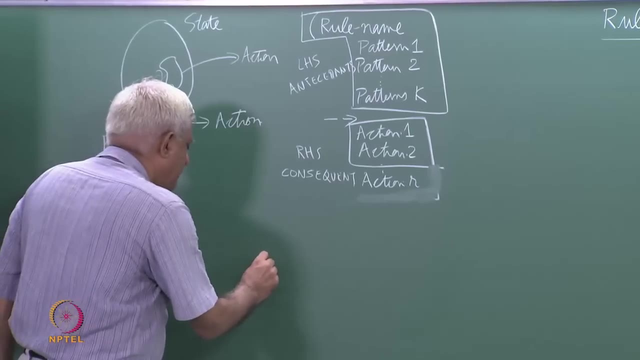 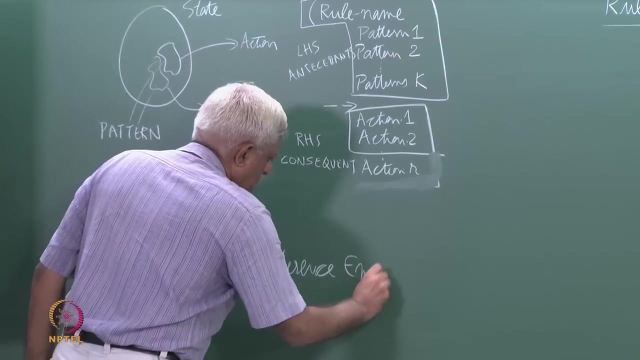 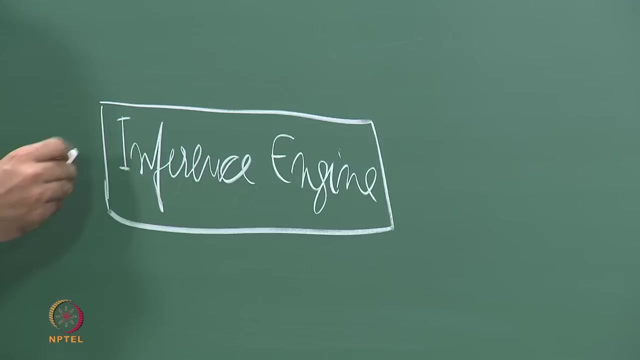 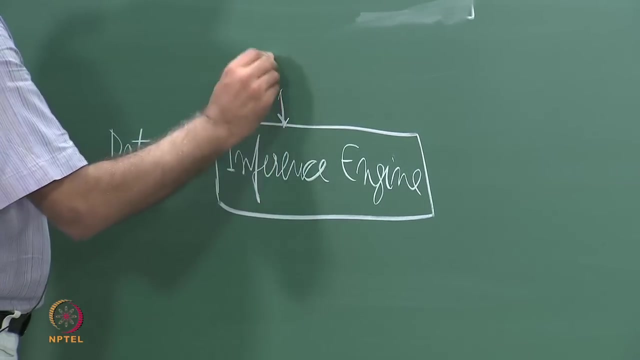 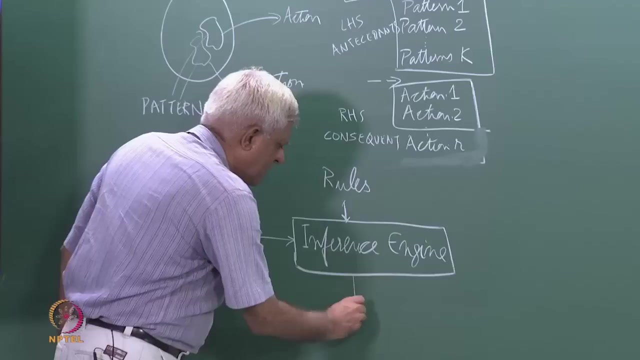 to solve problems. Now, how does that happen? So there is this idea of an inference engine, and this inference engine takes, on the one hand, data and, on the other hand, rules, and it generates the- I will just use a loose term to say the solution or a sequence of. 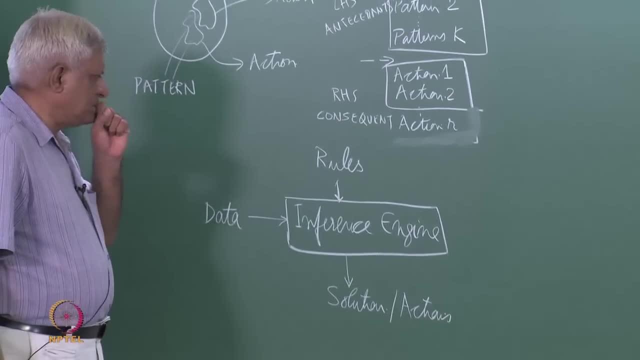 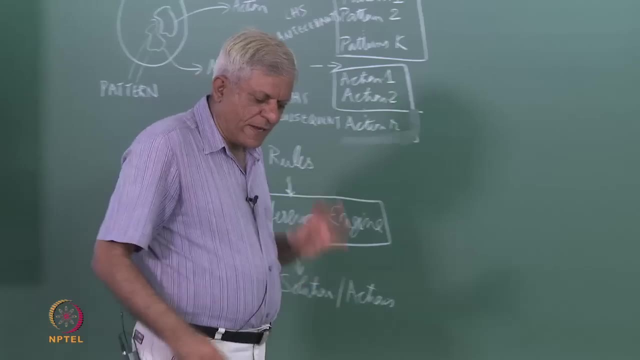 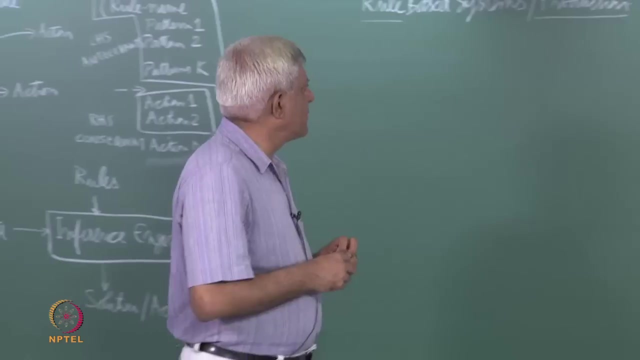 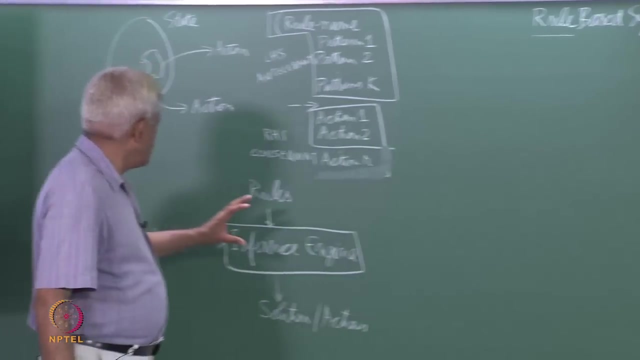 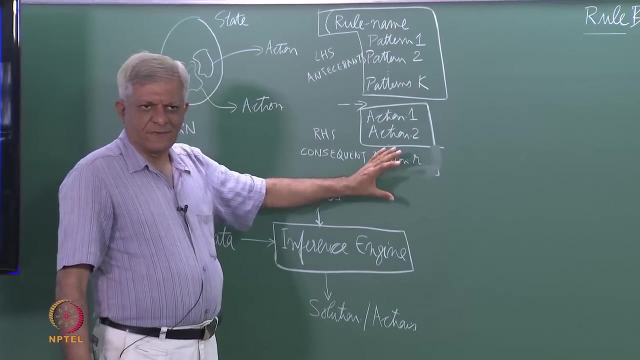 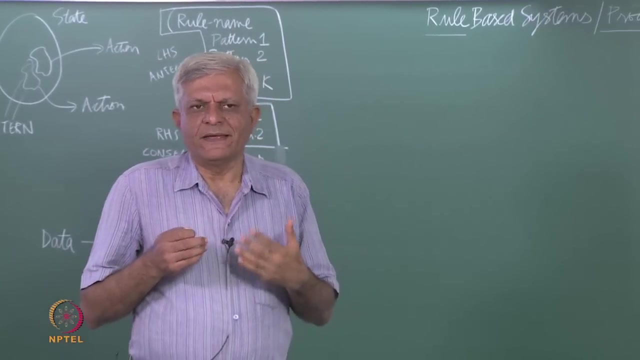 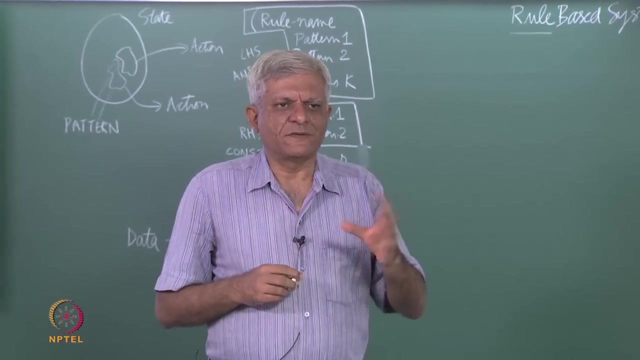 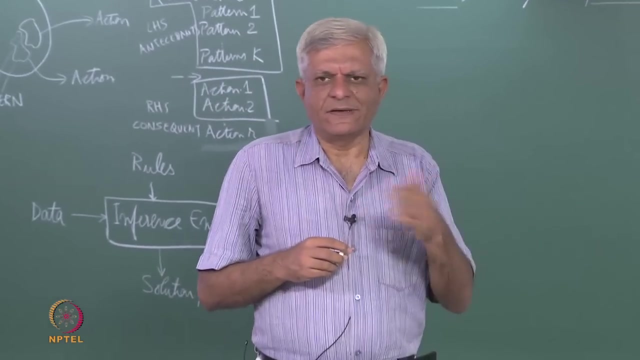 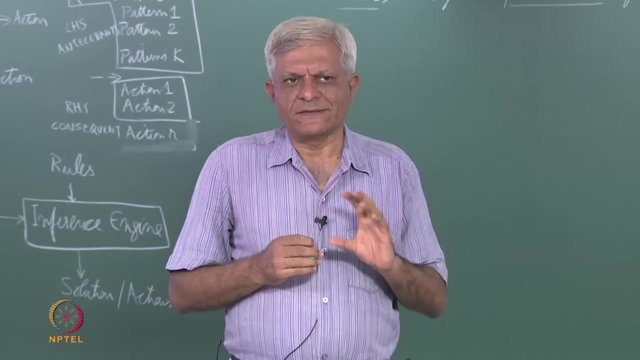 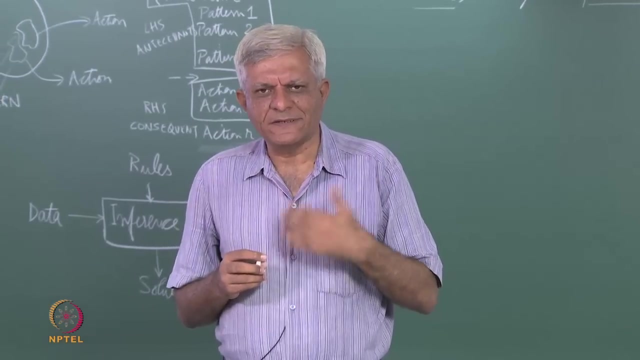 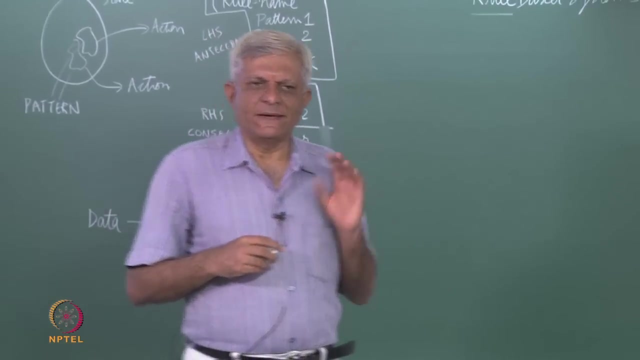 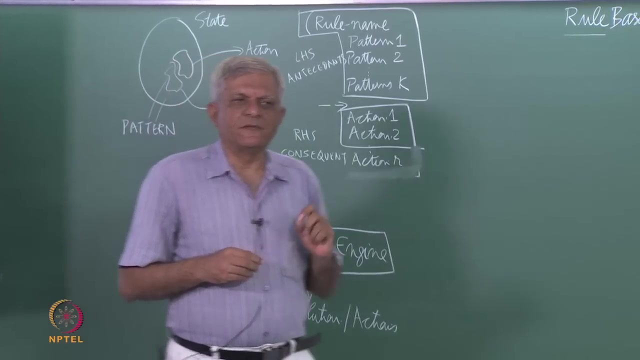 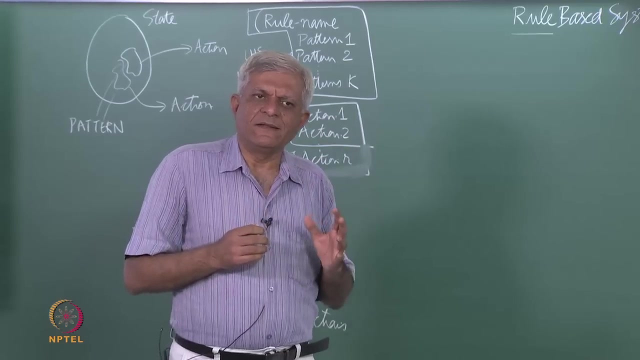 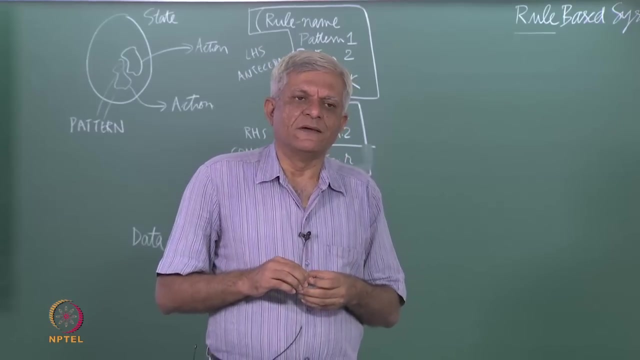 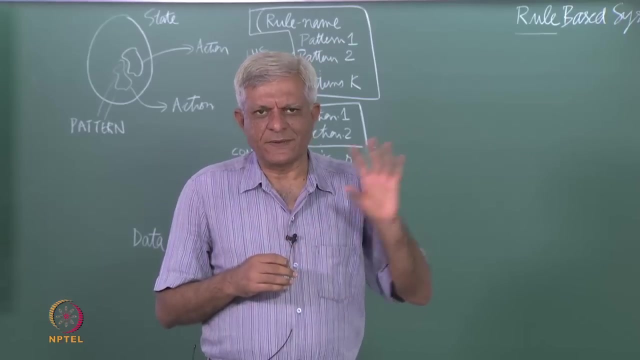 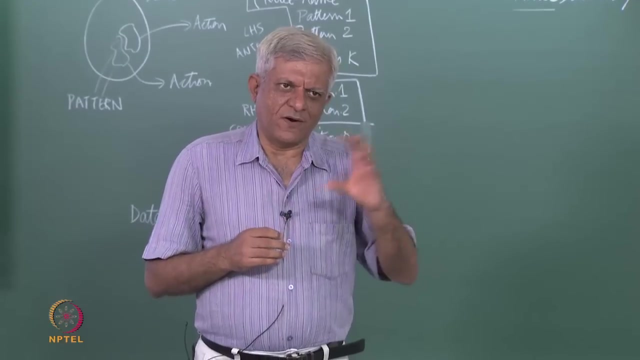 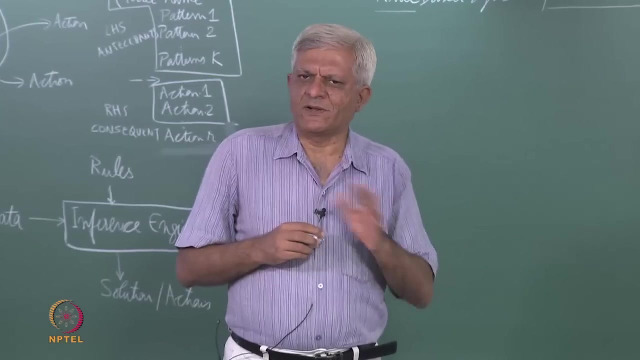 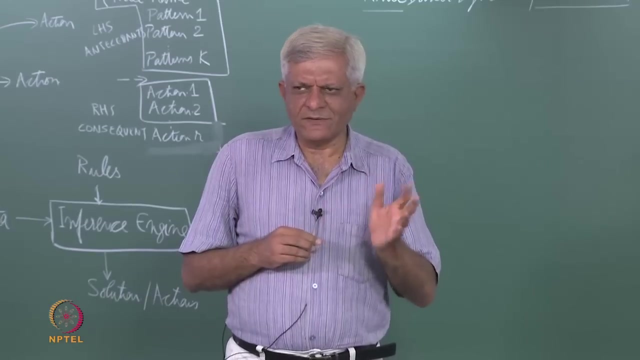 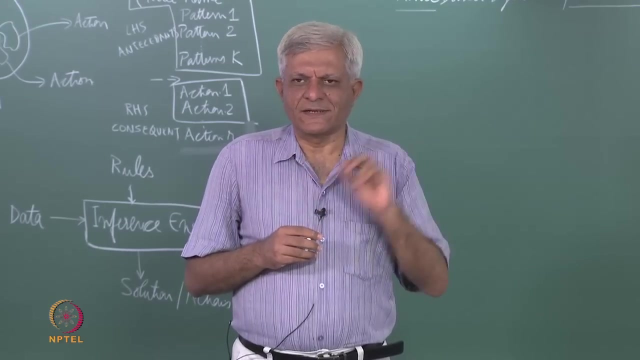 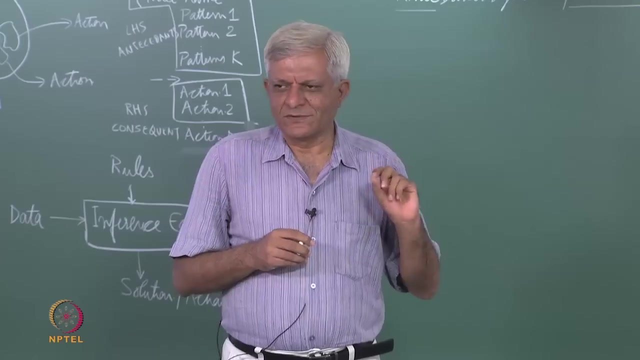 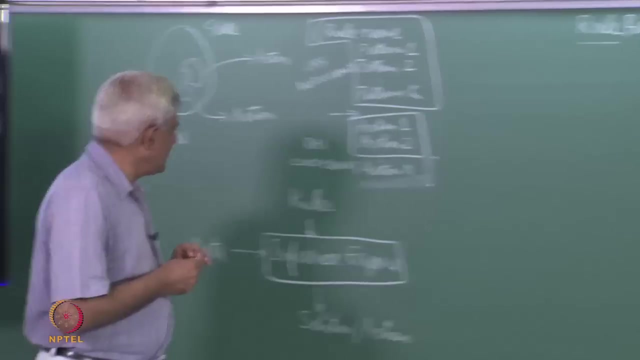 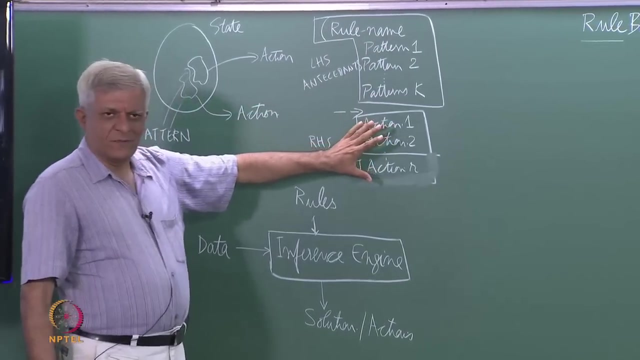 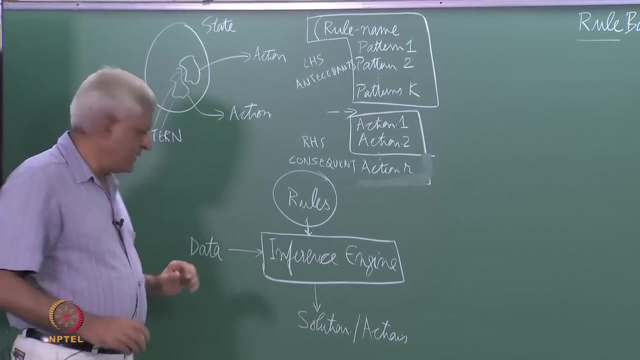 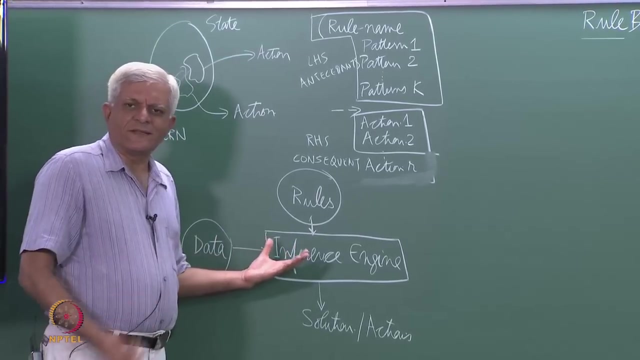 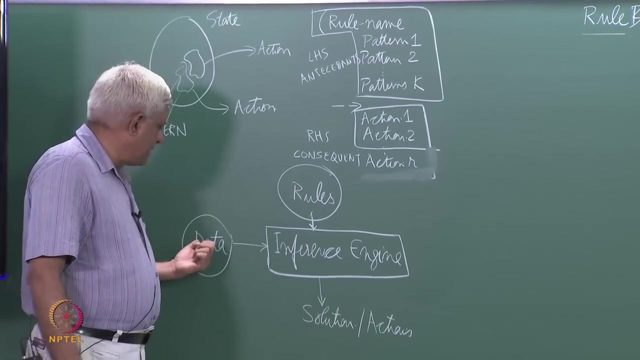 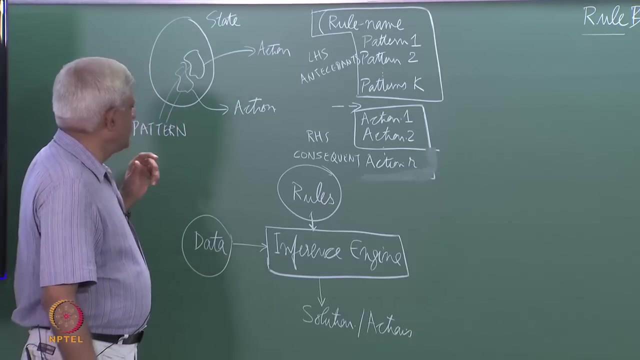 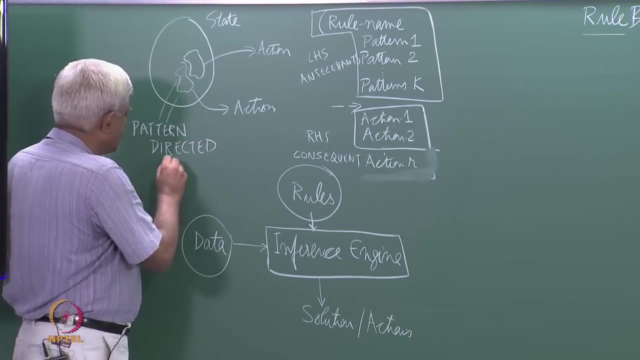 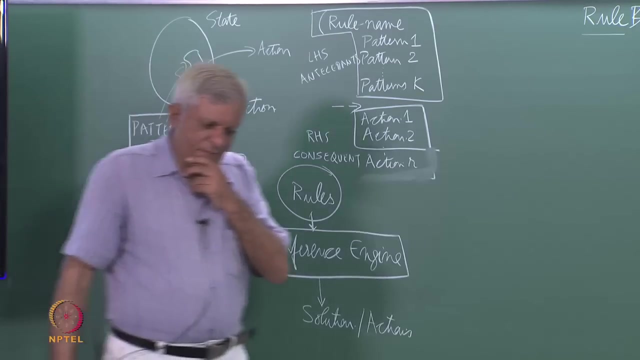 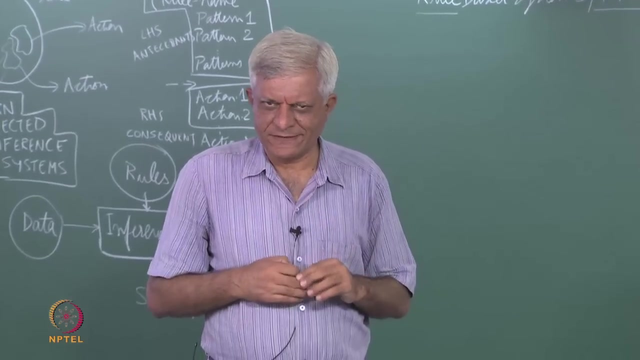 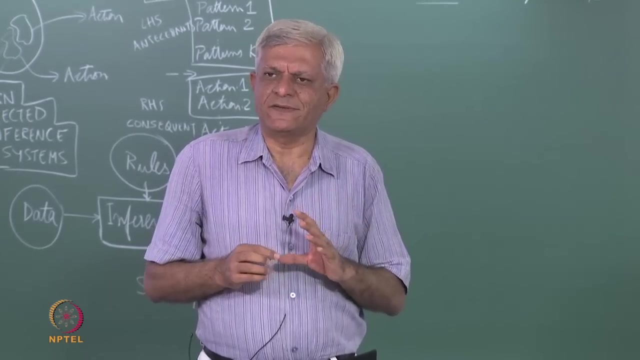 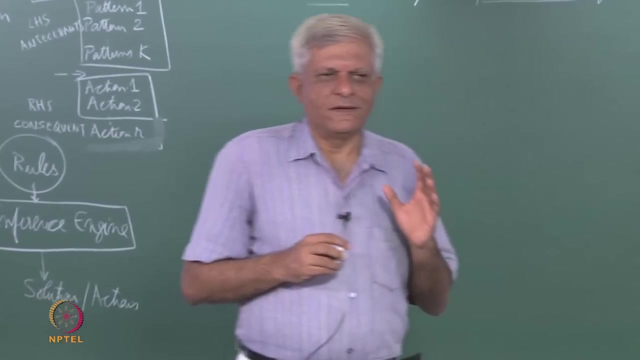 actions, When in the program which is about most people. 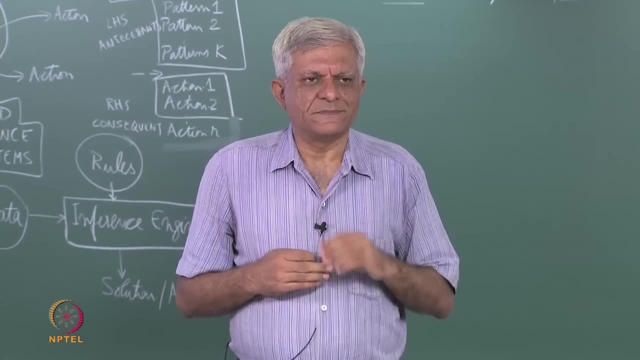 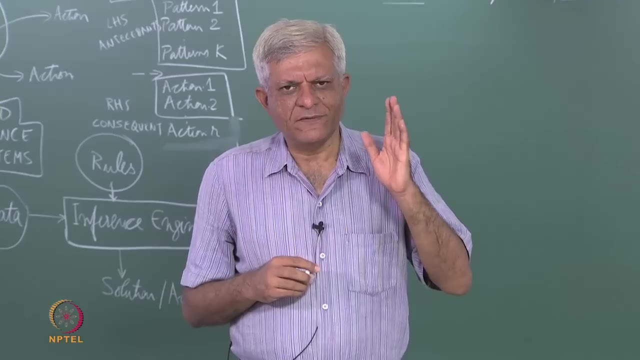 are used to languages like C in Pascal and so on. the task of the programmer is to give a control flow, say: do this action. 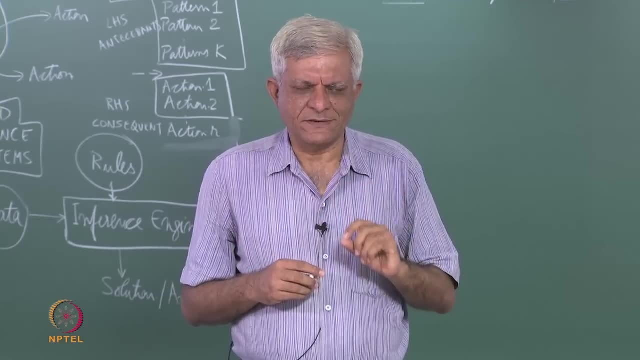 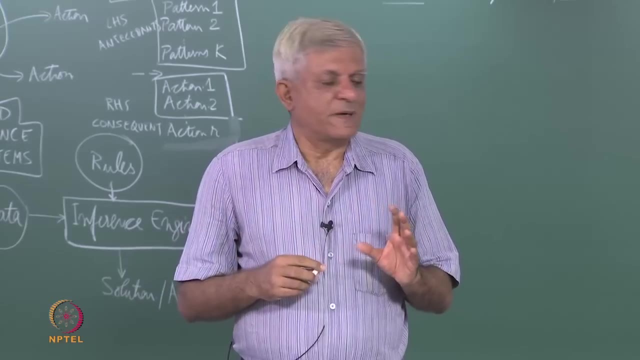 role. Say: do this action, then do this action, then do this action. Of course you may have more complicated things like conditional statements and branches and loops and all this kind of stuff, but it is the programmer which specifies what actions have to be done. 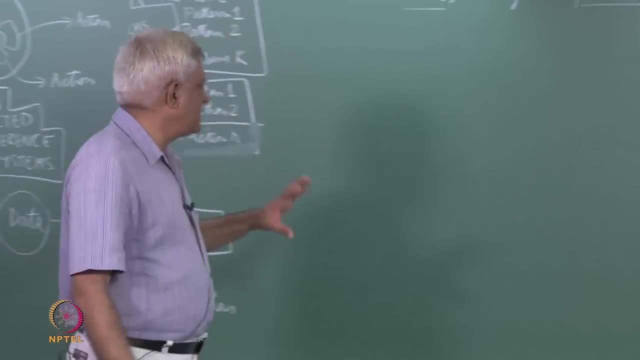 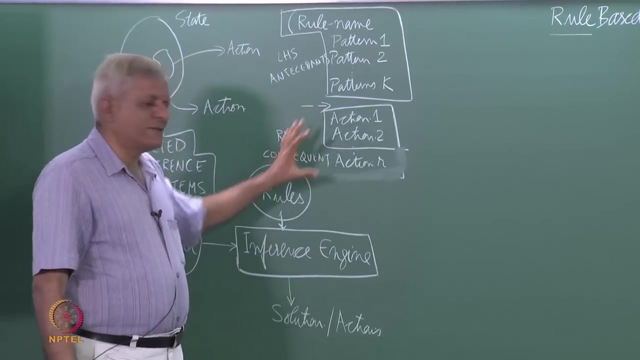 Now you can think of a rule base system. you can in some sense port it to an imperative language, and you can so remember that the rule base system basically consists of a large number of rules that the domain expert writes. You could convert it into an imperative. 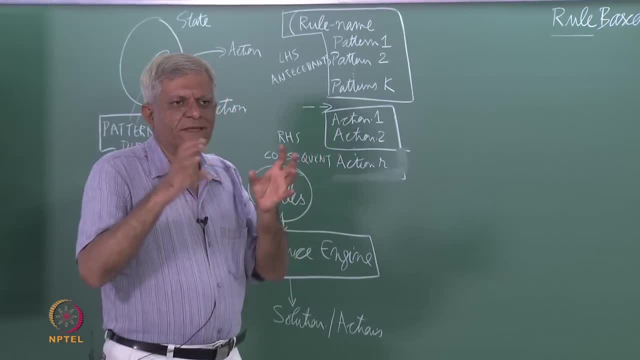 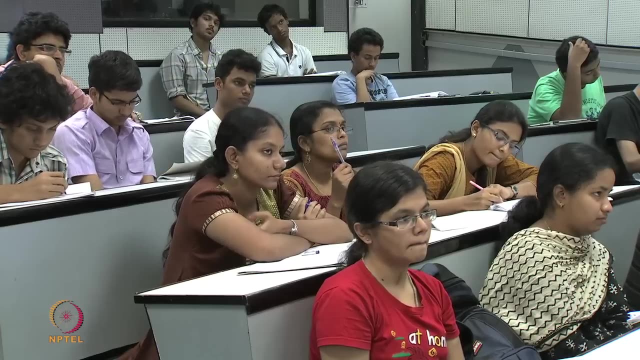 program and you could have a sequence of if, then statements, if this then this, else this, then this, and so on and so forth. The control flow is fixed and rigid in imperative program, In rule base systems. on the other hand, you can think of this as follows: that 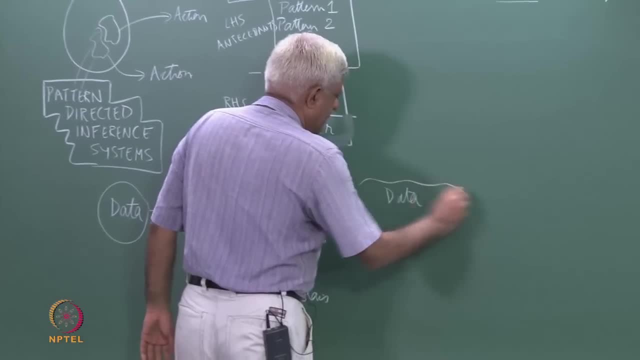 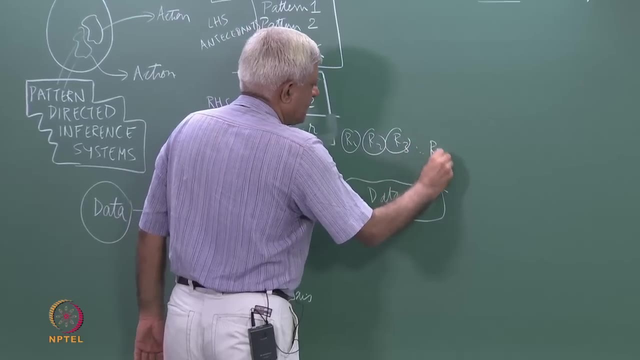 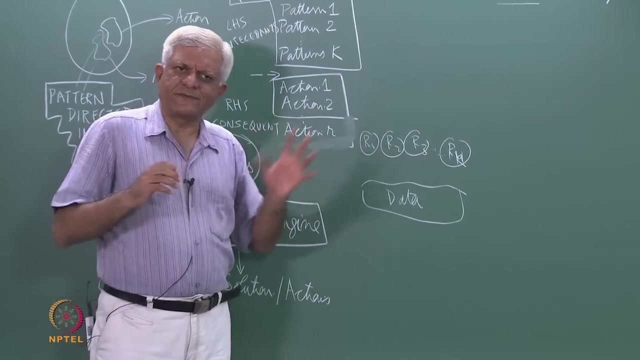 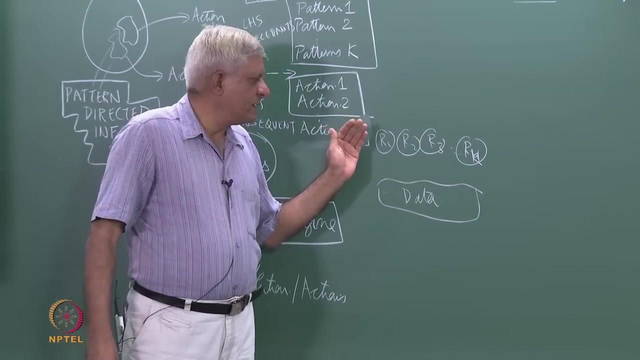 you have this data in some pool and there are set of rules hanging above this. And when I say hanging about this, it has to sort of make you think about it slightly differently, in the sense that there is no control, There is no relation between the different rules. You are not saying: apply this rule. 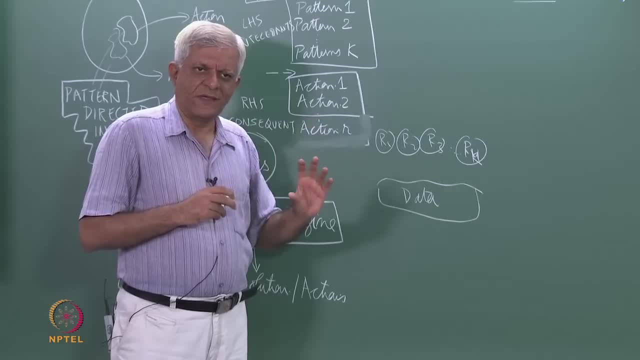 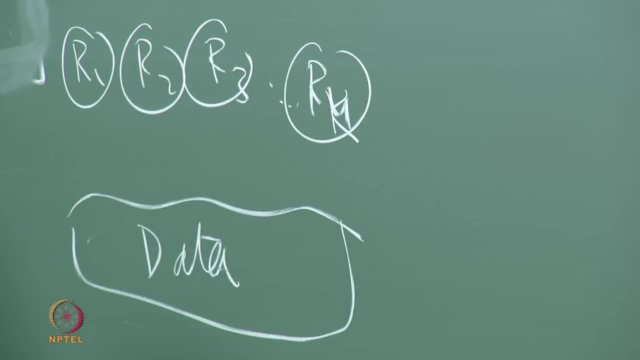 first and then apply this rule first, and then apply this rule first, and so on. You are simply saying, in each rule you are giving a little bit of modular piece of knowledge which says: if you see this pattern, then this is the action that you have to do. essentially, 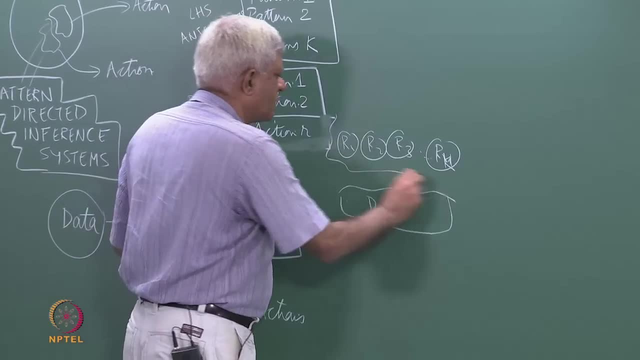 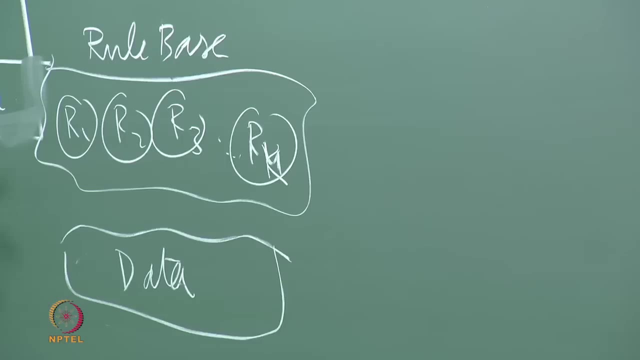 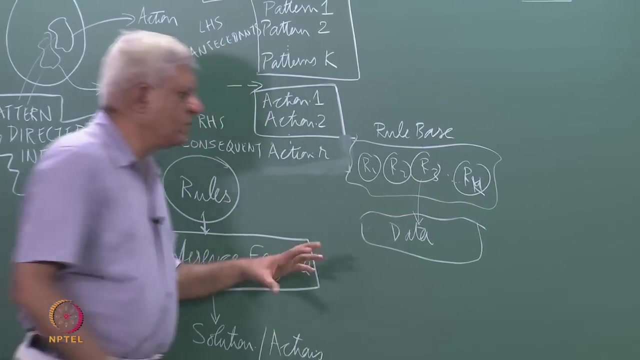 And all the rules are kind of floating around. So this is what we would call as a rule base, And what the inference engine does is that it would pick some rule and apply it to the relevant data and do the relevant action. Then may be pick another rule and apply it. 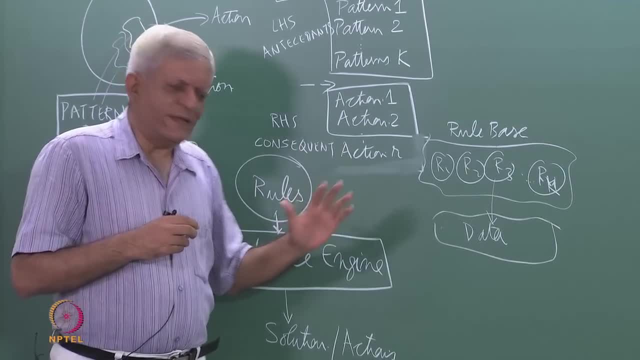 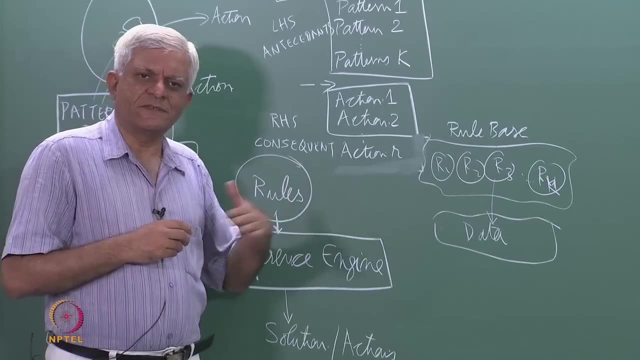 and so on and so forth, and it will keep doing that. It is an inference engine- and we will look at this in a little bit more detail- which decides what are the actions which are actually done as opposed to in imperative programming. who programmer says: do this action. 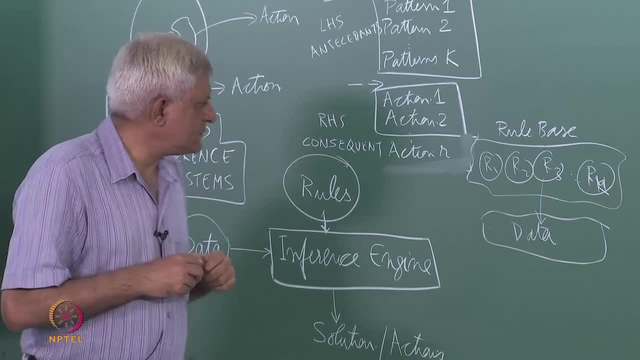 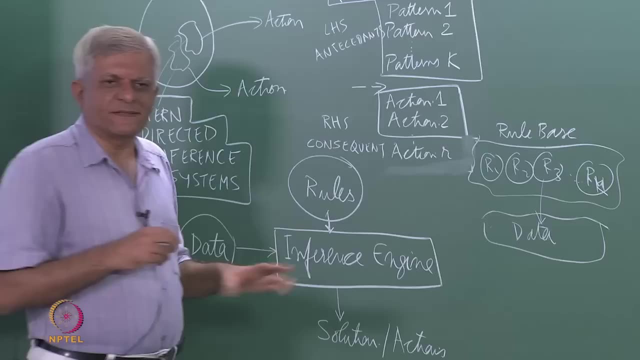 then you do this action and so on and so forth. So I am not finished. I had some questions. Now I will leave it aside and will carry on. So, before we get into the details, I also want to highlight a difference between two. 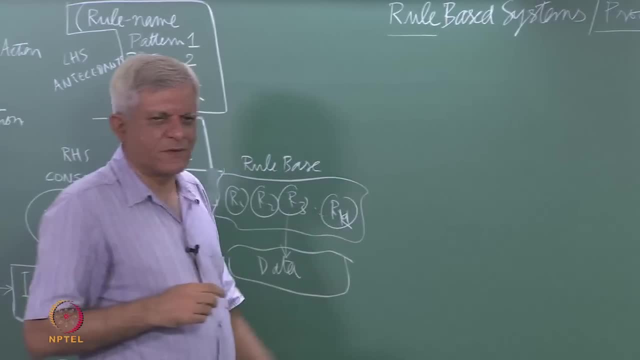 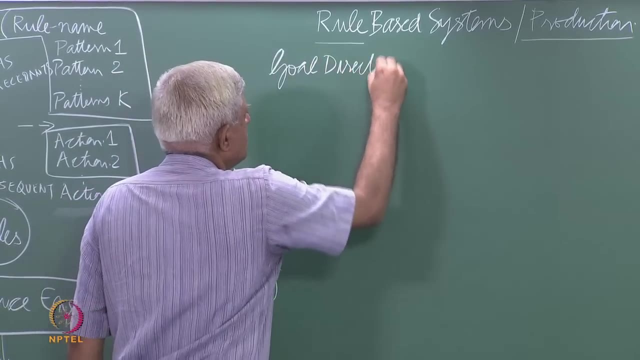 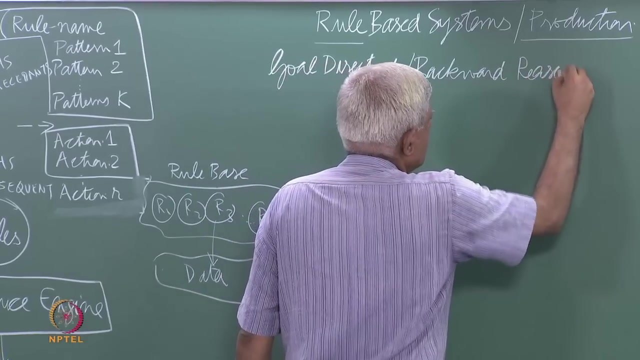 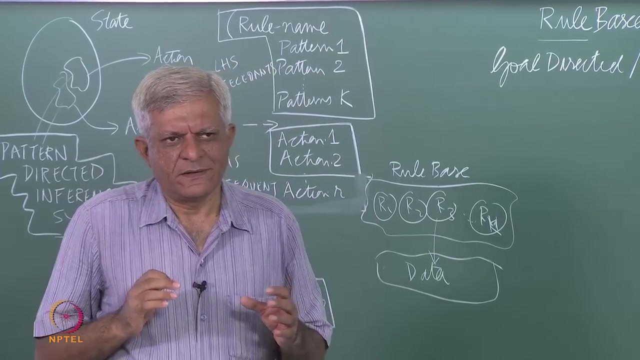 kinds of reasoning, and we have slowly talking about reasoning. we have not really done so. One is goal directed or backward reasoning, and by this we mean that you reason from goals to sub goals. in some sense We have already seen an example of this, when we are talking about planning an evening out. 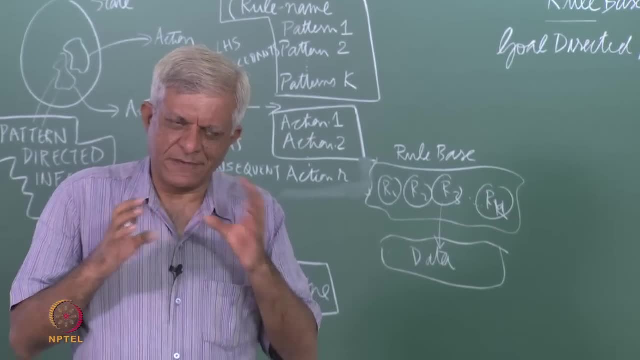 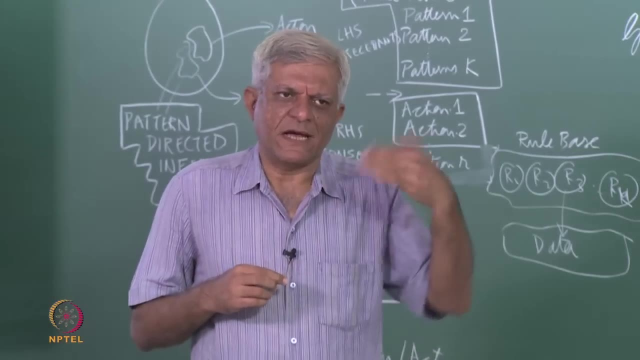 and you said that an evening out is planned. So if you have an outing plan and if you have a movie plan and if you have a dinner plan, so those are the sub goals essentially. So you start with the major goal and then you come to the sub goals essentially. 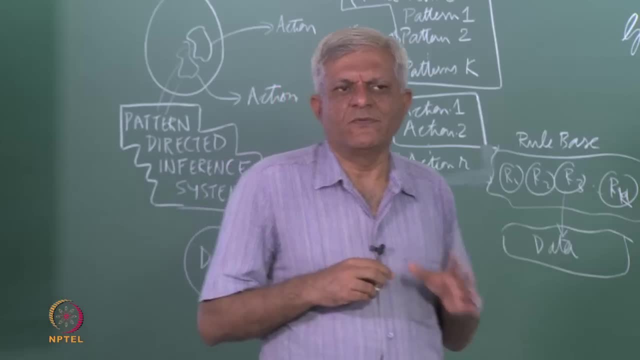 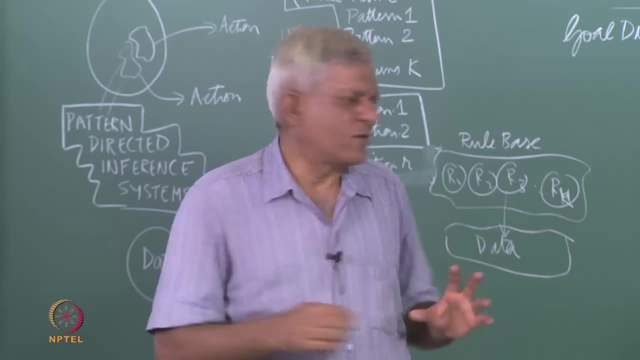 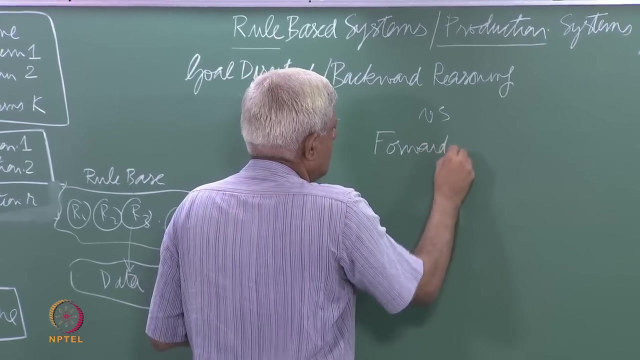 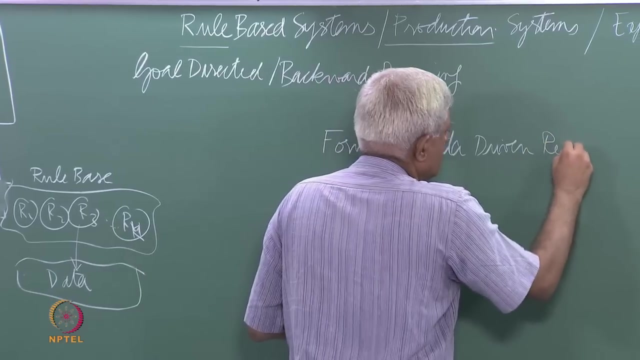 And there are people, a lot of people, who feel that human beings, by and large, are goal directed reasoners. they are backward reasoners they do not reason from. So this is goal directed versus forward, or you might say data driven reasoning. 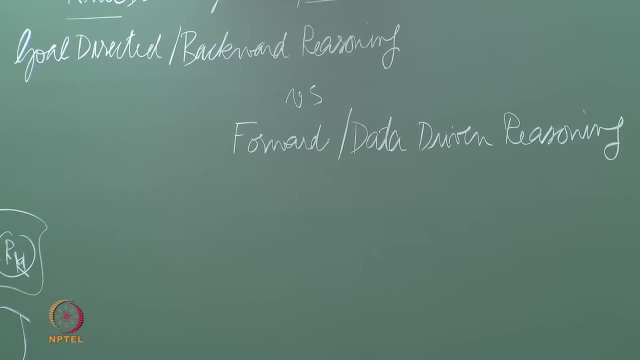 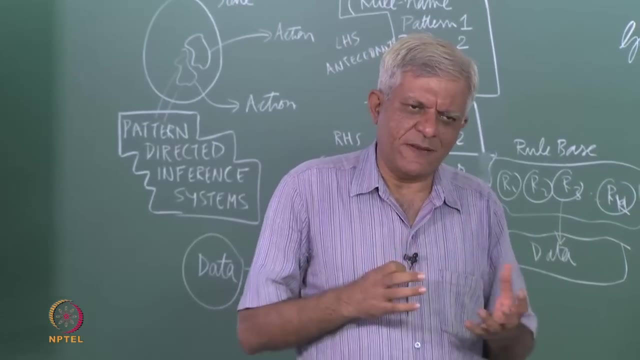 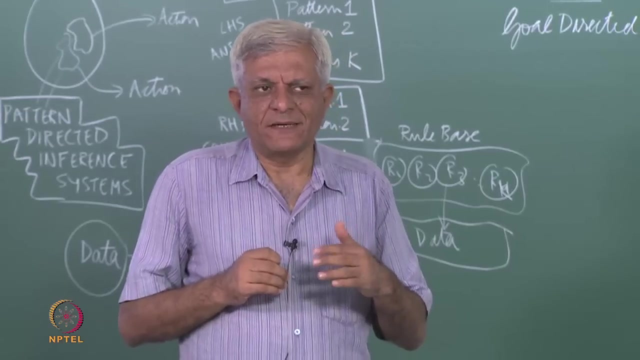 So data driven reasoning is some kind of an algorithm which looks at data and says that if I see this pattern, I will do this action, and so on and so forth. So the decision of what to do next is driven by, is decided by the data that is available. 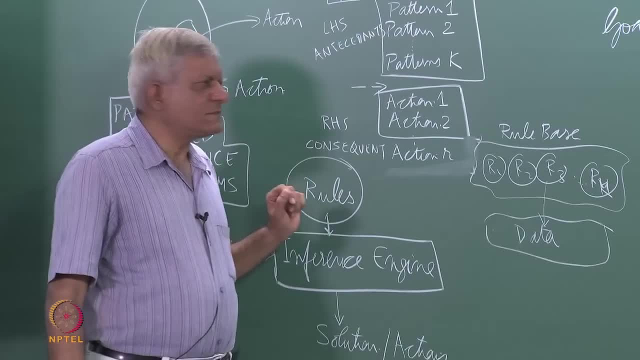 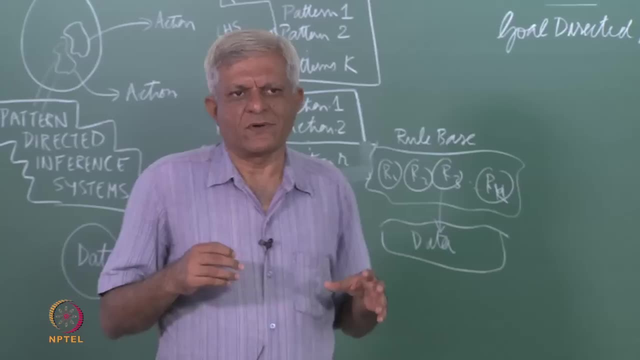 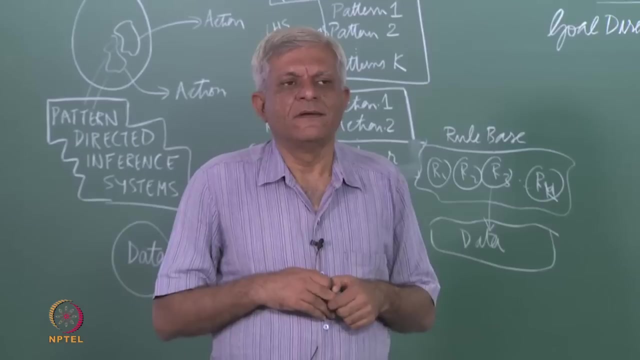 to you, which is the form that we will be looking at today. So goal directed reasoning says that if I have to achieve a certain goal, what sub goals should I achieve essentially? So, for example, you might say that if you want to get a scholarship into a good US university, 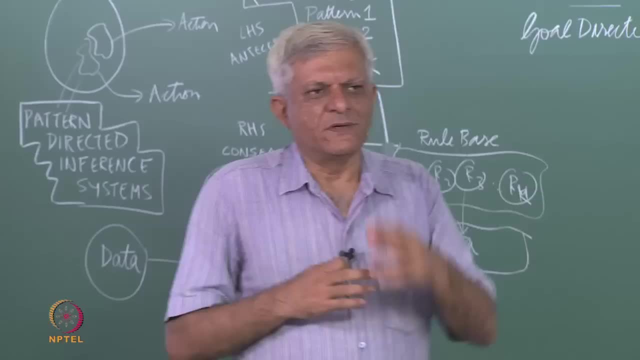 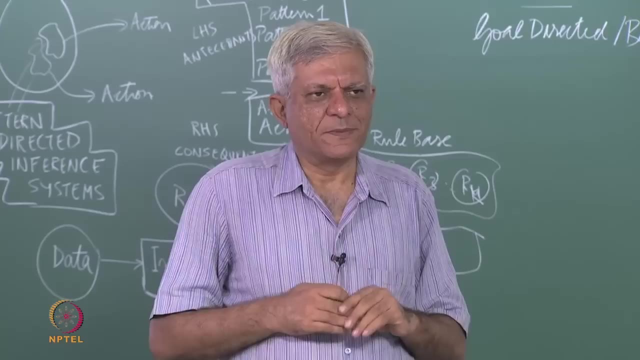 for doing post graduate studies. then what do you need to do? You need to write GRE, you need to do well, you need to get recommendation letters, you have to write an excellent statement of purpose and all this kind of sub-definitions. 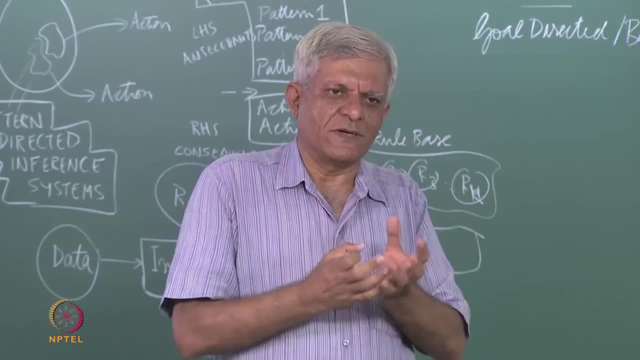 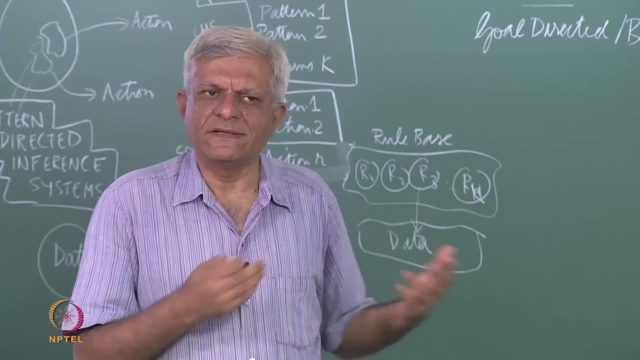 These are sub-goals, and to do that, to get good grades, what do you have to do? You have to attend classes and study hard and write exams well, and so on. So if you go from goal towards sub-goals and essentially, eventually, towards actions, 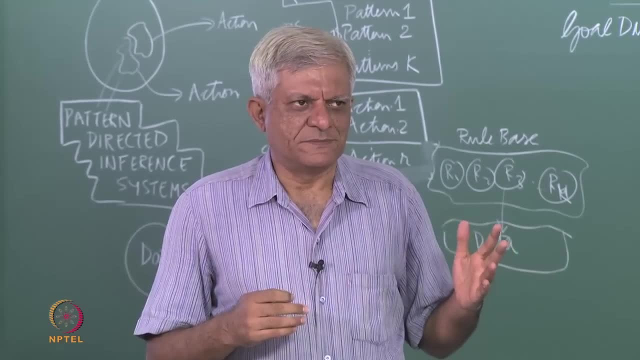 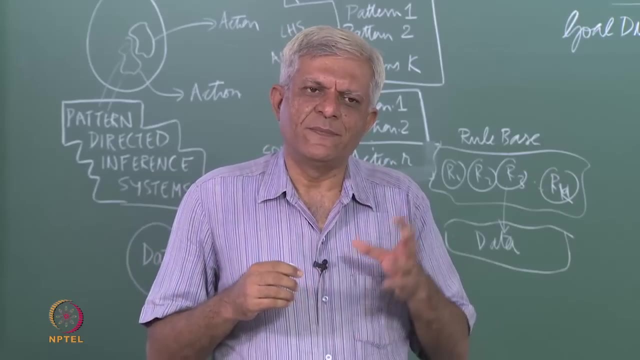 then you can decide what are the actions that you need to do. essentially. Again, let us say that if I have to plan a trip from here to Monday, then in goal directed reasoning, I would say that first may be I need to go to Delhi and then from Delhi. 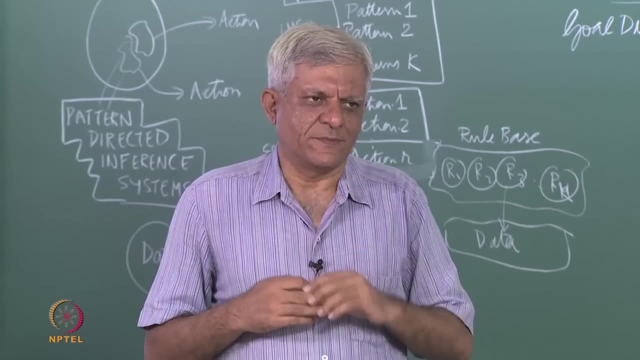 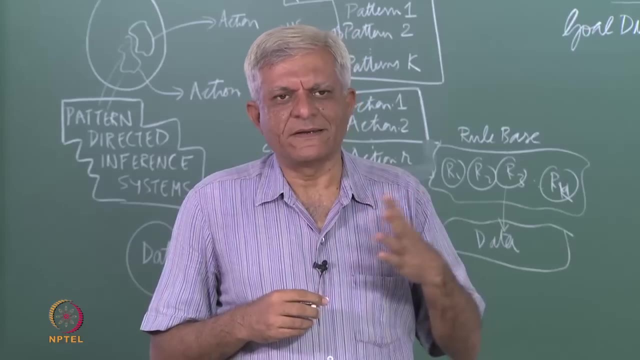 I need to fly to Chandigarh Or take a train to Chandigarh and then take a bus or a car or something, and then work out the details later. essentially, How do I go from here to the airport? How do I book my ticket? 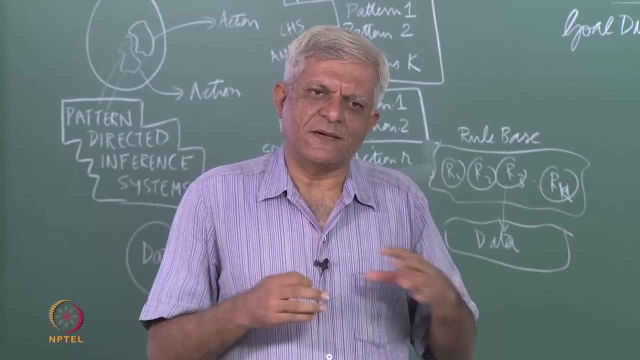 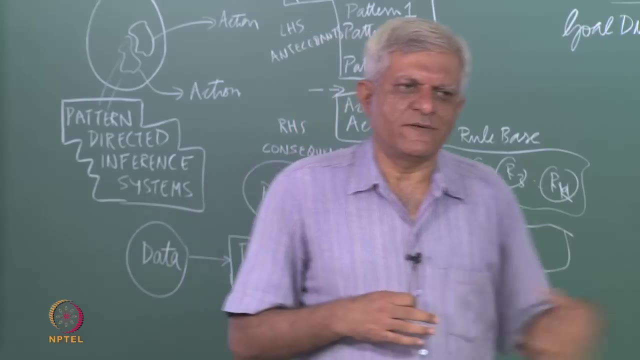 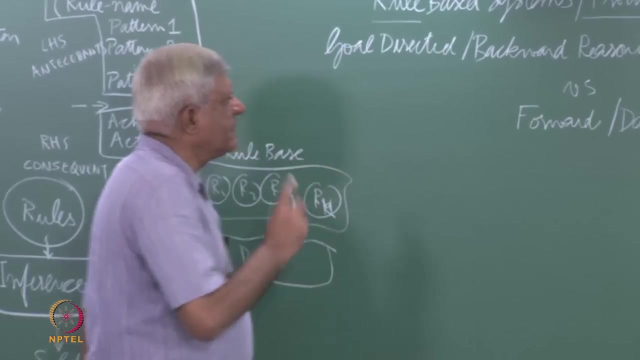 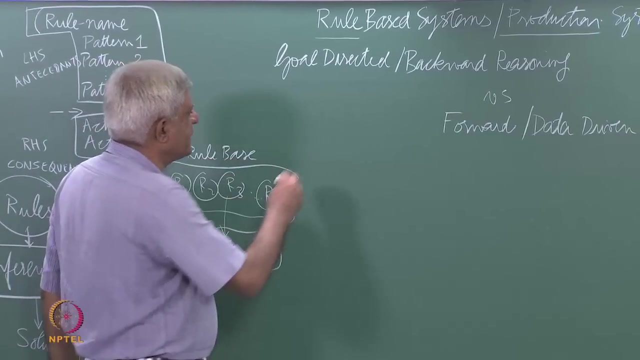 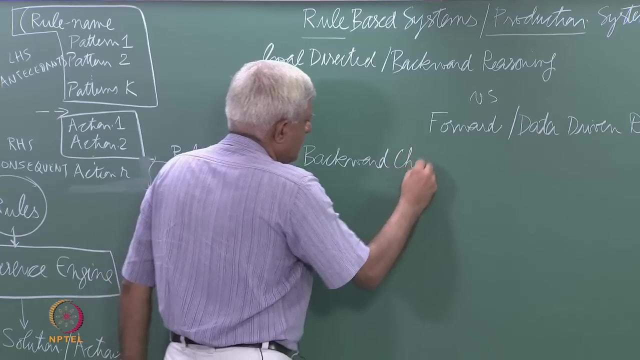 And how do I go from? the lower details come later. In goal directed reasoning you reason from the high level goals to the low level goals and at the lowest level you have actions. essentially, Now there is a corresponding Implementational comparison that you can make. it is called backward chaining versus forward. 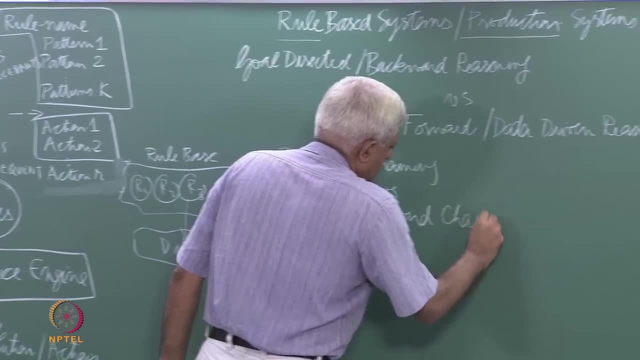 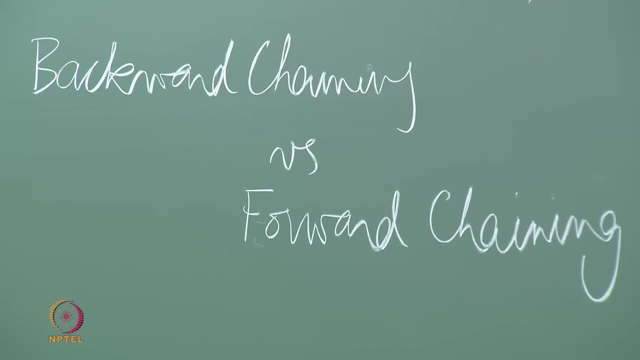 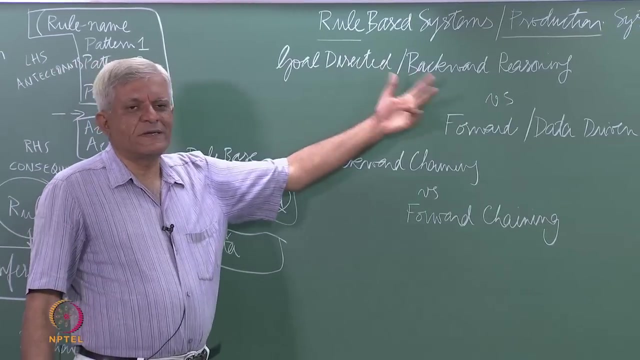 chaining. So by backward chaining and forward chaining, we essentially are talking about how to do it, For example, how the programs are implemented, whereas the backward reasoning and forward reasoning we are talking about what is the kind of reasoning you are? 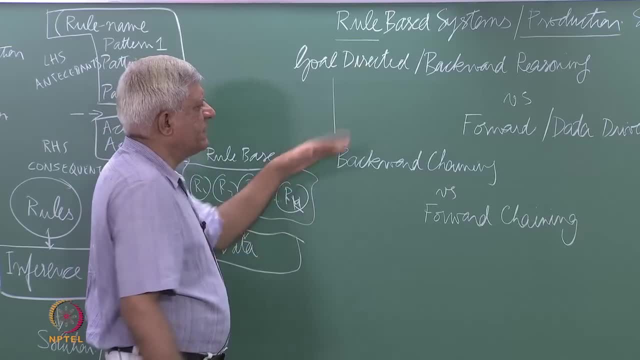 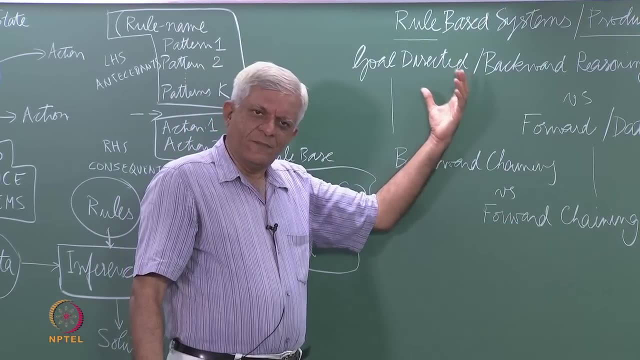 doing So by and large. of course, backward chaining goes well with backward reasoning and forward chaining goes well with forward reasoning. but it is possible to do forward chaining and implement backward reasoning, or it is also possible to implement backward chaining and implement forward reasoning essentially. 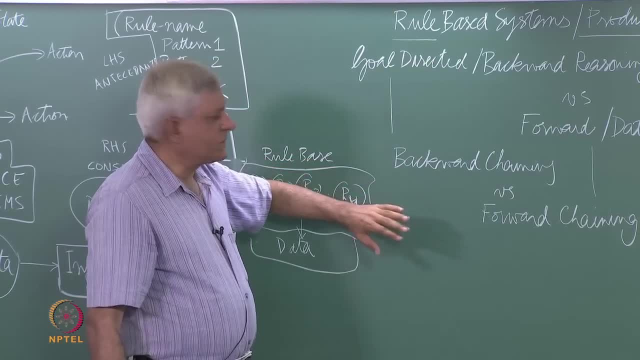 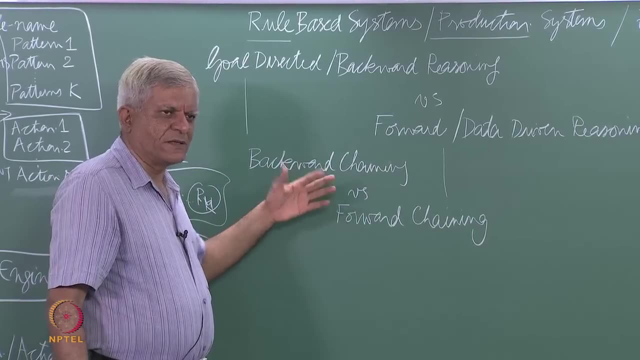 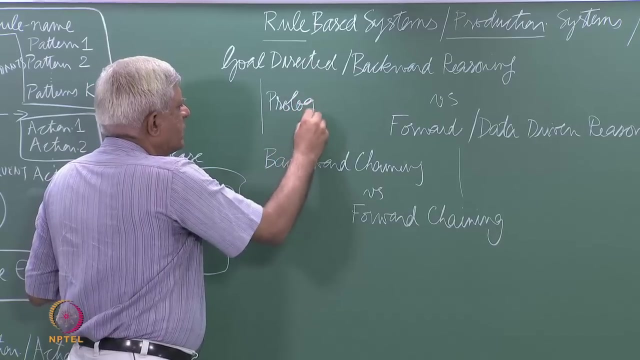 reasoning and backward chaining. sorry, backward reasoning and forward chaining is something, or actually we should call it backward chaining. So this combination- for those of you who have written programs in prologue, you would recognize that in prologue you are doing essentially backward reasoning. and if you view 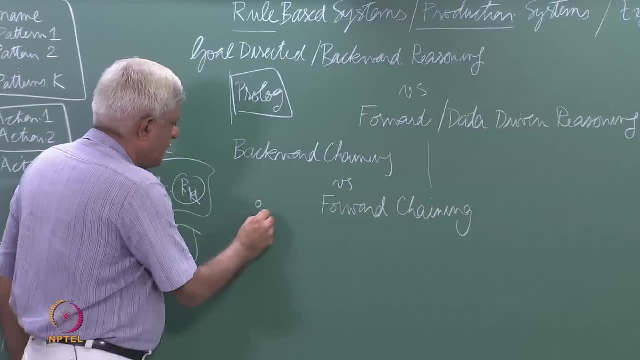 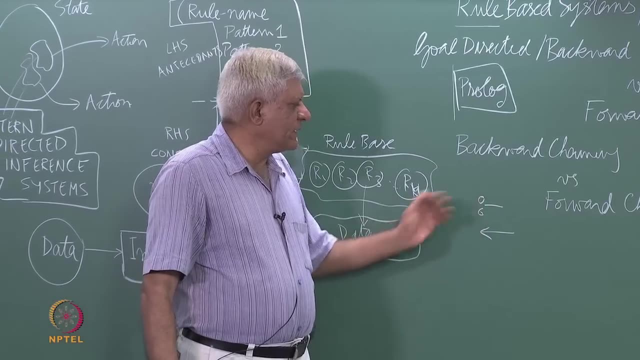 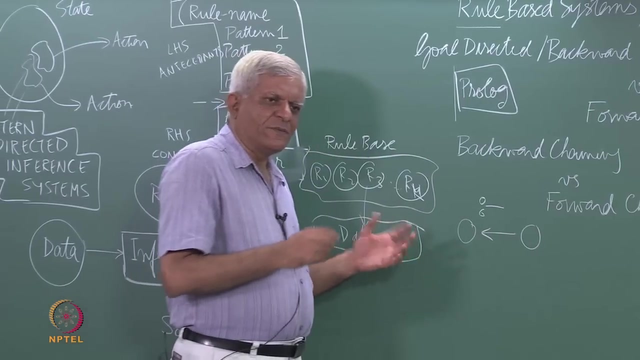 the sign. this sign in prologue as an backward pointing arrow, which we will do when we look at logic a little bit later in this course. we will look at this. then you can see that you are essentially chaining from this to this. So in backward chaining you are chaining from the right hand side to the left hand. 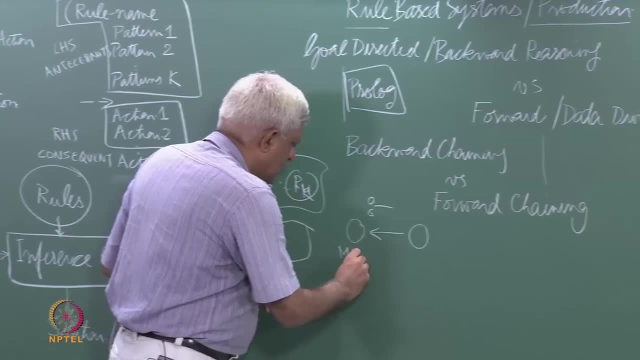 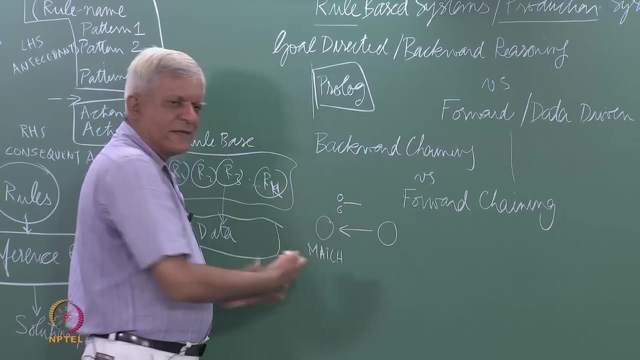 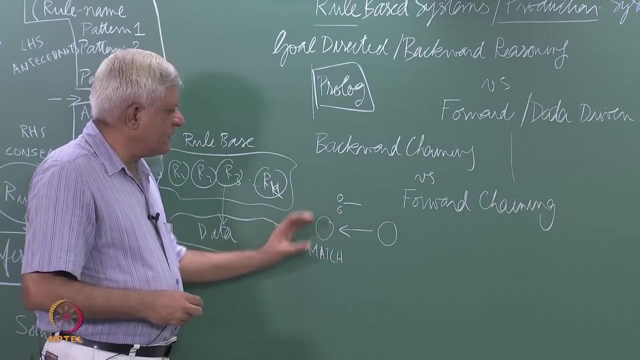 side, which means you match. So this is actually the right hand side. why? because the arrow is pointing this way. I could have drawn it like that, but in prologue you write the goal first and then you write the sub goals. if you remember prologue that, if you want. 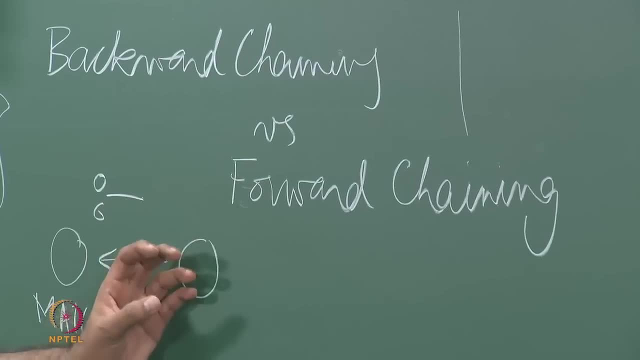 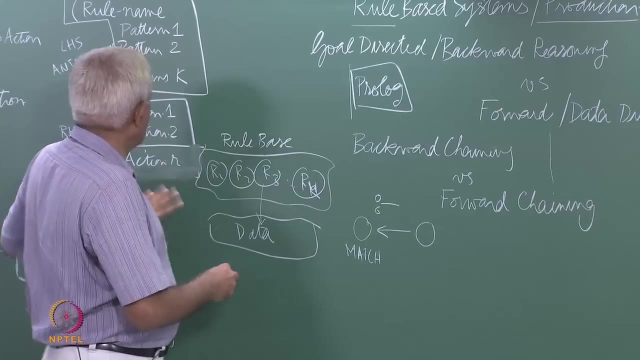 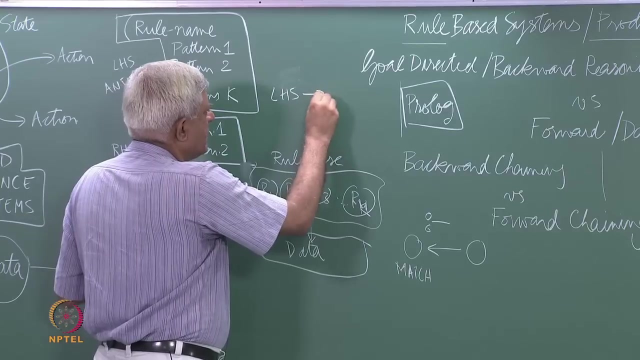 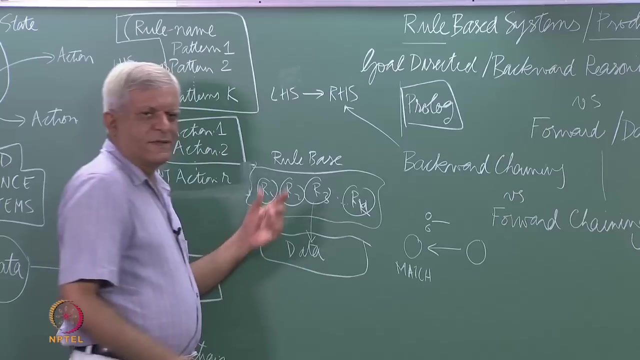 to sort and array, then you have to have a permutation of an array which should be sorted and so on and so forth. So it really depends on the match which side. So if you look at this rule- format LHS and RHS- then in backward chaining you are matching here with the RHS and 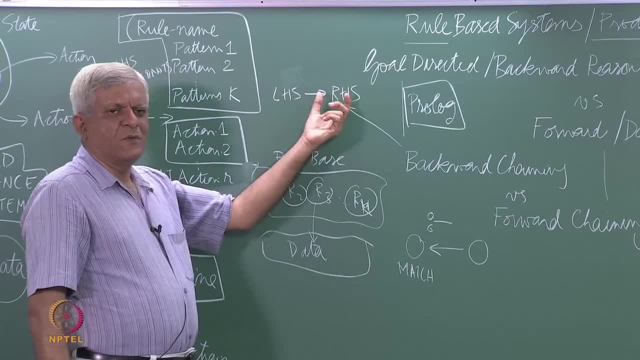 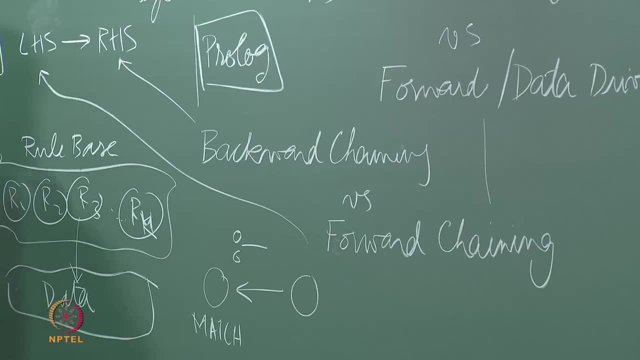 moving to the LHS. So you are asking that if this has to be true, then can I show that this is true? in forward chaining, I match the LHS and go to the right hand side. If I say this pattern, then I do this action. So we will be focusing today on forward. 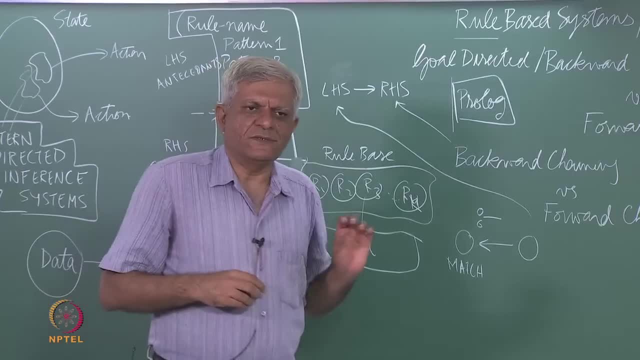 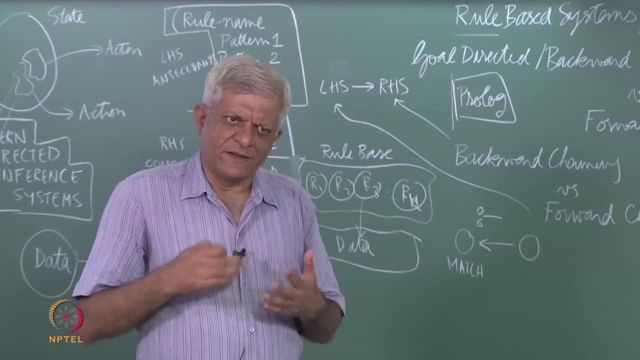 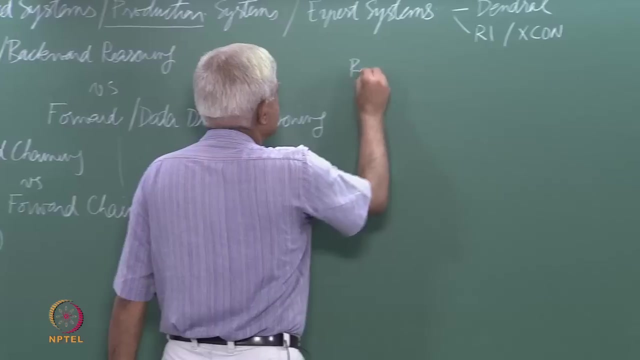 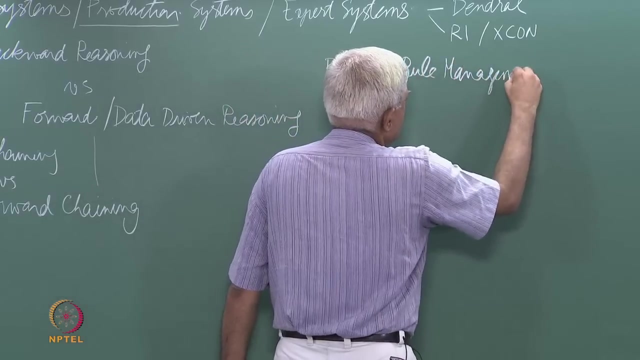 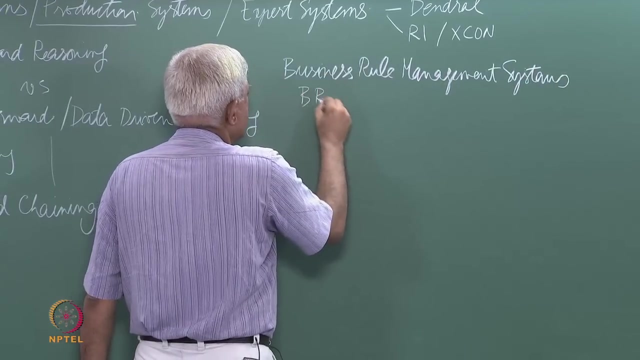 chaining mechanism Because it is very widely used technique in the industry. so I gave you coupling of example about banking and giving loans and so on and so forth. But there is renewable energy usage for ff management systems. So if you just look at this thing, BRMS, there is a whole community. 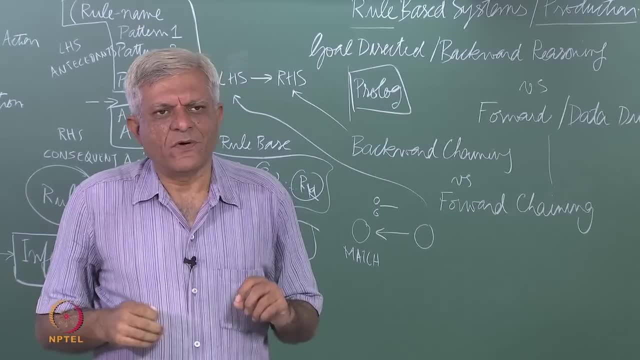 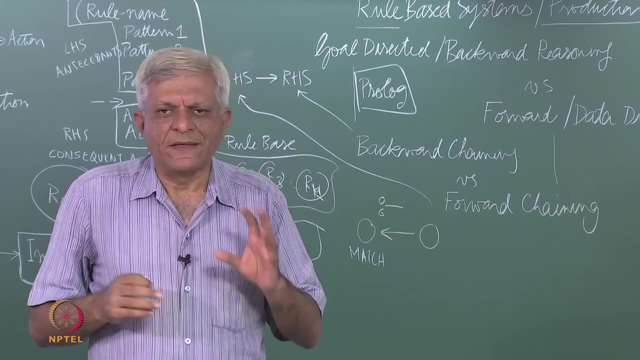 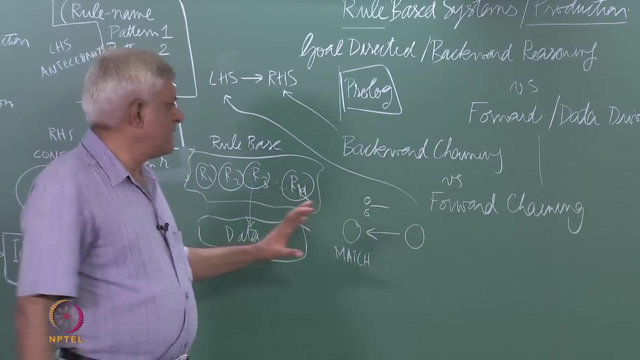 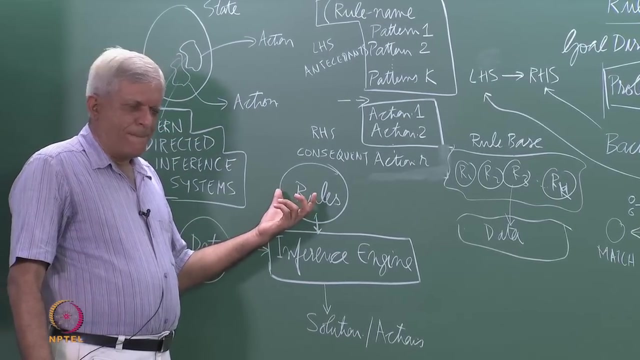 out there which is developing software for people in business, meaning it could be industry, manufacturing industry, banking business or anything- People who are domain experts to exploit computing power. the basic mechanism is this: that all you ask them to do is to write the rules and you implement the. 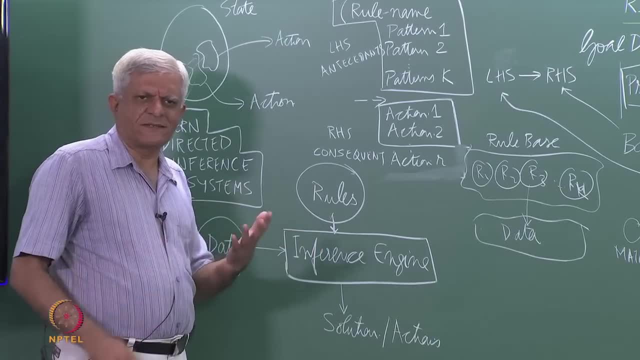 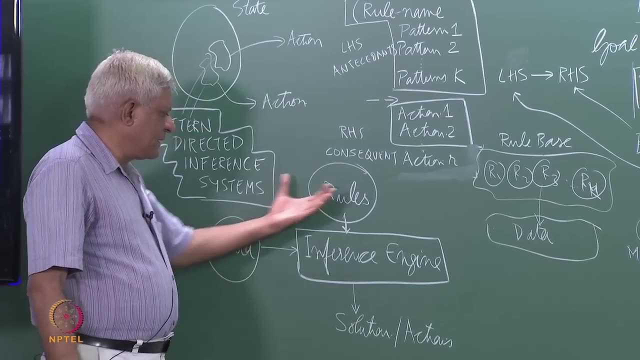 influence engine, which is a general purpose influence engine. You can say a search engine is a general purpose program. in a similar manner, an influence engine is a general purpose program which looks at their rules and their corresponding data and makes all the actions which are necessary to be done. essentially, 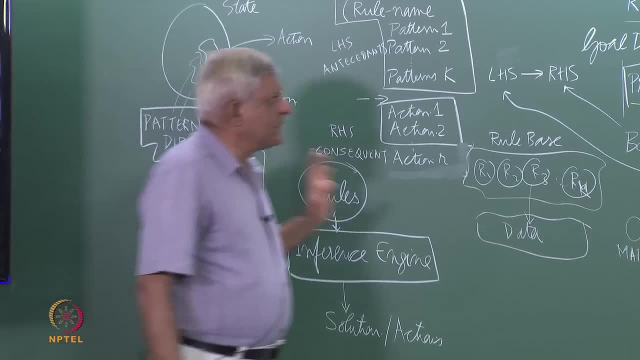 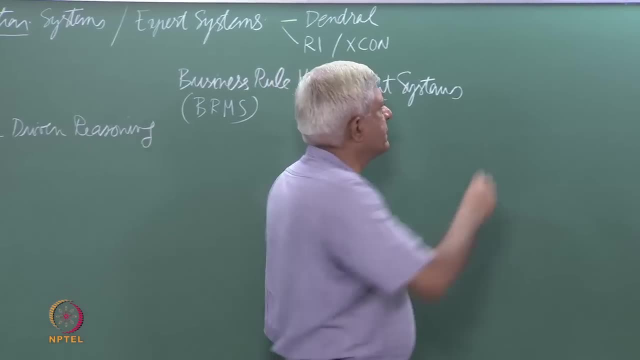 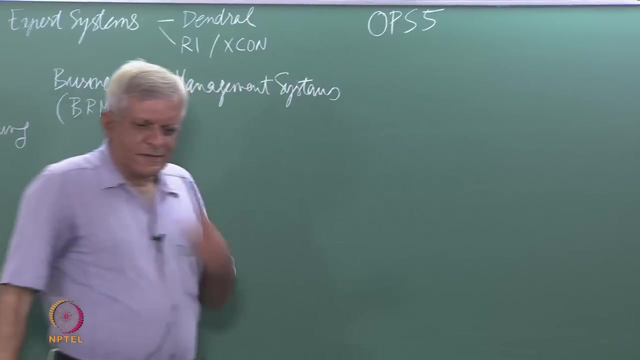 Now let us get down to some examples. So the language that I am using- we do not really have to use it in, I mean, you may not have to implement it- is called OPS 5.. This is the language is devised, which was devised I. 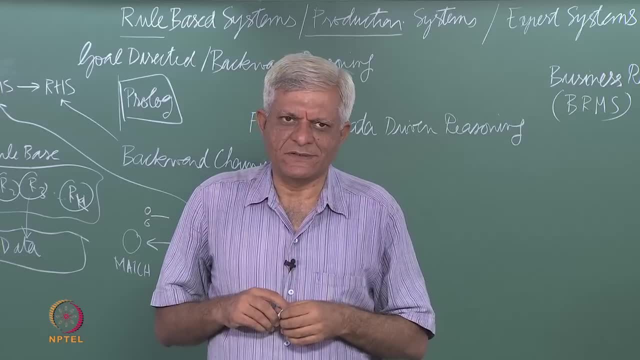 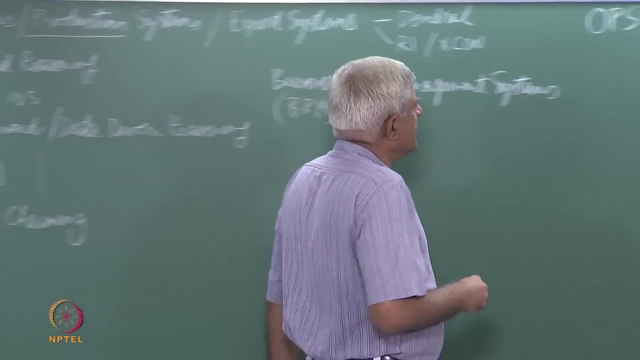 think in the 70s, also at Carnegie Mellon University, which is one of the centers where lot of AI related work was done in the middle of the last century. And some people say that O stands for official, So it is a official production system. 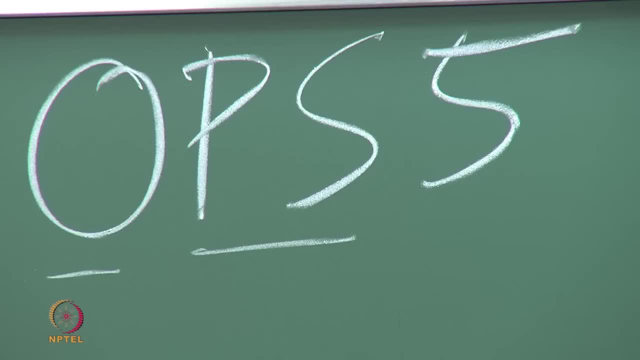 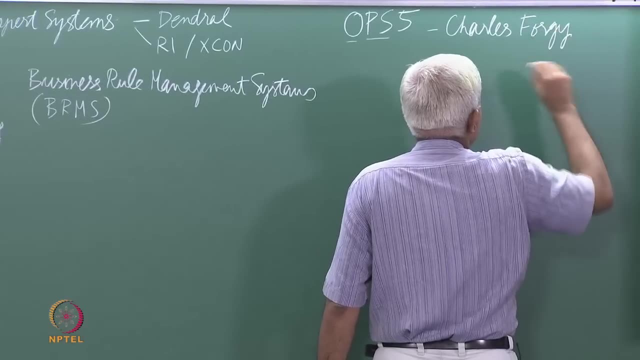 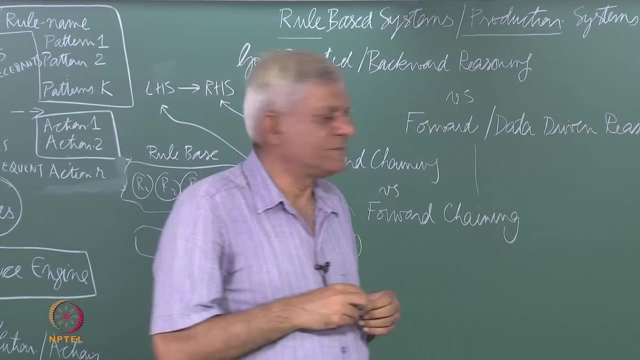 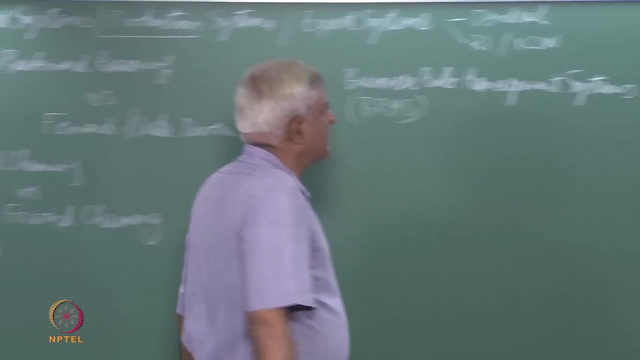 language, and its version was 5,, which became popular. It was developed by a guy called Charles Fourgy, who implemented this algorithm that we are going to look at for his PhD thesis, And then eventually, of course, it became something which was commercial in nature. 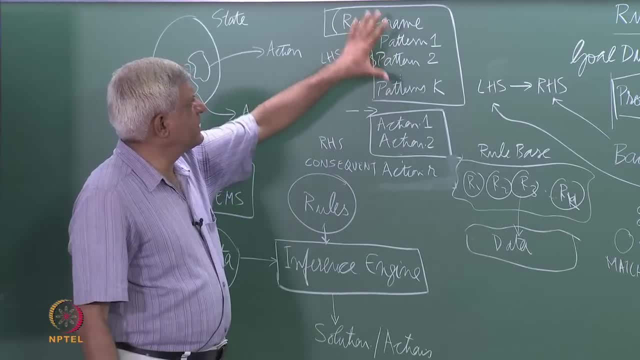 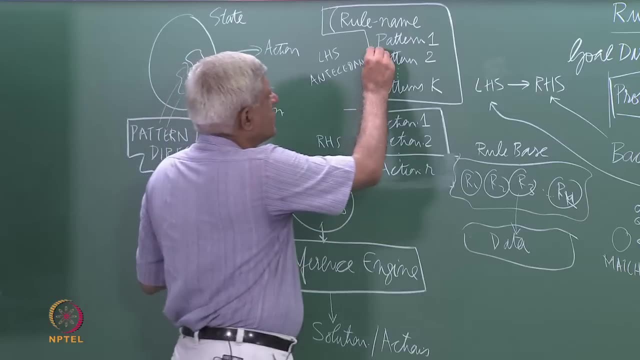 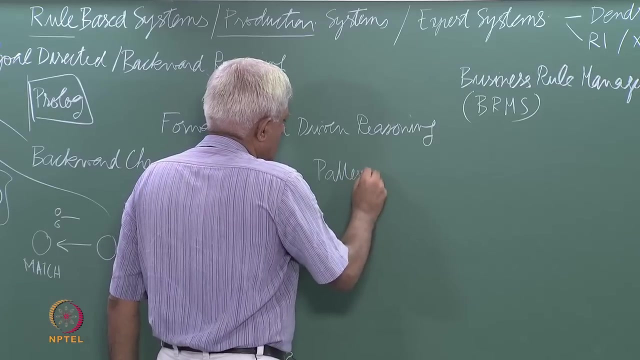 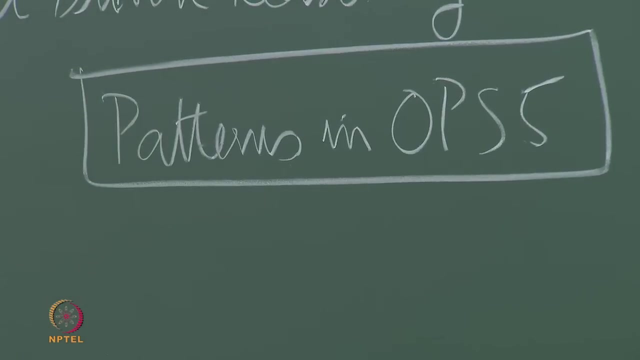 So, of course, what we need to do is to describe what is this language, what is the syntax of this language, and so I will focus, we will first focus on the patterns. So how do patterns describe in so they follow the something like a, like a objective? 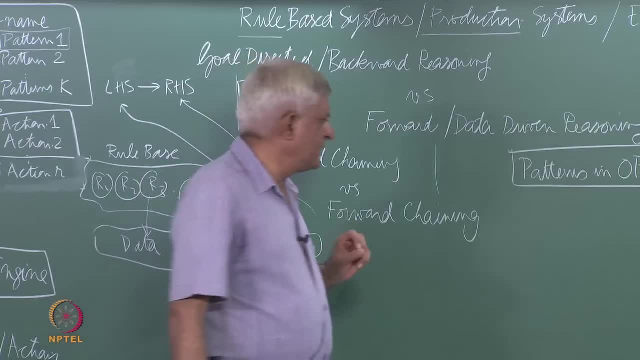 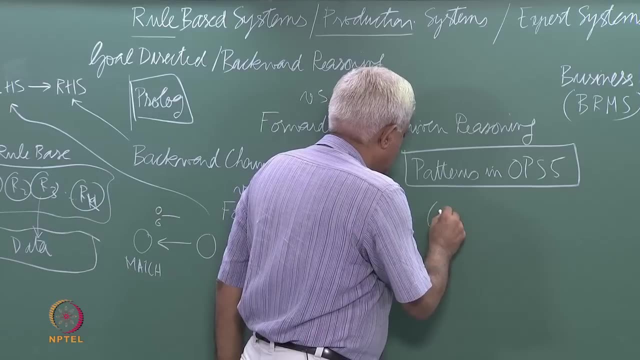 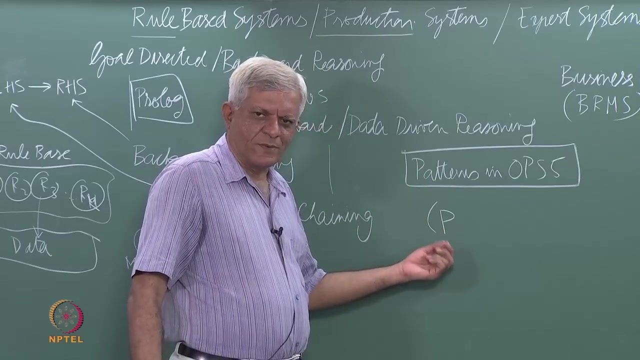 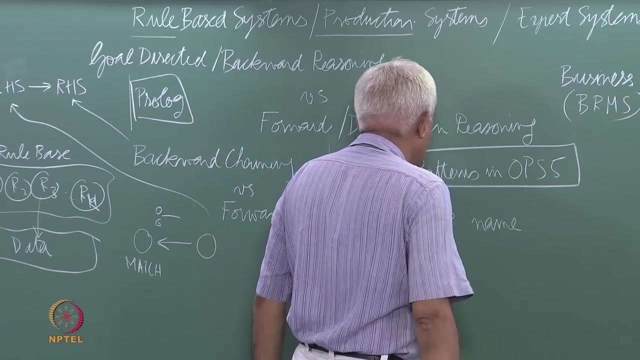 oriented way of representing things which are like classes. So one of the things that this language uses is that it uses p to stand for production, then name also. sorry, that is a language of a rule, so we will come to a rule a bit. 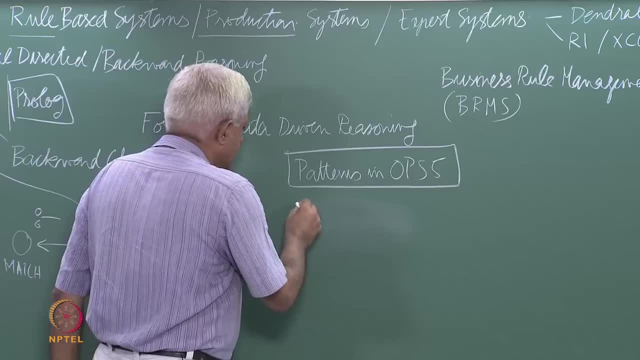 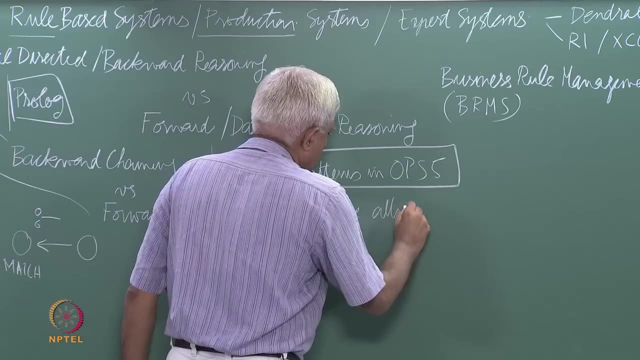 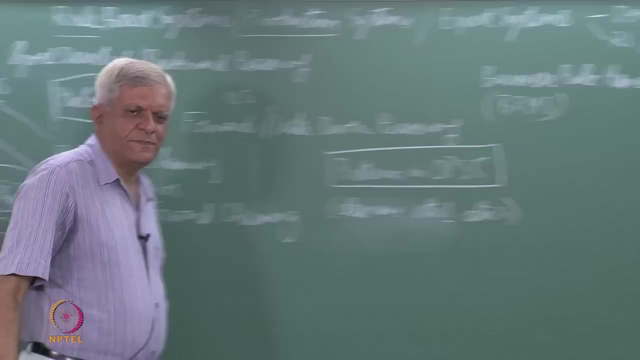 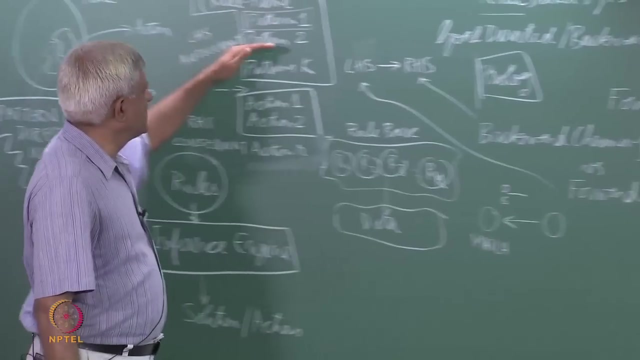 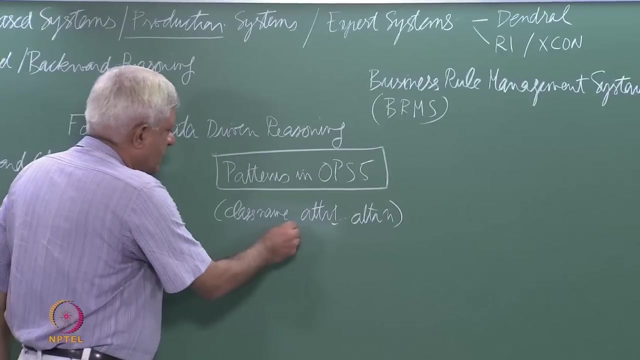 later. First, we want to talk about patterns. so there is a class name followed by attribute names, So very much like the class name. you know, remember that patterns are these things which are the which constitute the left hand side of the rule, and each pattern is made up of a class name followed by a set of attribute. 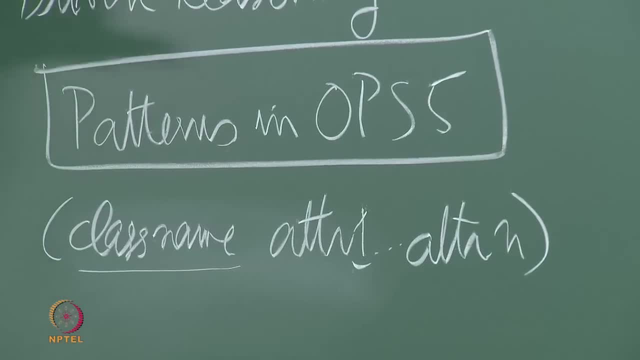 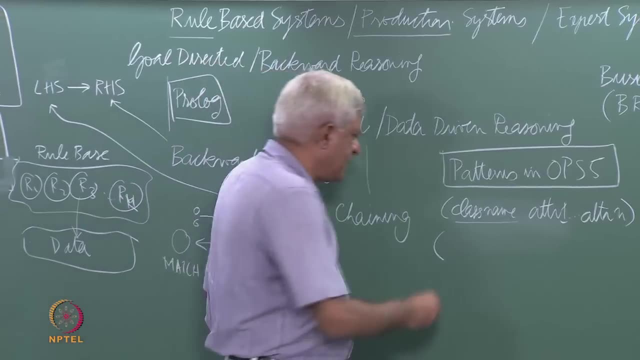 names. So this is the data structure that we are using in this language OF file. So, for example, if I am implementing a program, want to play cards, I might have a class name called card, then I might have the name of. 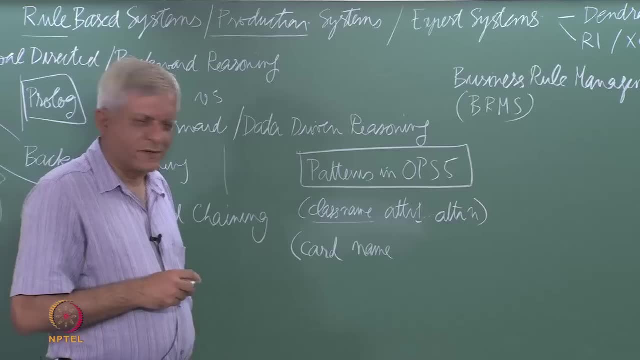 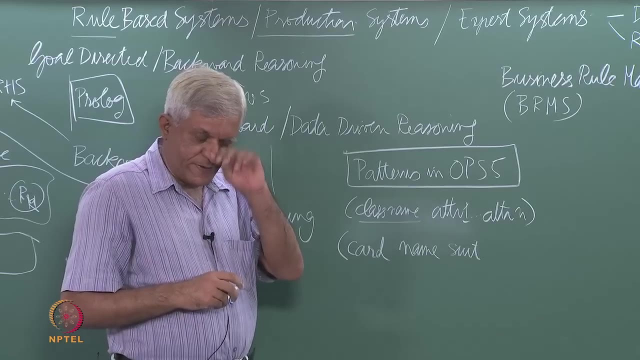 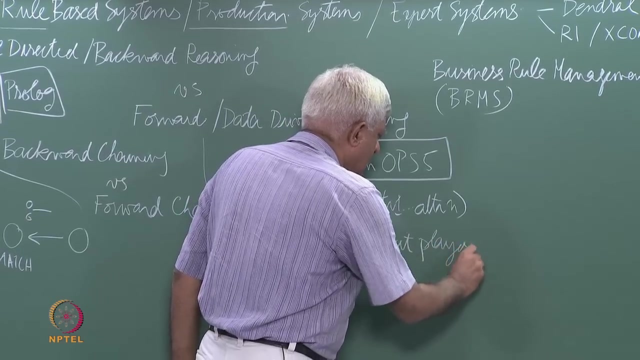 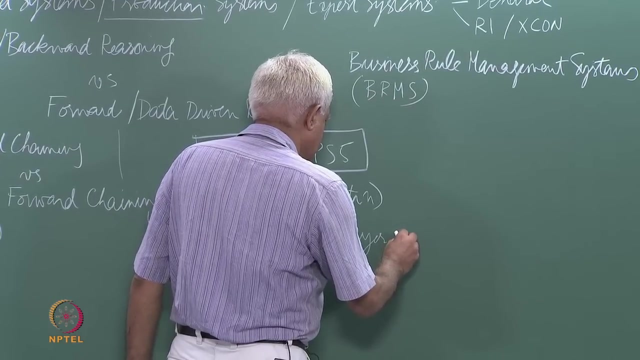 a card, for example ace or queen or ten, the suit of a card. So for those of you are familiar with cards, so spades and diamonds and clubs and so on- I might have the name of a player who is holding that card and 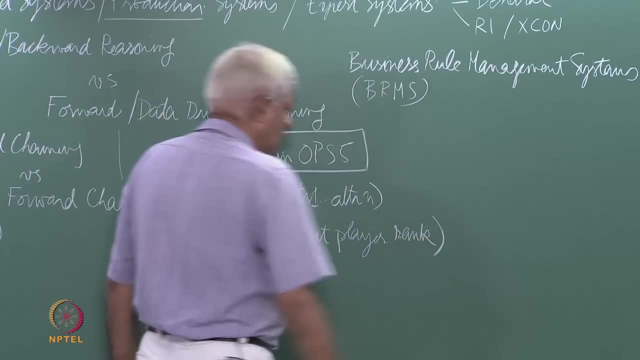 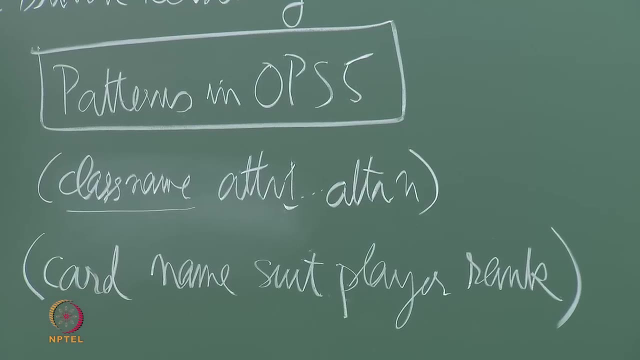 I might have rank of the card. So by rank I mean the current rank. So in most games, for example, ace is rank 1 and king is rank 2 and so on. but as the game progresses these ranks might change. 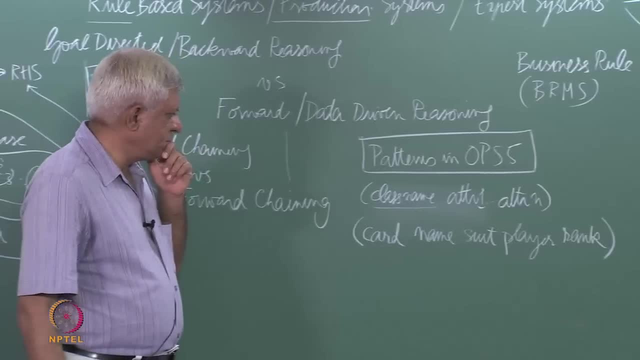 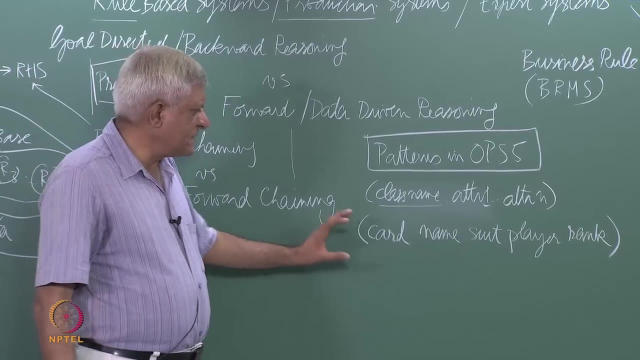 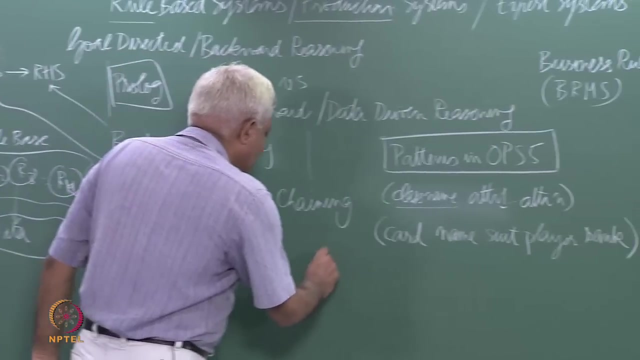 So I might want to store that essentially. So this is a class description and corresponding to this class description, I may have several patterns. So the patterns are the left hand side of the rule and a rule is signified by this opening bracket. 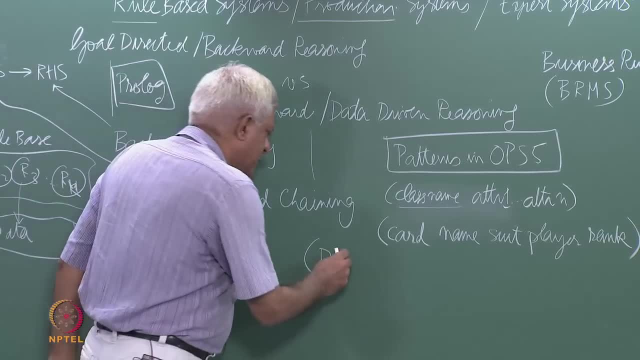 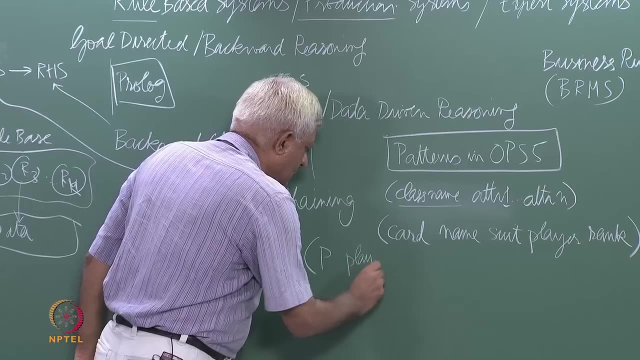 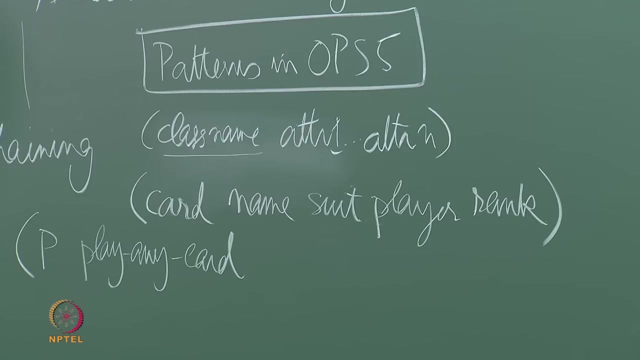 followed by p, which stands for production, and then the production name. For example, a play any card, let us say. I just want to write a rule which says: a play any card that you have essentially, And in this rule I might have a pattern. 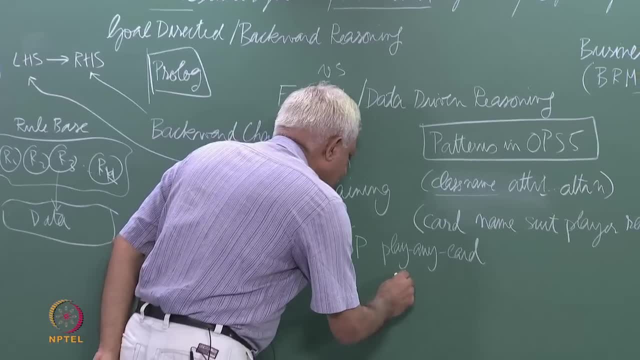 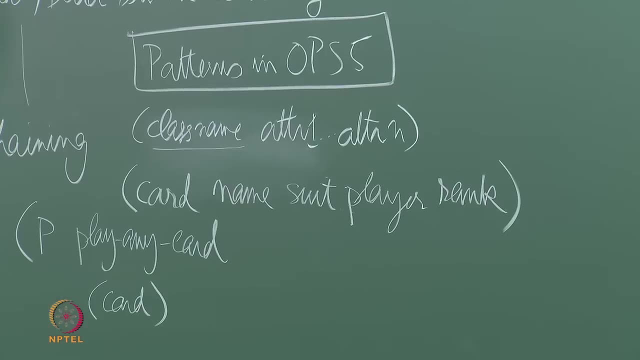 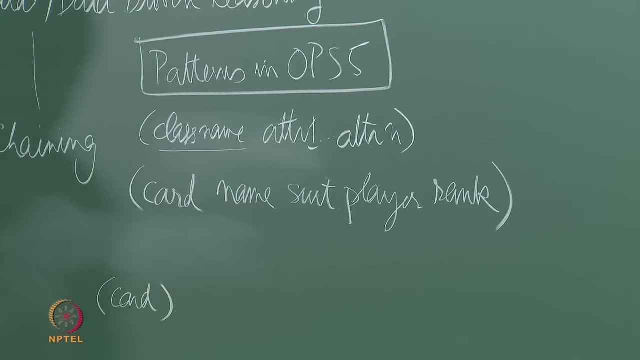 which says that you have a card- and I might just specify this, so let I come to this later. So let us just talk about the difference, different kinds, So for instance, here's kind of patterns that we can have, So we can. 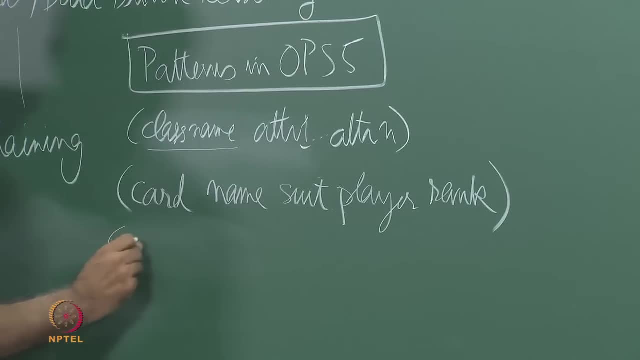 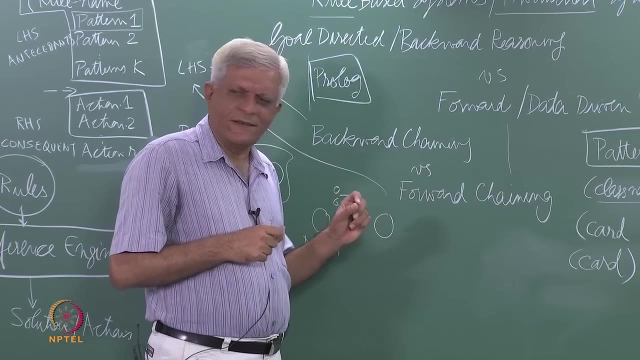 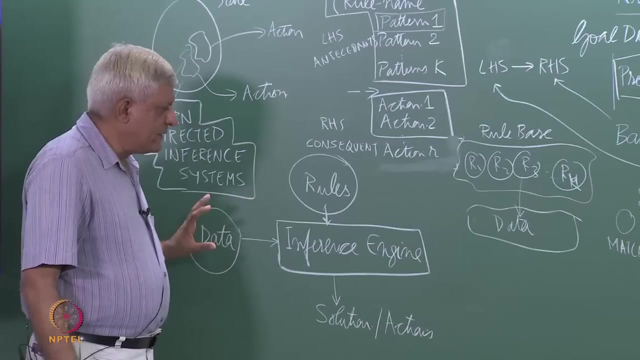 have just the name of the class as a pattern, which means that if the inference engine can see one data element in your data- So remember we have this data which has the class name card- then that will match that tool. Our task is to eventually going to be to match. 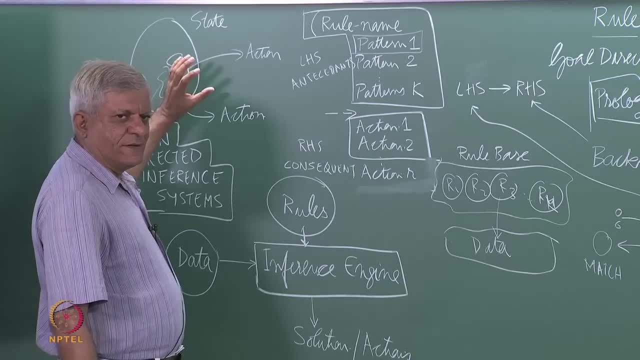 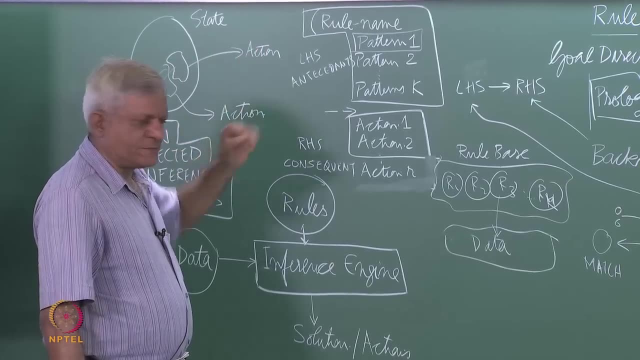 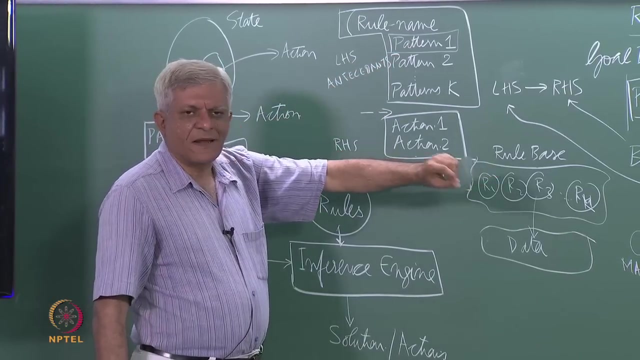 the pattern and see which patterns match. Of course there may be more than one rules which may be matching- we will come to that later- and then what action can be done? So for matching the rule, we have to match patterns and each pattern should match some. 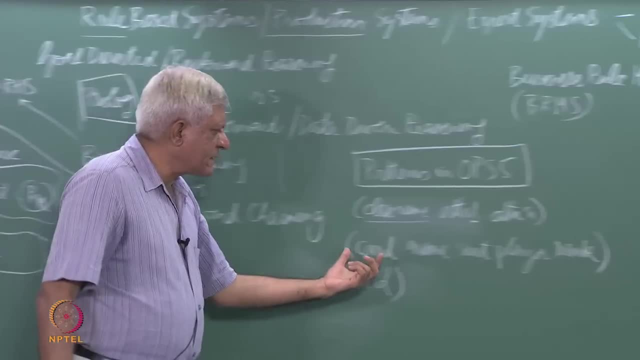 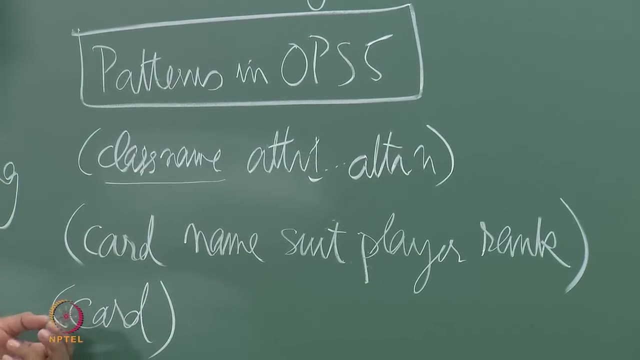 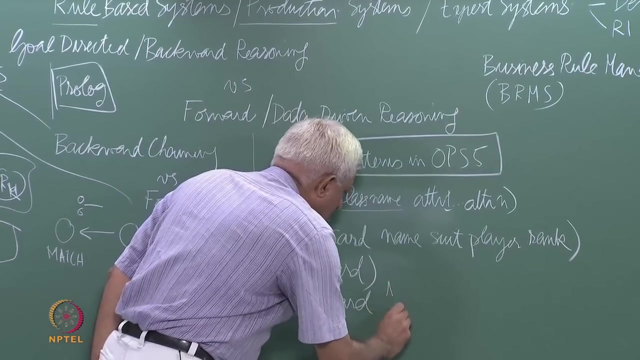 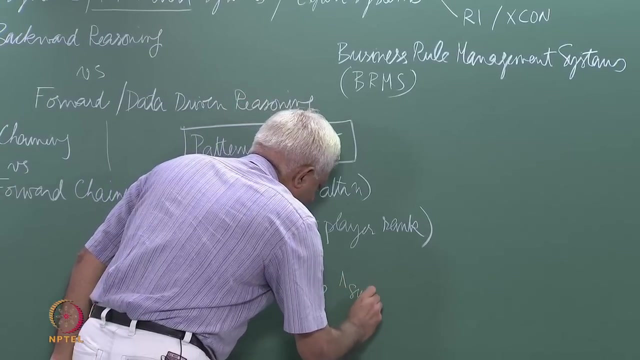 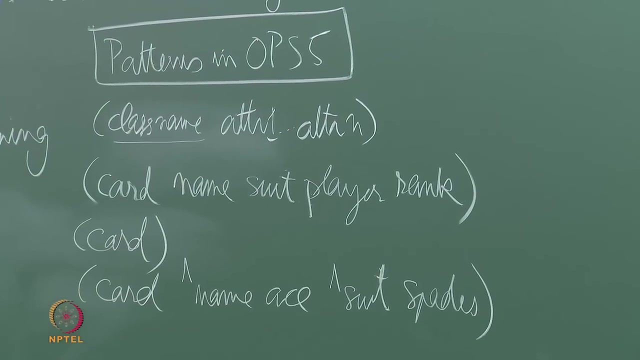 class description. So if my this class name is card and its attributes are name, suit, player and rank, then the pattern must be an instance of that, essentially, So I can have, for example, card name is suit space. So here I am saying that. so 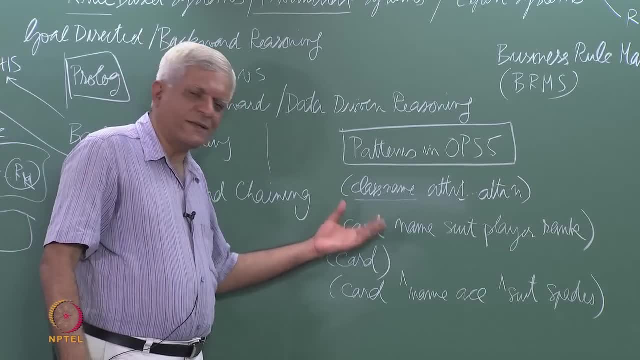 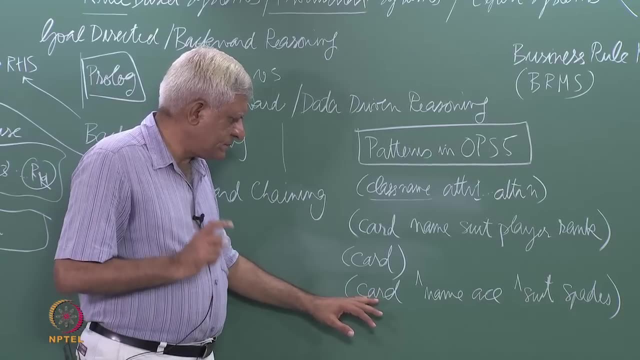 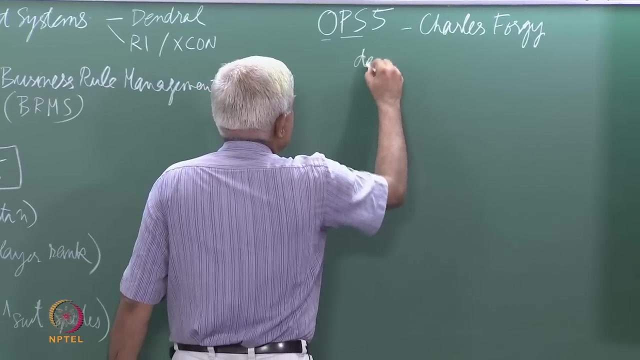 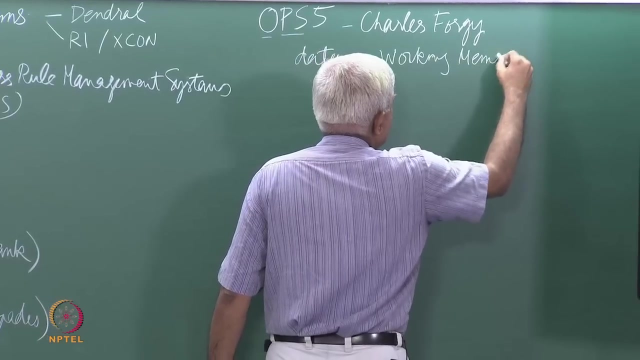 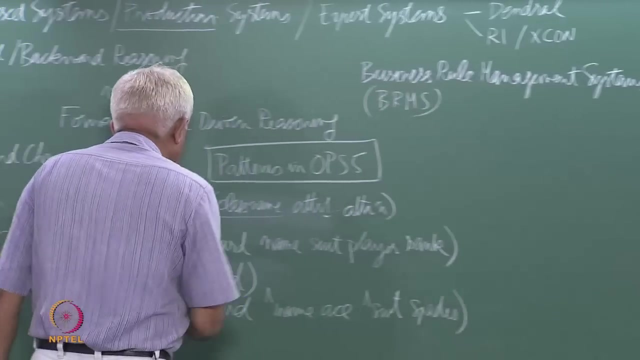 this is the way data is represented. this is the way the meta data is given as to, which describes the data. So data itself is written likewise this. So I have a element which obscure. data is in the working memory, which is called w, m, and each of this is called a working memory element. This is my Input system, where this data is taken by symbol fod and data is sent to the attacks list, isn't it? So this data itself is written like this. so I have an element which now pops five data there and alsoligt's data itself is written. 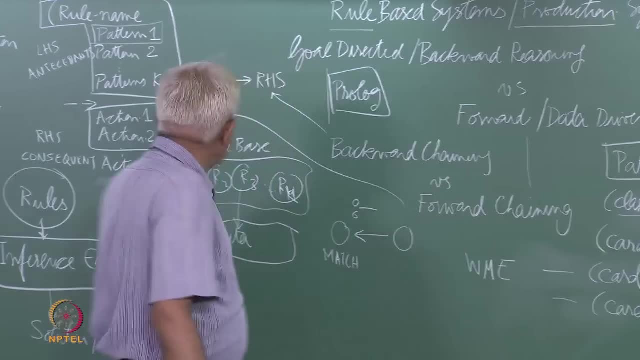 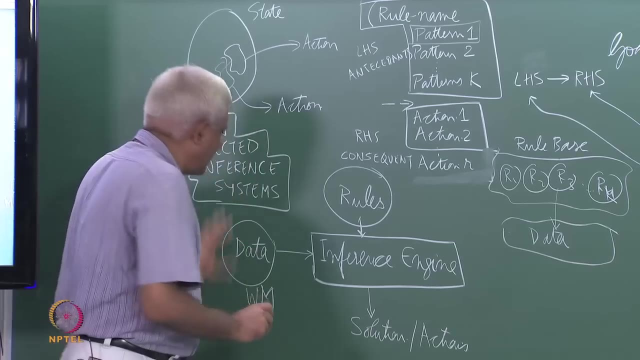 like that here. so I have a element. do I choose that I'll take this now, or how do I do this? So IT is in the working memory, which is called WM, and each of these is called Working. this is a terminology that they use. So this is a working memory and inside this of 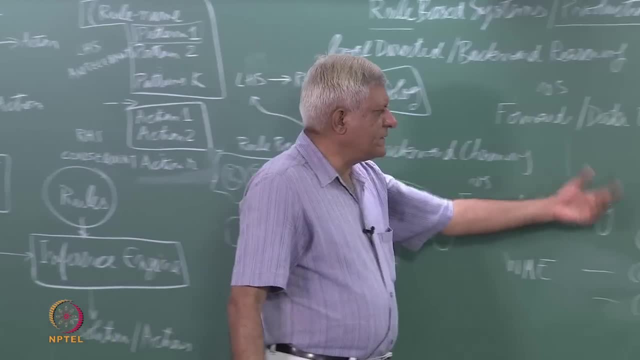 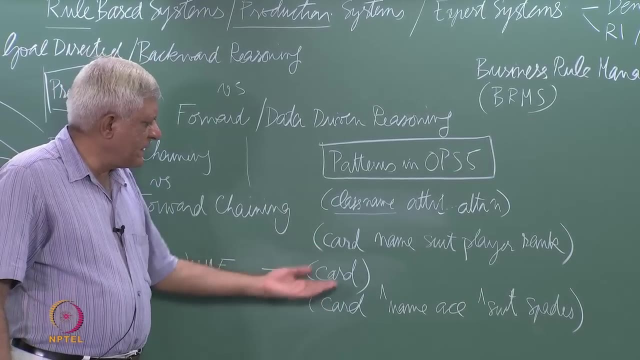 course there are these working memory elements where each element is an instance of some class name which may be not completely specified, which may be incompletely specified. So, for example, here I have only said that there is an element which belongs to the 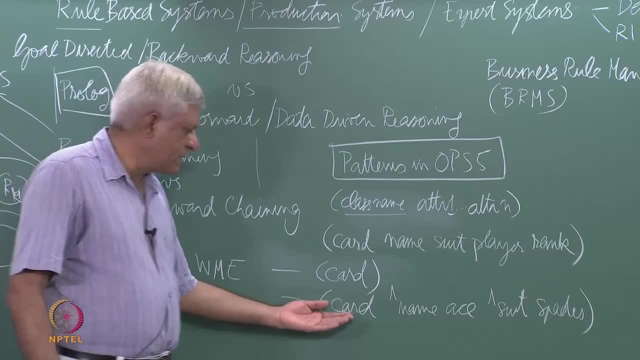 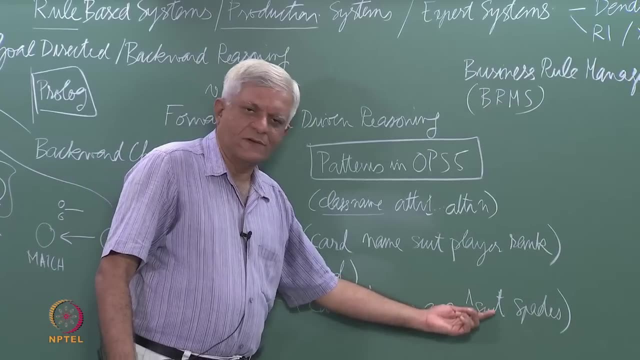 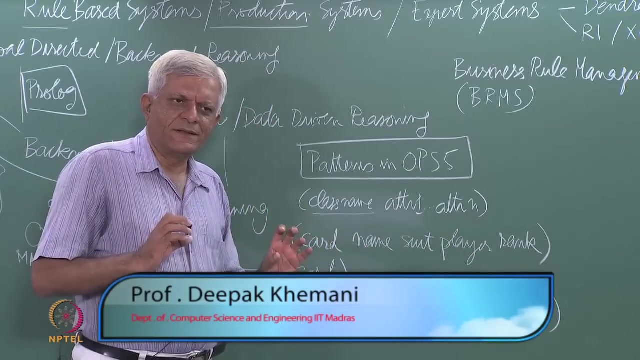 class name card. here I am saying there is an element which belongs to the class name card and the attribute name has value s and the attribute suit has value spades. essentially. Of course I can specify other things also, but any partial description can be there in. 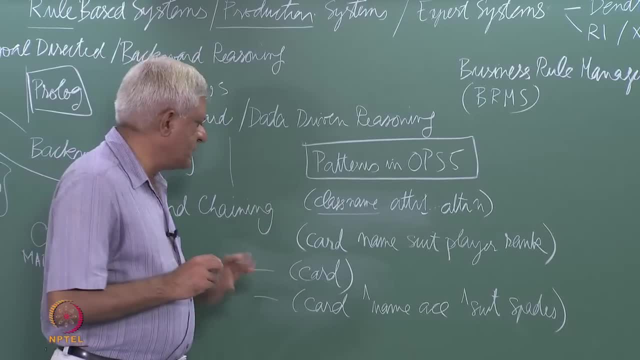 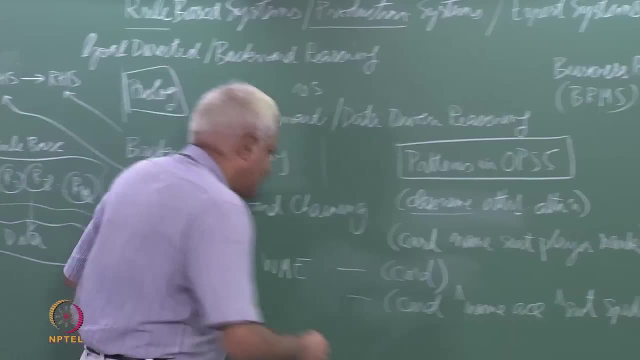 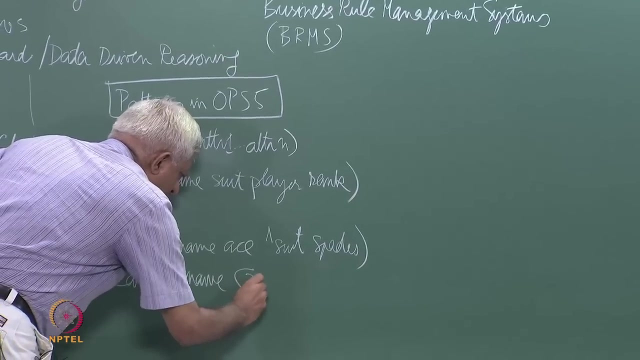 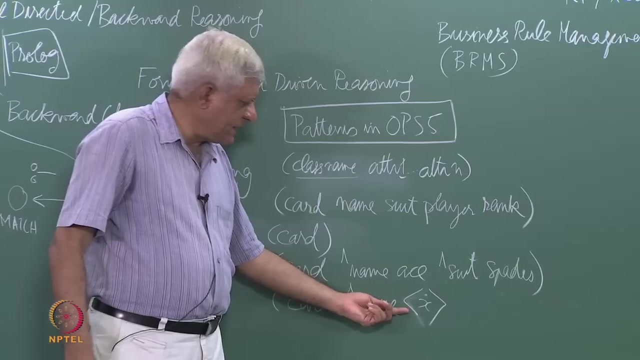 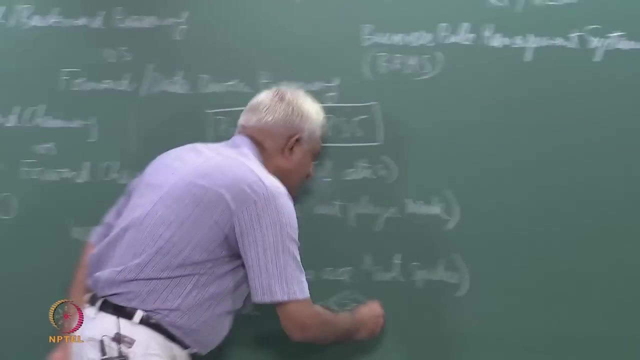 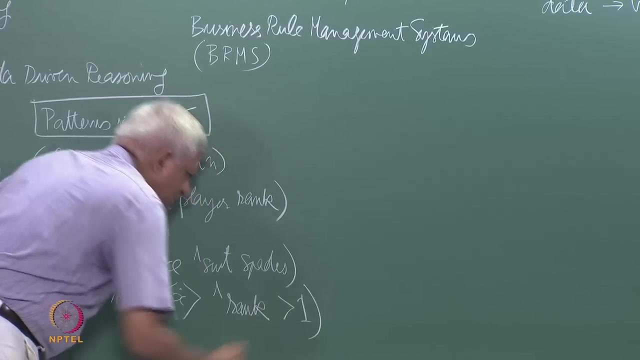 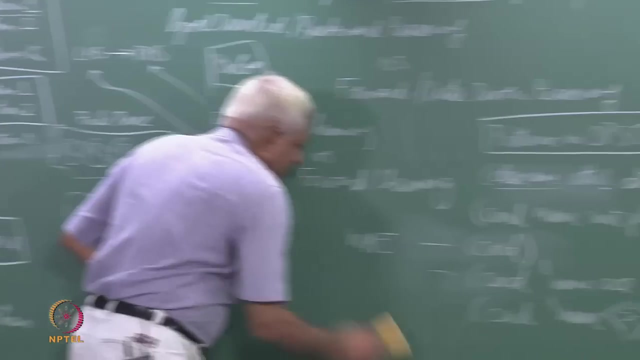 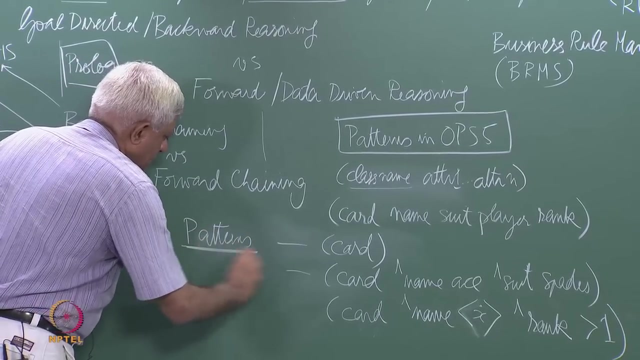 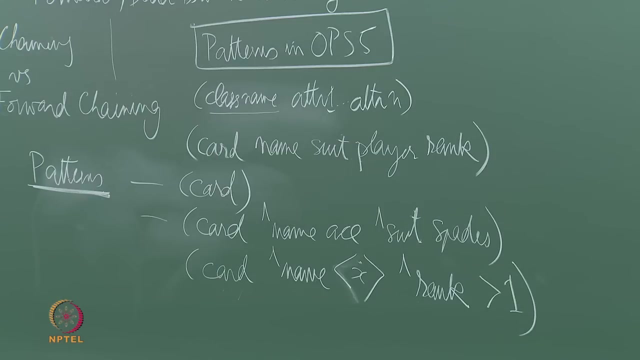 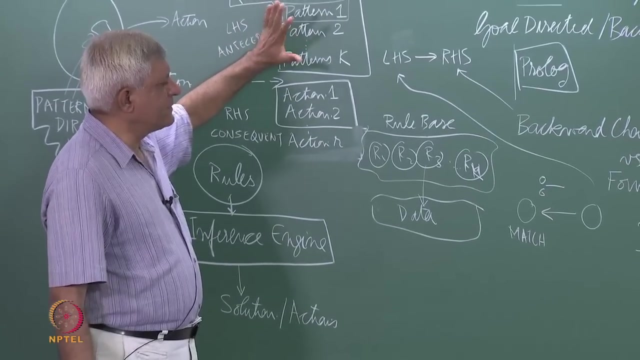 the pattern. we are talking about patterns in rules. essentially I can say things like card the patterns. So the left hand side of the rule is made up of a collection of such 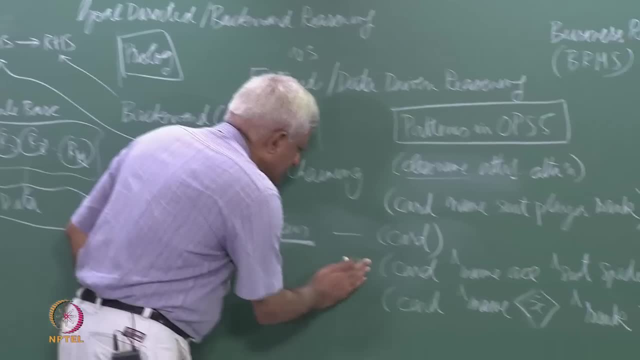 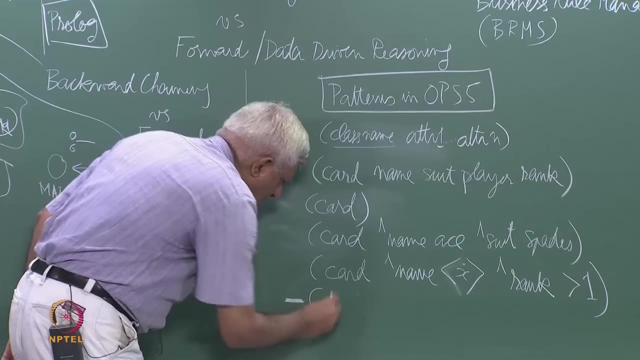 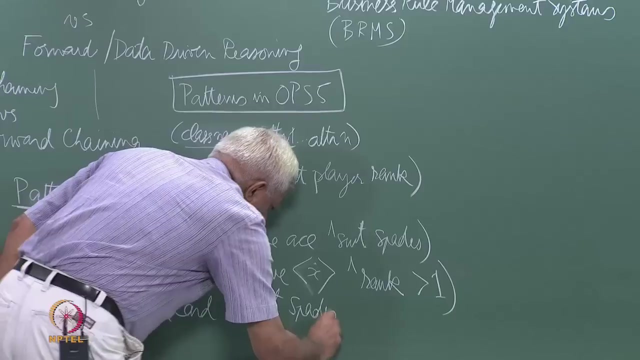 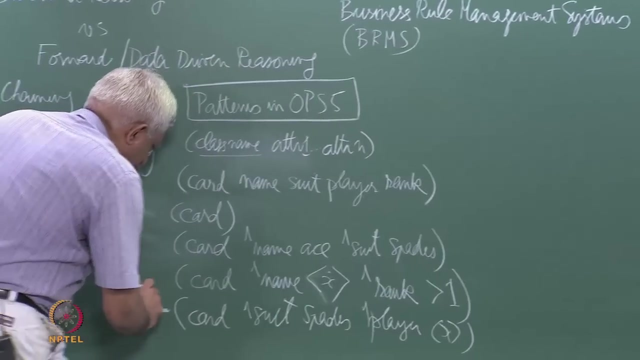 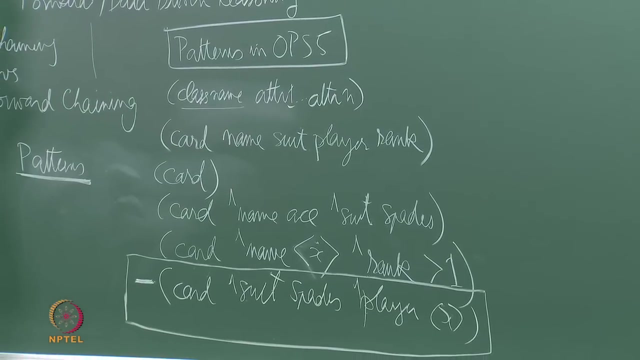 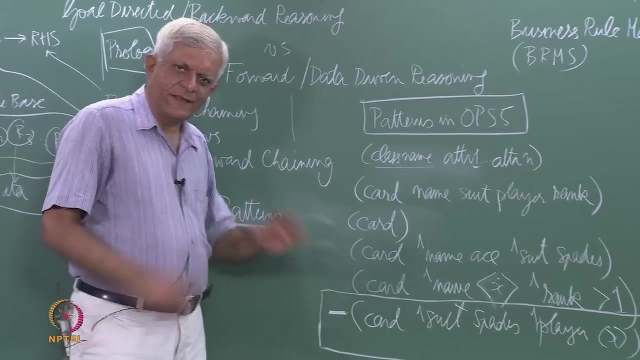 patterns. you can also have a pattern which is with a negative sign here, So this pattern is should be interpreted differently. it should be interpreted as saying that there is no such pattern in your working memory or there is no such data element in the working memory. 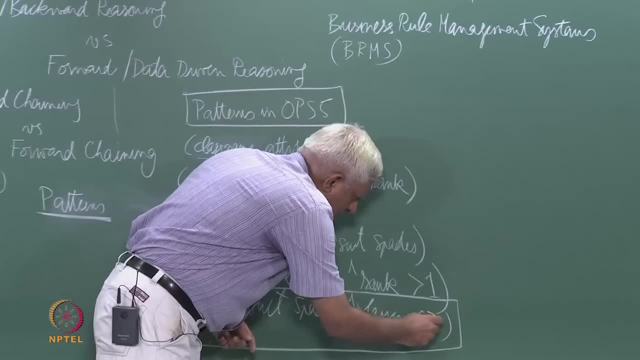 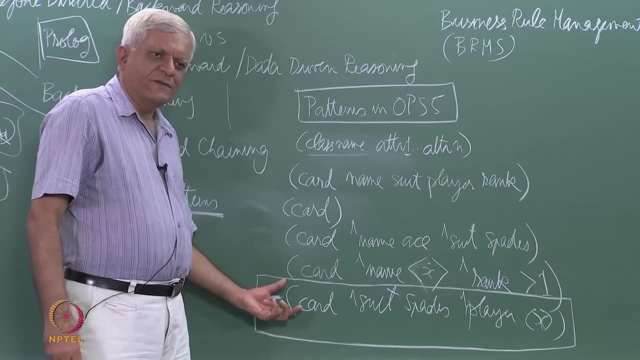 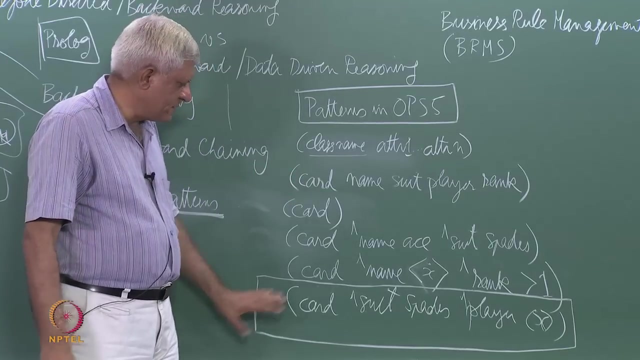 which says that player x- this is a variable x- has a card of spades. So such a pattern would be used to describe the fact that a given player does not have any spade cards in his or her hand. So this negation sign basically is the opposite of this. this says that this: 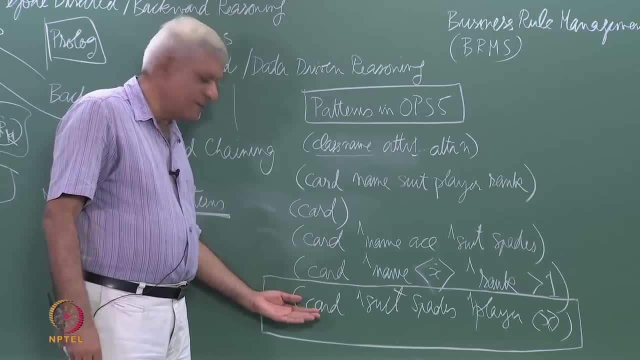 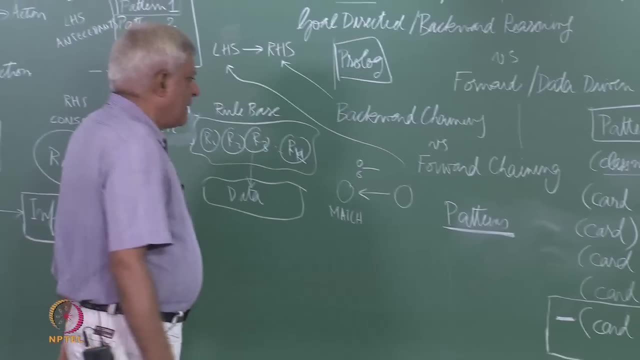 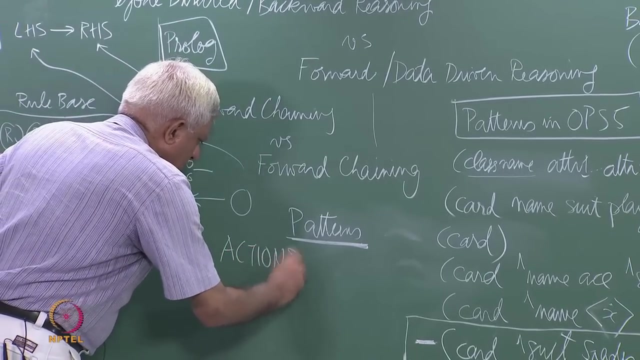 must be present in the database or in the working memory. this says that it must be absent in the database and only then this rule will match essentially. we look at some examples Now actions. so remember, we have patterns and we have actions. so the two most 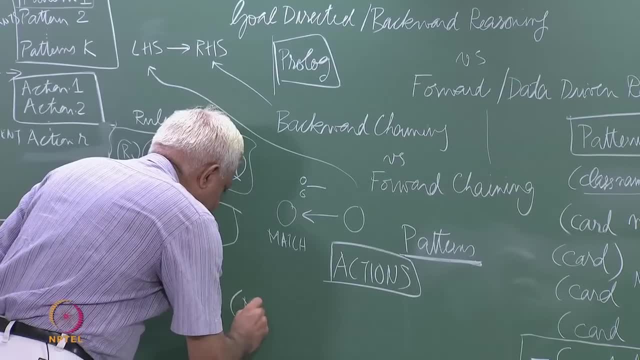 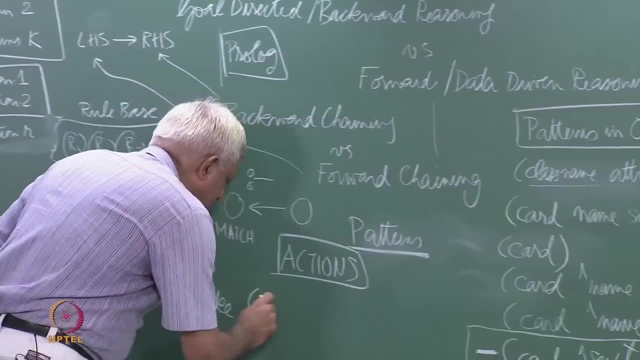 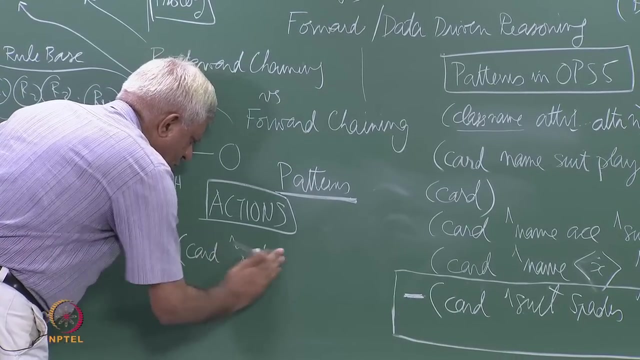 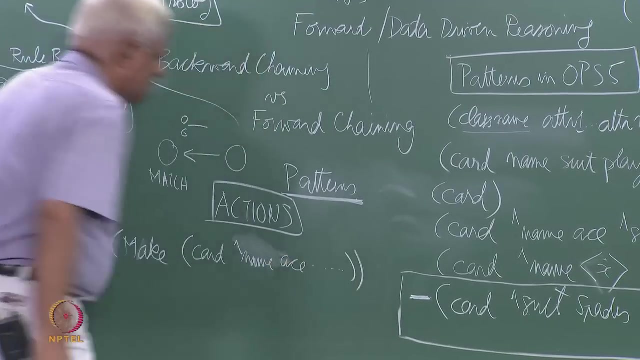 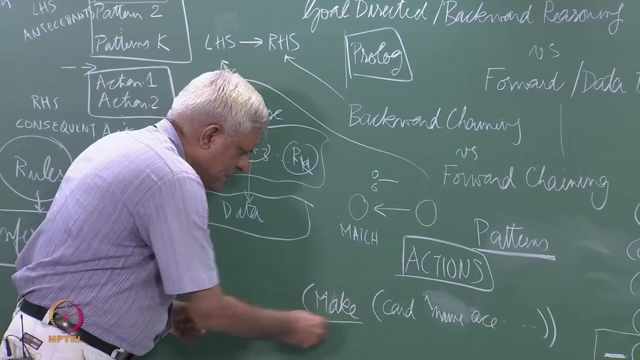 important actions in op swipe is one is called make and after this you describe the working memory element. So you can say, for example, card spades- sorry, suit name ace, and so on and so forth. So what action does this make action? it creates a working memory element and puts 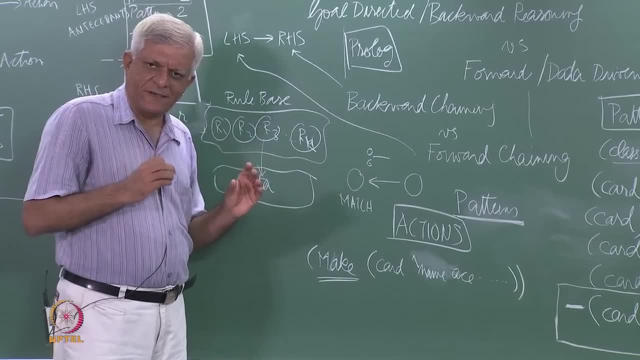 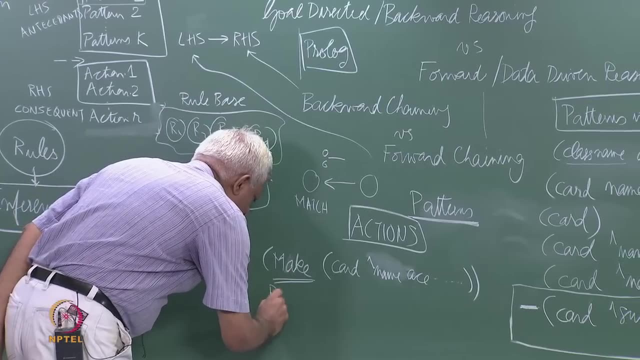 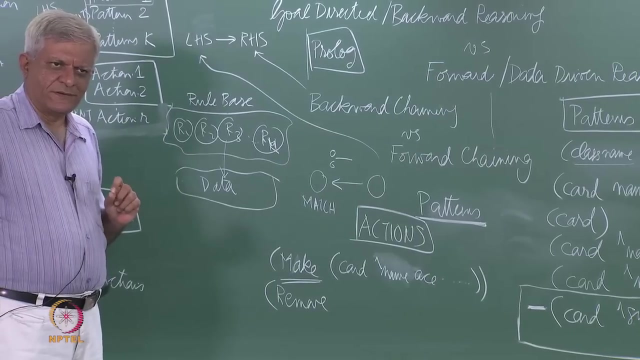 it into the working memory, or it. in other words, it creates a data element and puts it in the database, if you want to call it a database. Corresponding to this, there is also a remove action. Now, a remove action takes an argument like two and the action takes. 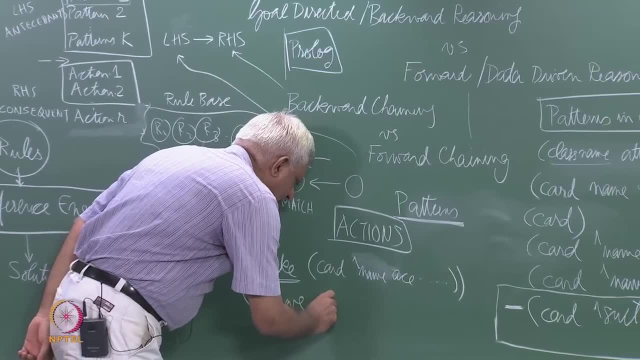 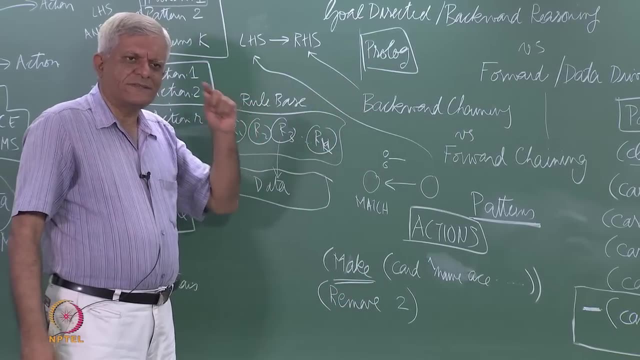 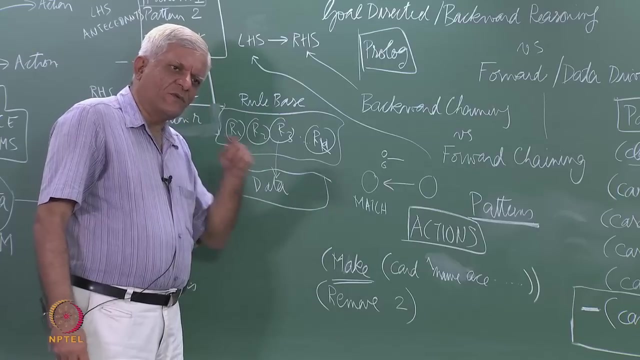 two like the rule 2 and this two Japan y sorry, luxurious. and this two, as you will see in the example, refers to the second pattern in that particular rule. remember these actions are on the right hand side of rule and this action is saying that: remove the. 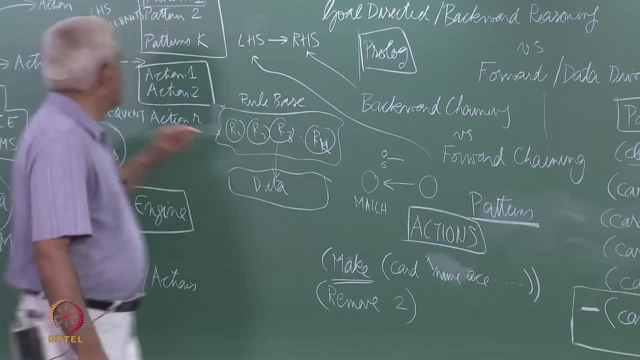 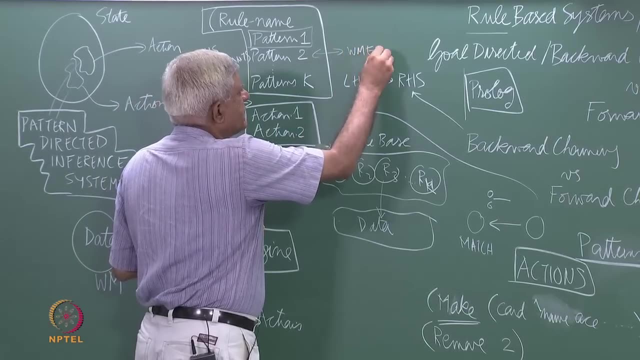 pattern. remove the data element with. match the second pattern. So this pattern number two matches some data. So that will match something based on some working memory- x, let us call it- and this action is saying that: remove that from the working memory or. 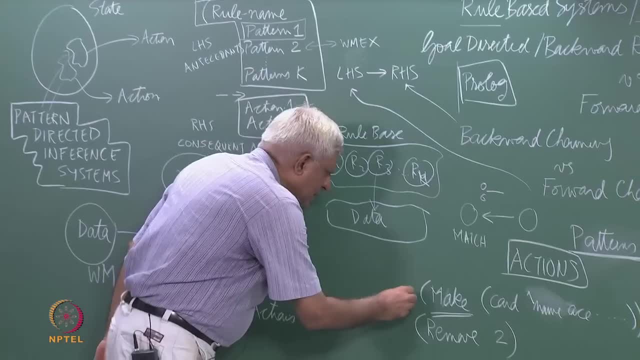 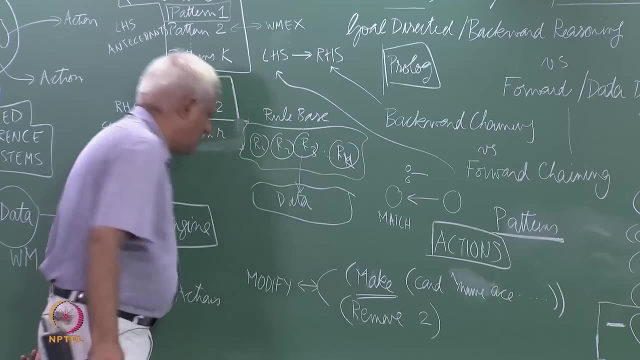 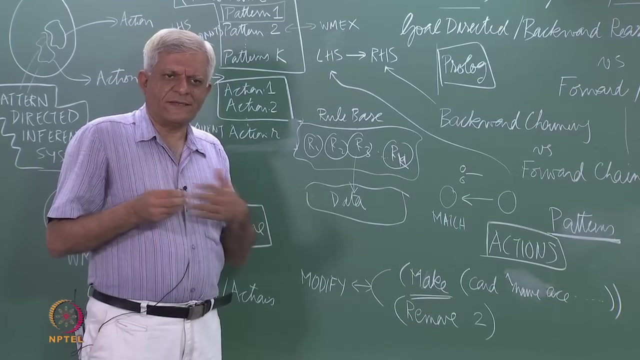 remove that from data. essentially, If you can combine this, you can have an action called modify. So, for example, as a game progresses, you want to change the rank of a card essentially. So let us say somebody has played the ace of spades and now you want to say king of spades has rank one. then you 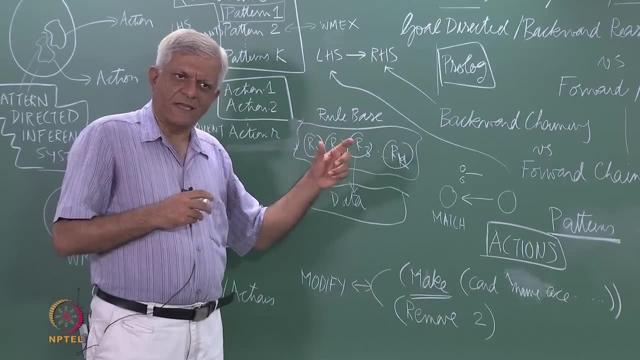 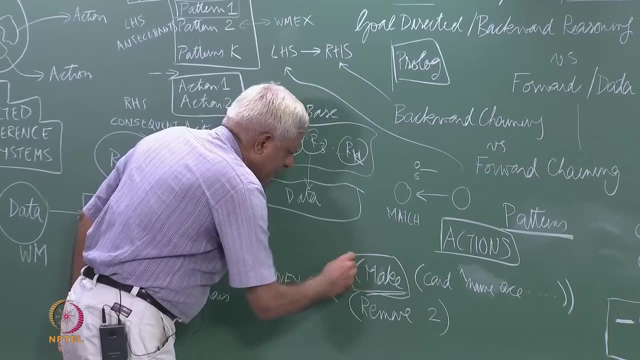 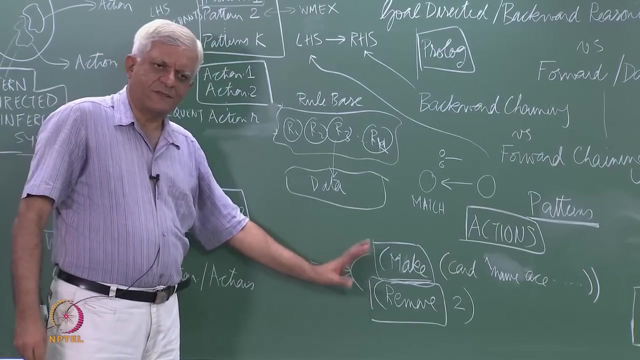 could say: modify that particular working memory element and change the rank to value one, and so on. So we have the. basically, we have these two actions, make and remove- but this can lead to a third action, call. any modify action can be seen as a combination of make. 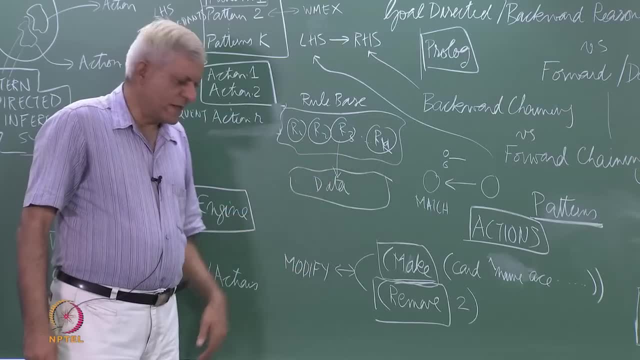 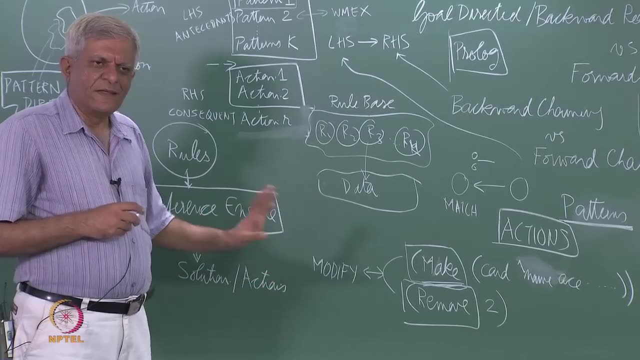 and remove and make it: remove the old one and put in the new one. it is like modify. Apart from that, you have standard actions that you may need, for example, reading from a file and so on, which we will not go into here because we want to focus more on. 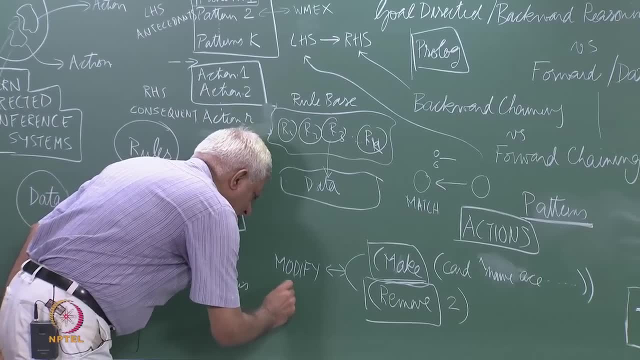 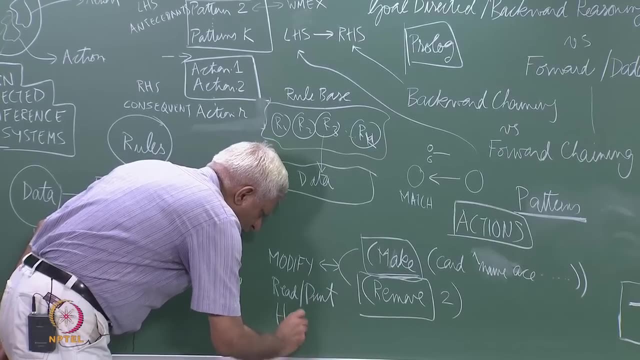 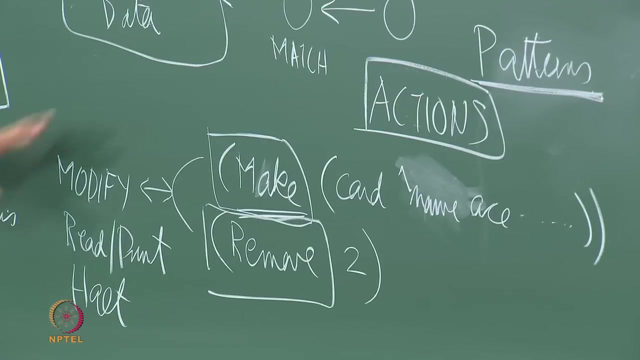 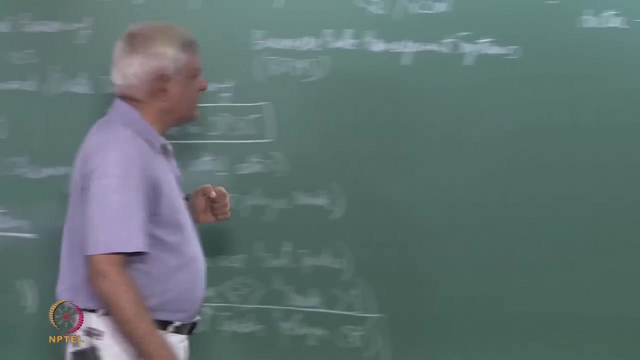 reasoning is done. So there are actions like read, write, print. There is even an action called halt, which says that stop the system essentially and exit essentially. So we will not look into those details here. So let me now give you examples of a few rules and 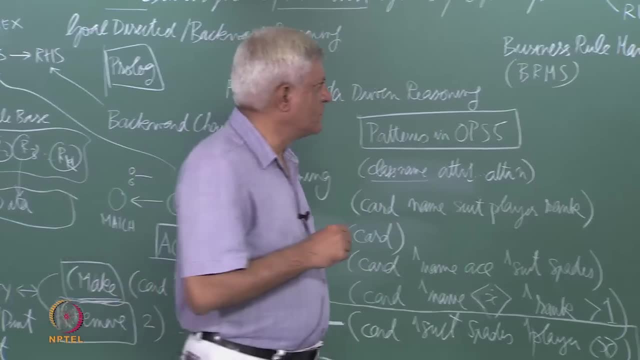 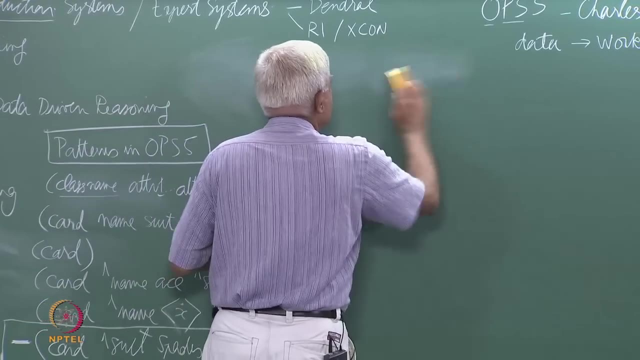 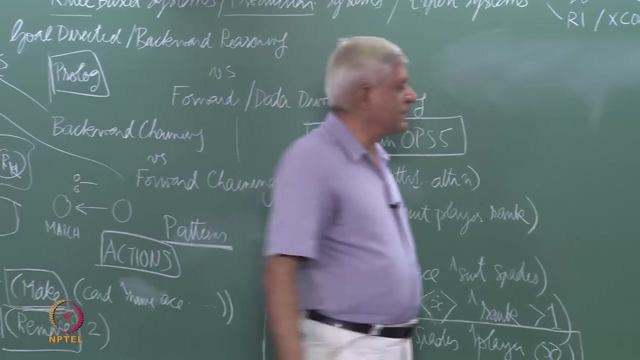 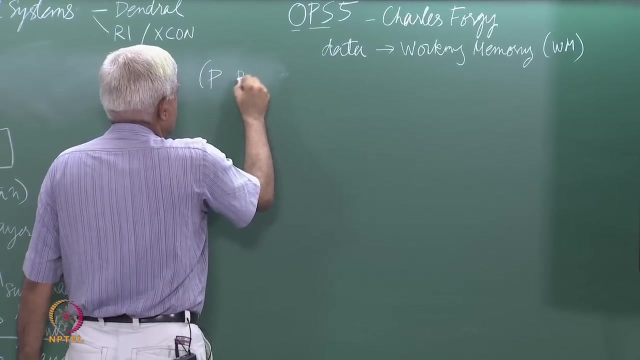 then we will see how the system operates with these rules essentially. So I will write these rules for a card game, and I assume that everybody has some inkling of what card games are like essentially. So let us say we have a rule called play. 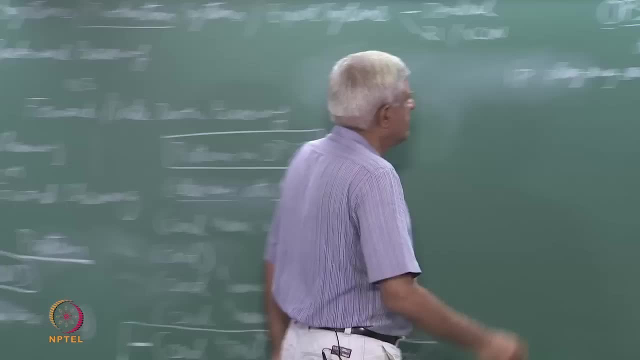 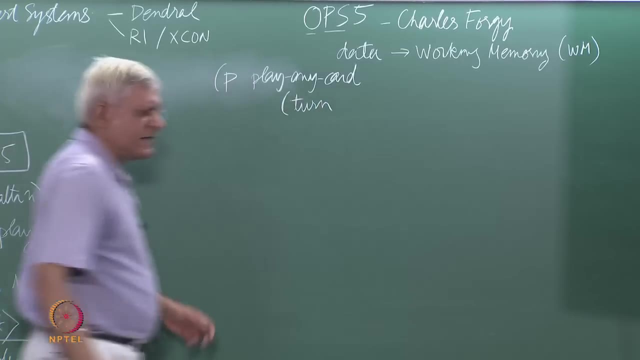 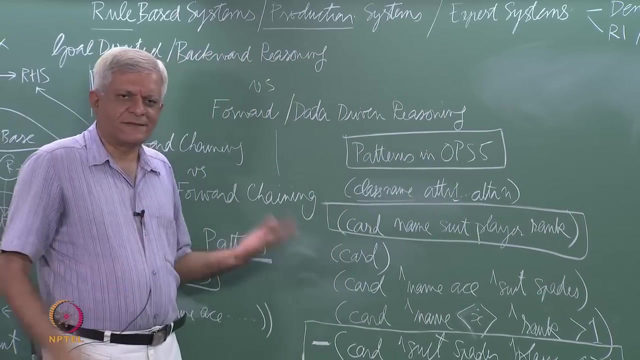 any card and the pattern is: let us say, there is a class name called turn, which I have not described. I have only described one class name here, which is this, But obviously you will have many different class names in your system. 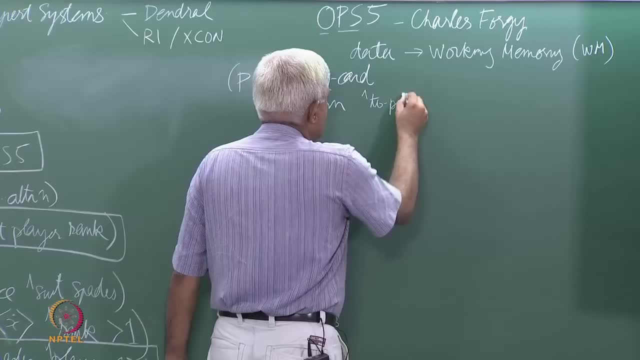 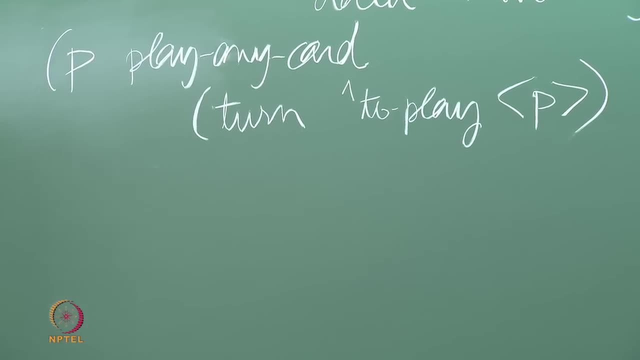 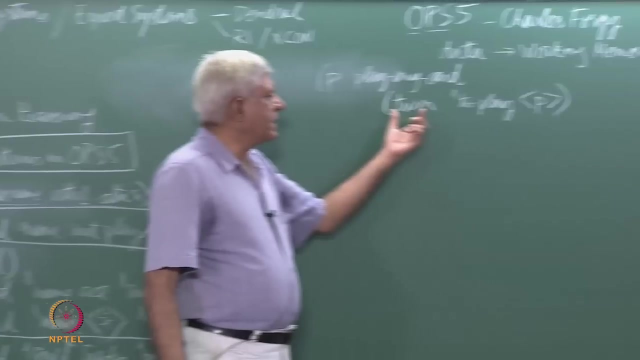 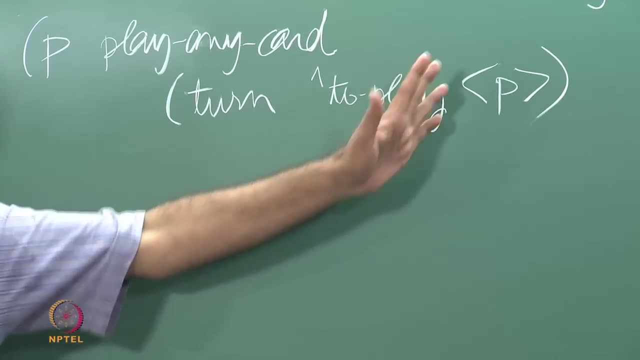 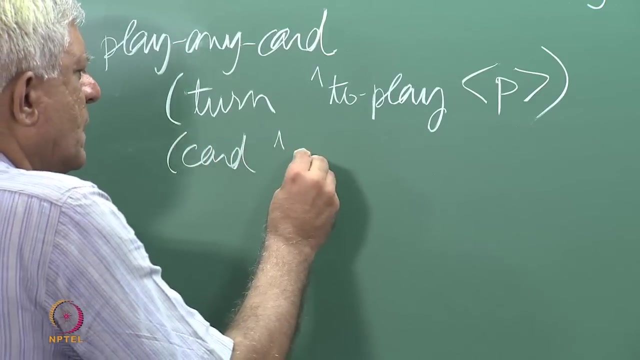 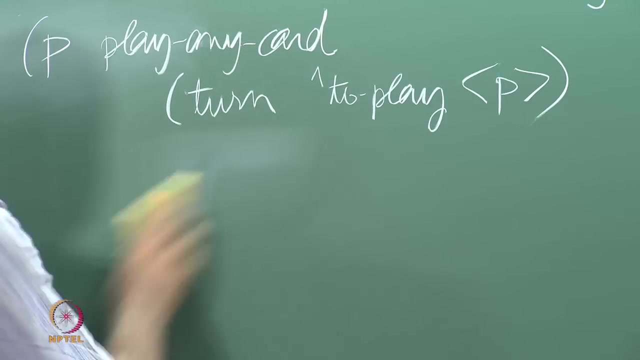 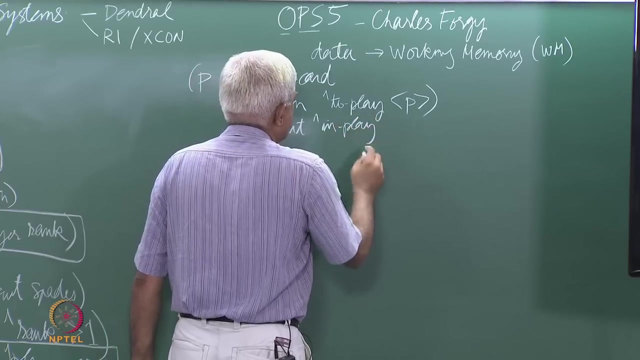 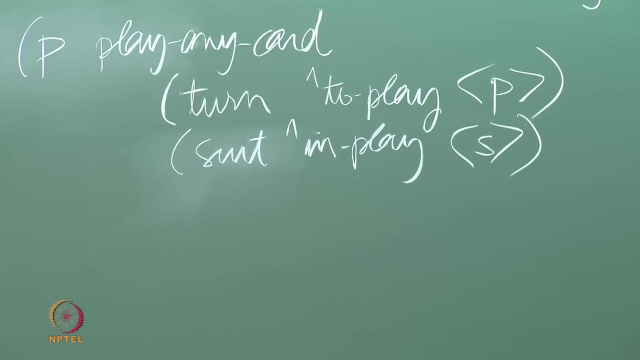 Let us say that already somebody has started playing a particular suit. There are many games in which you have to play the card of the same suit as somebody else has done, So 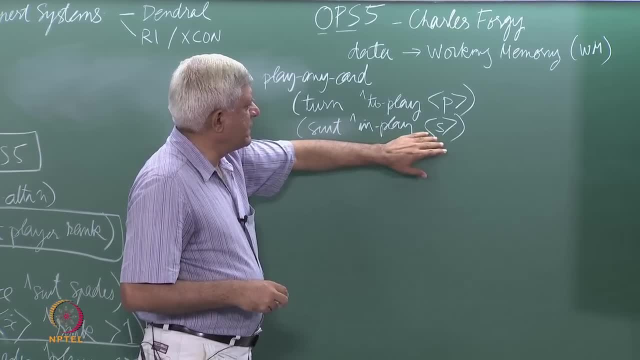 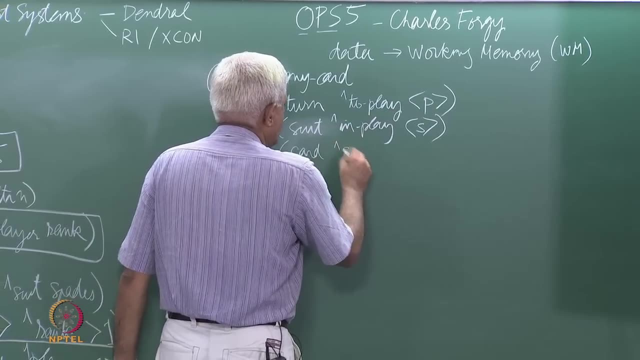 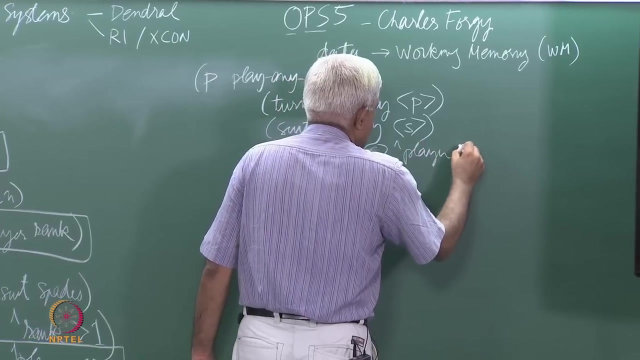 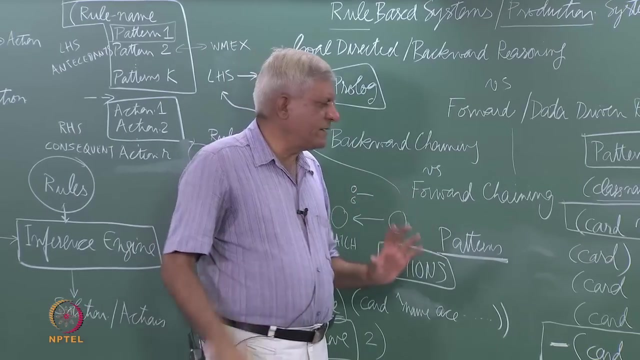 this is saying that the suit that is in play is S, some variable S, and this is some player P, and this player has a card of suit S. So notice that there is no order sanctity here. essentially, I may say that it is name, suit, player, rank, but that does. 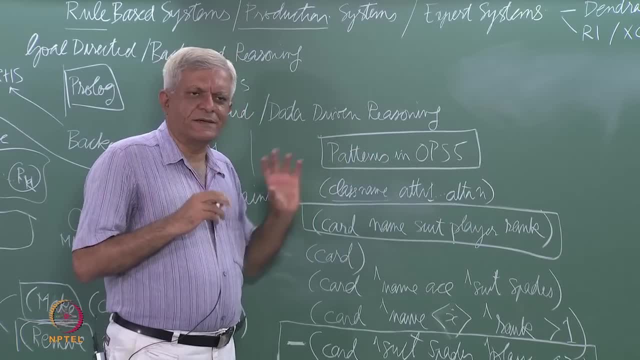 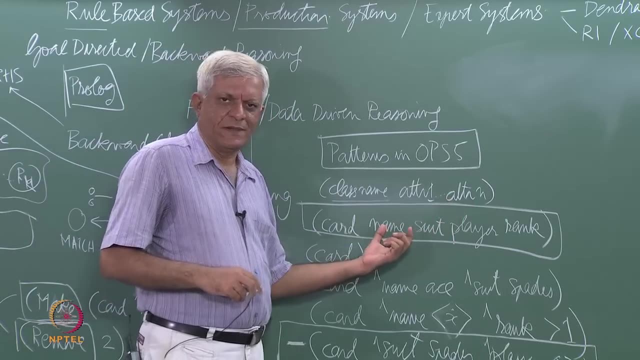 not matter, because we are segregating the attribute names with the attribute values. You can specify the name of the player and you can specify the attribute names in any order. You do not have to specify them in this particular order. So here I have, said card with suit S, player P. So all I am. 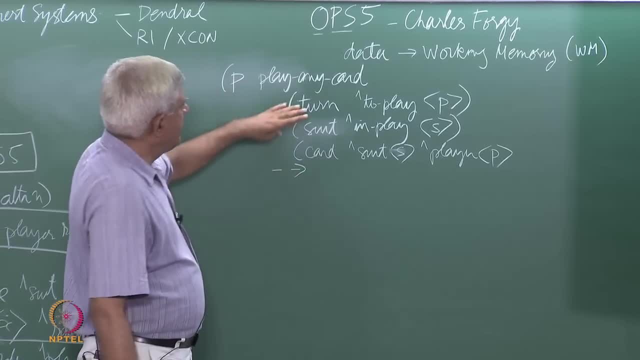 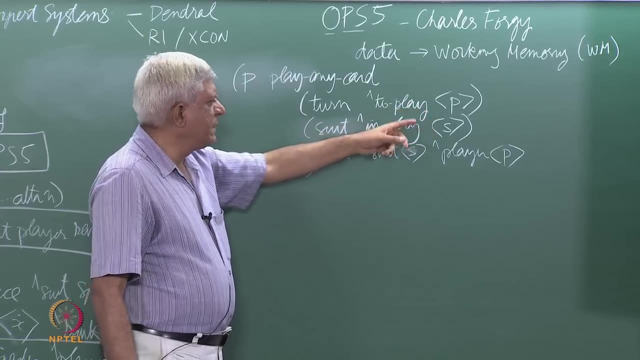 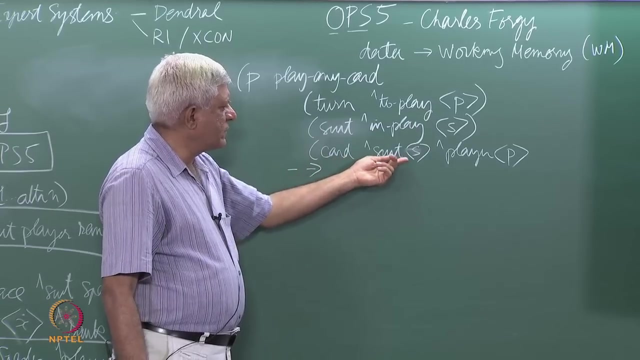 saying so what I am saying here, that if it is a player's turn to play and the player could match anything, and if the suit in play is S and if there is a card which is of suit S and it is being held by player P, then that player P should play that card. 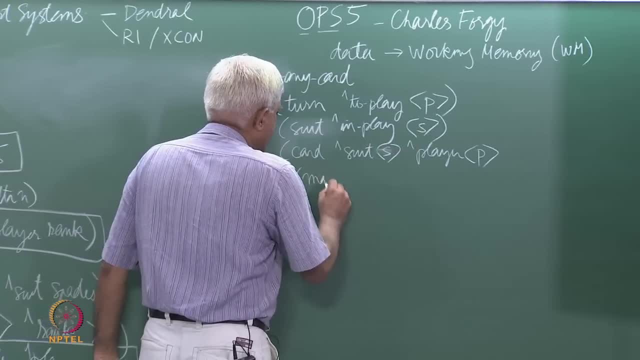 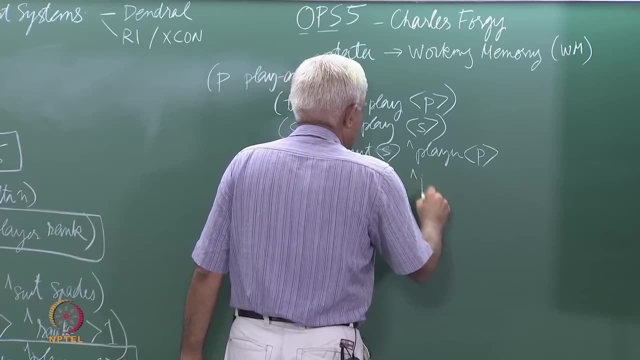 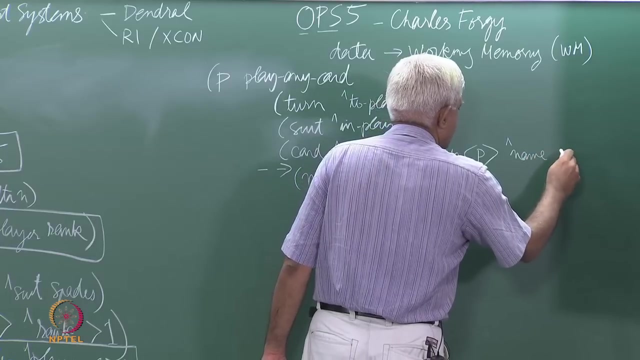 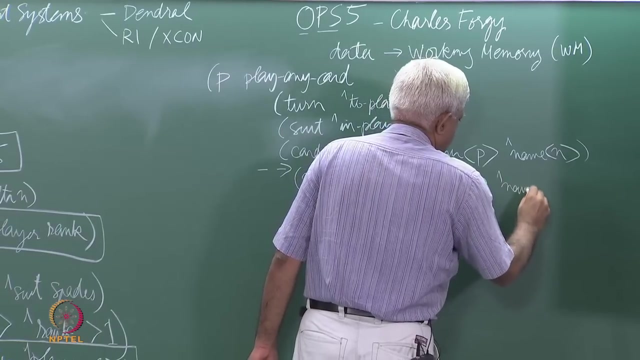 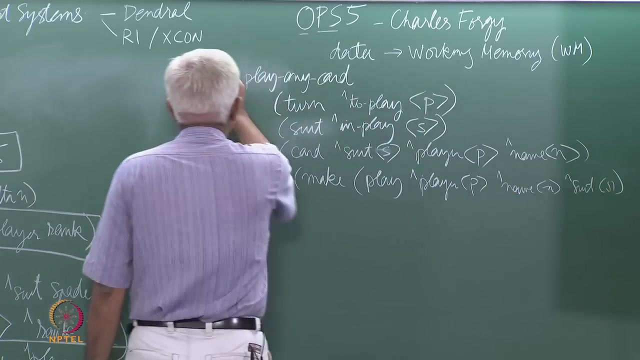 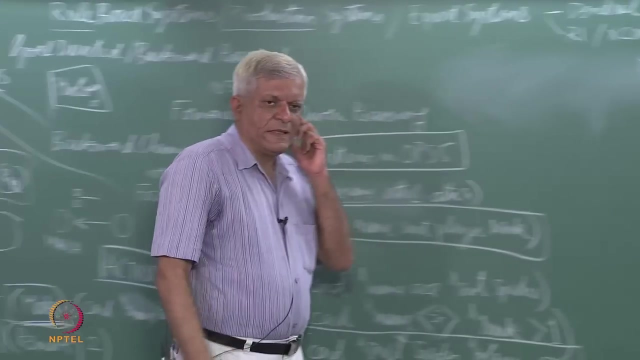 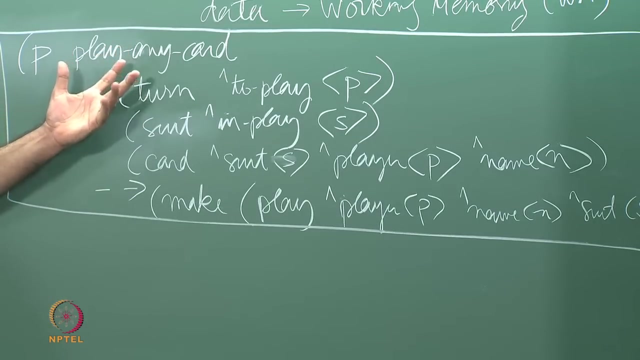 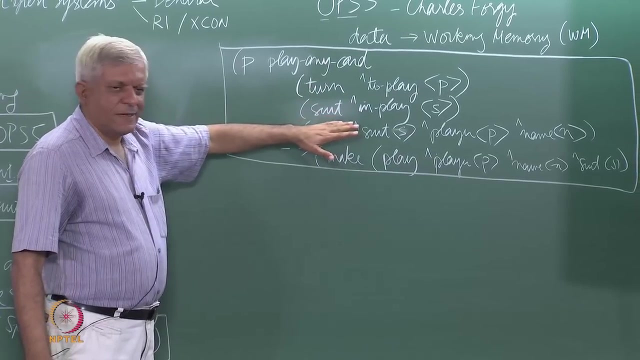 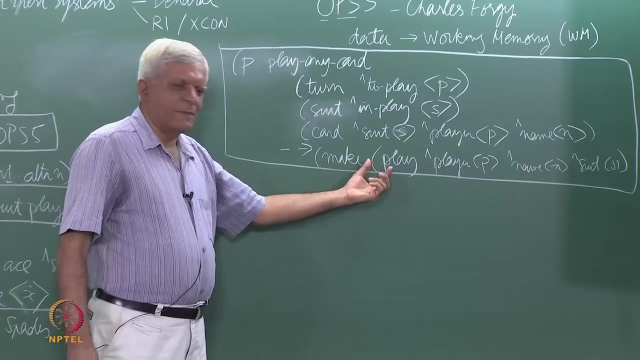 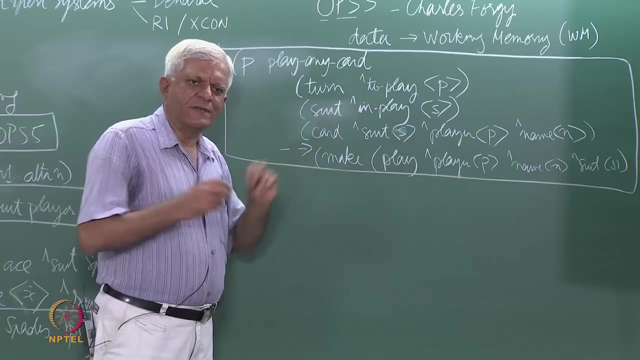 So let us say, I use this make. 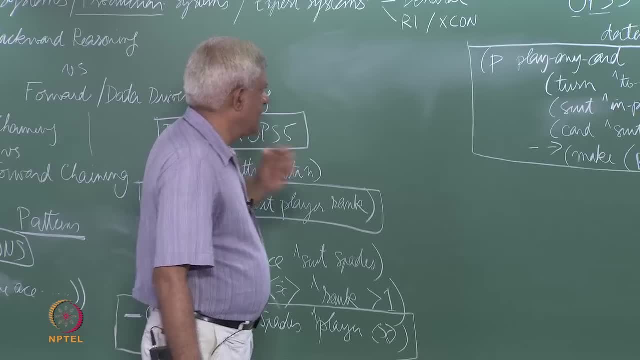 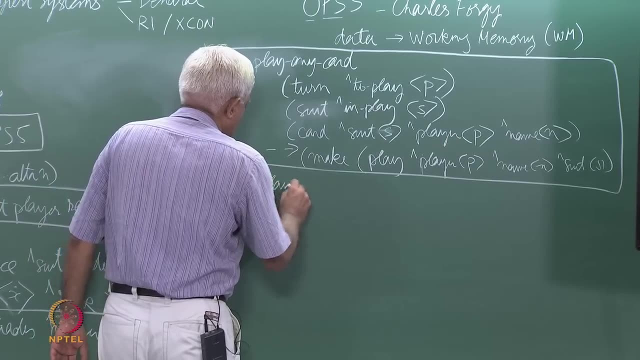 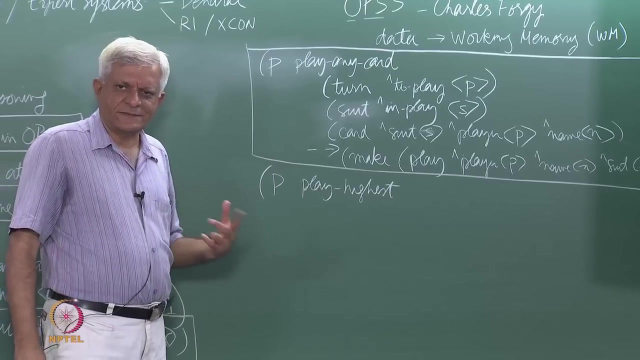 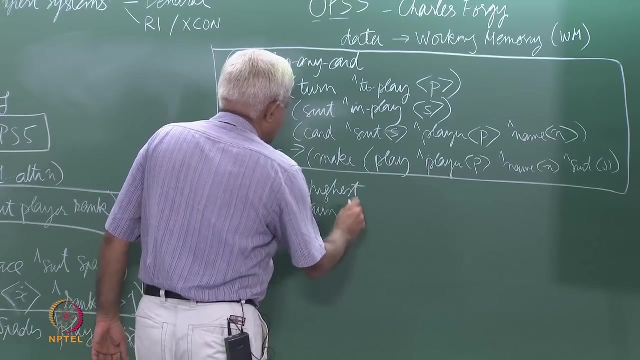 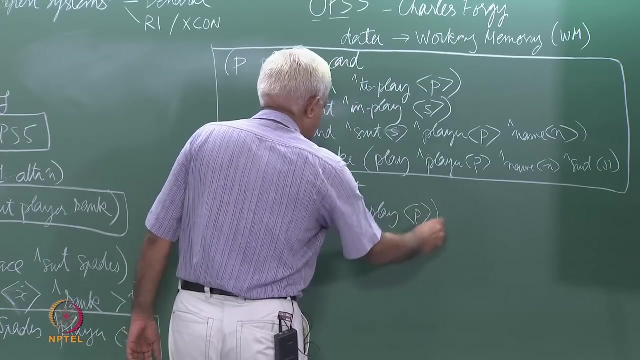 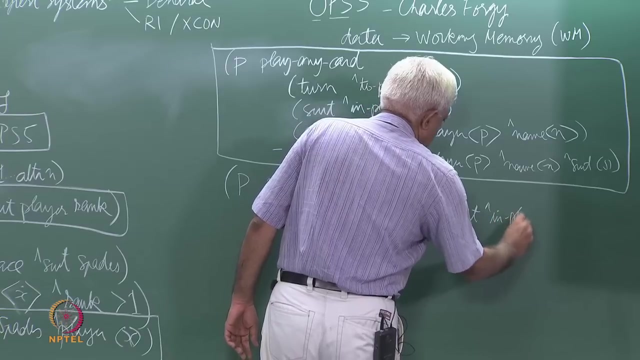 So let me give you another rule just to. So if you want to not play any card, but you want to play the highest card, essentially, then what should the rule look like? the first two will be the same term, So let me write this here. So the first. 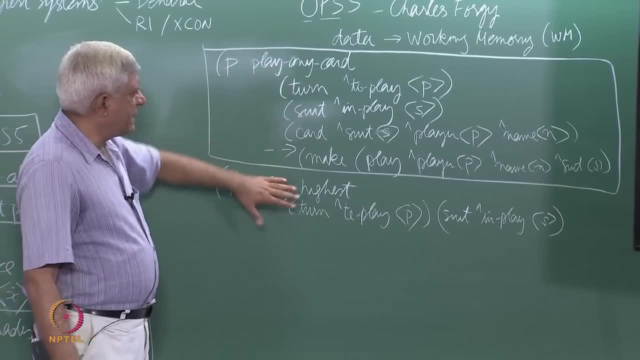 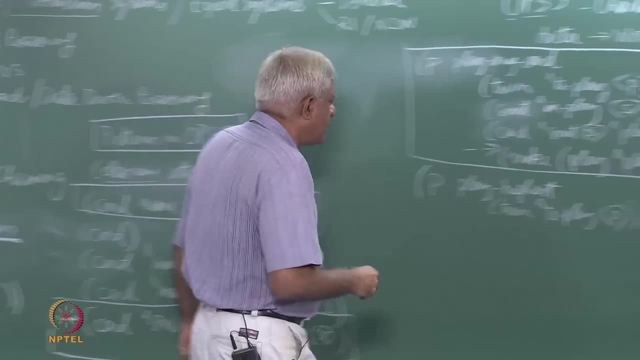 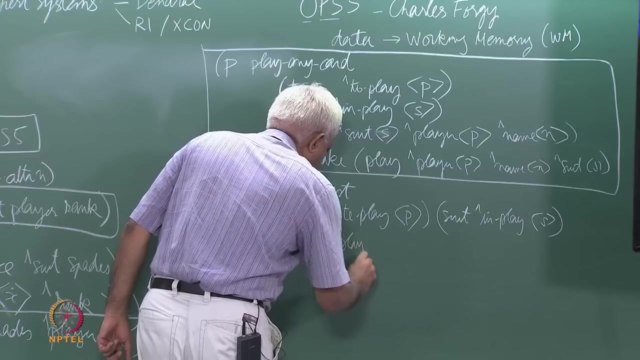 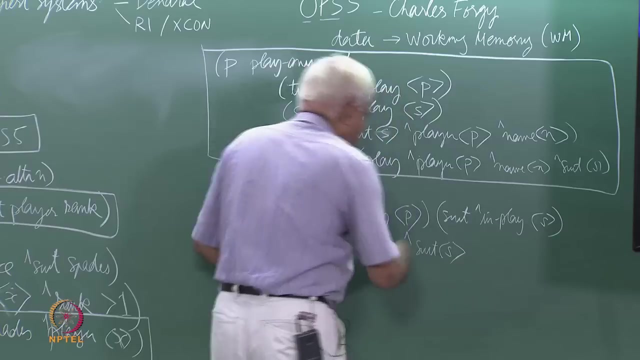 two patterns are still the same as this rule, but the other patterns will change. Now we want to specify that the card that you play must be the highest card in the suit, And we can do that by saying the following: let card player P suit S. So first, of course, we are looking for a card being held by this. 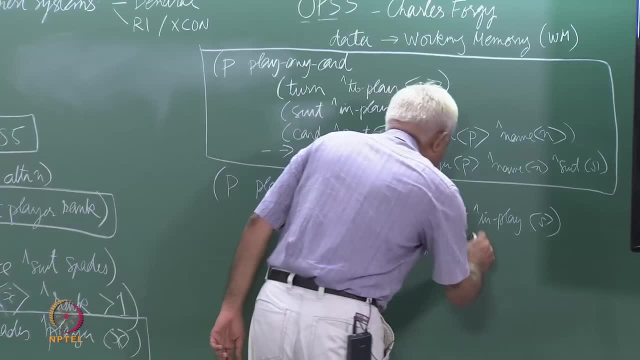 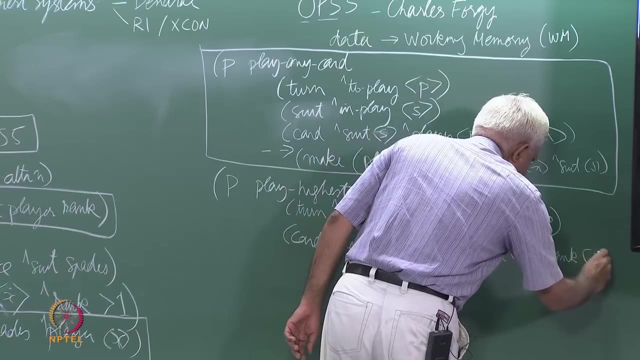 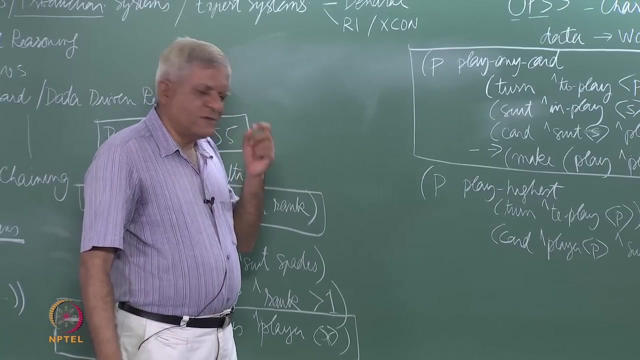 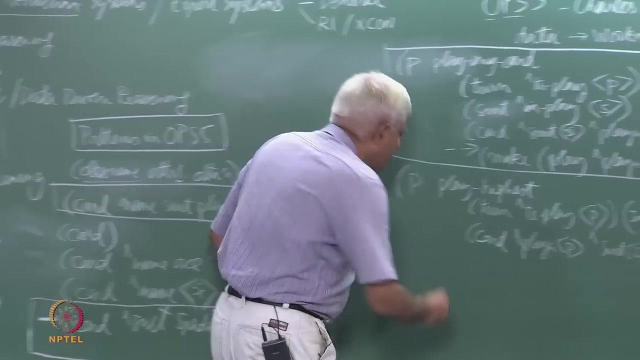 player and in this suit. So let us say name, N and rank, Because we are interested in picking the highest card. we should talk about the rank and we should say that there is no higher card. It means we can say that there is no. 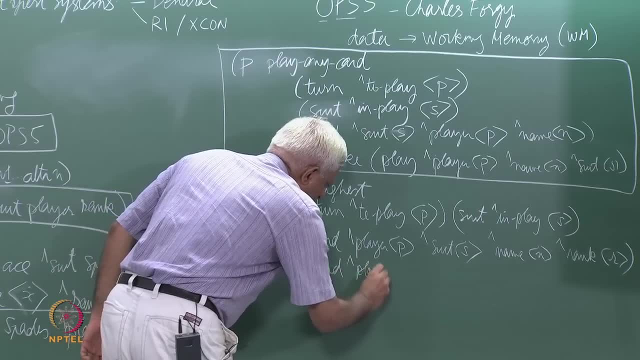 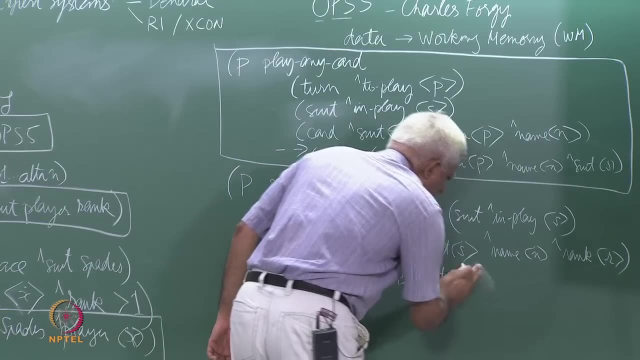 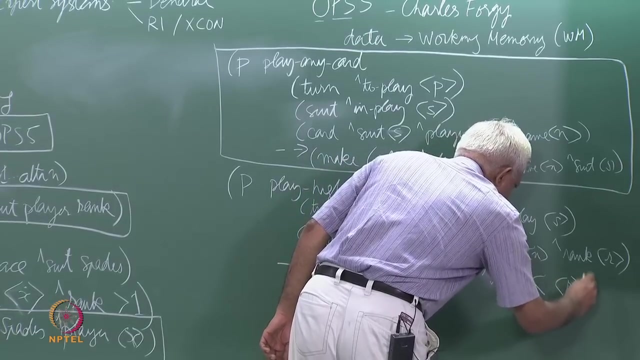 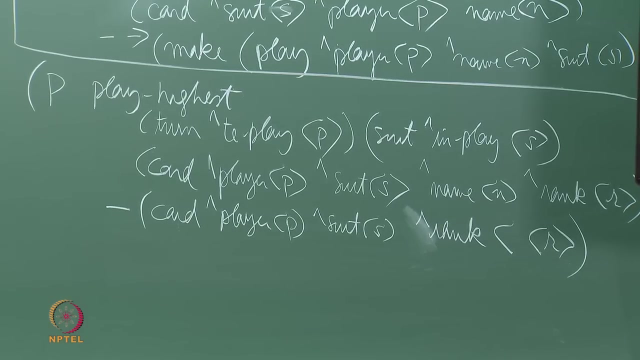 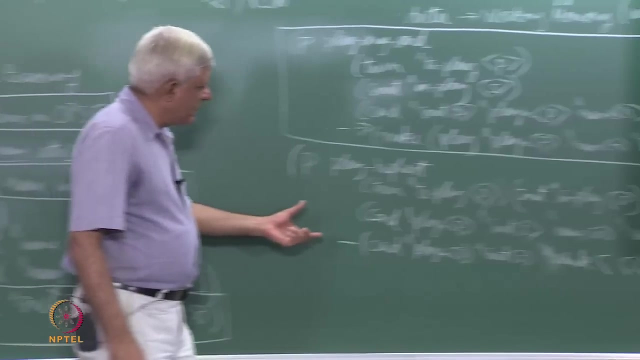 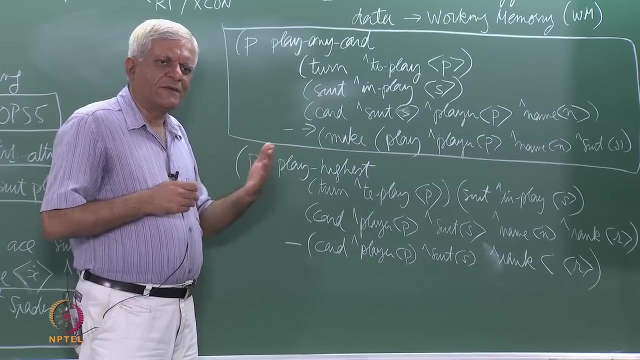 card, the same player P name we do not care about. So let us say that there is no higher card. So this is a that negative thing that I was telling you about. So, between these two patterns, we are looking at a set of data elements and picking the one with the highest. 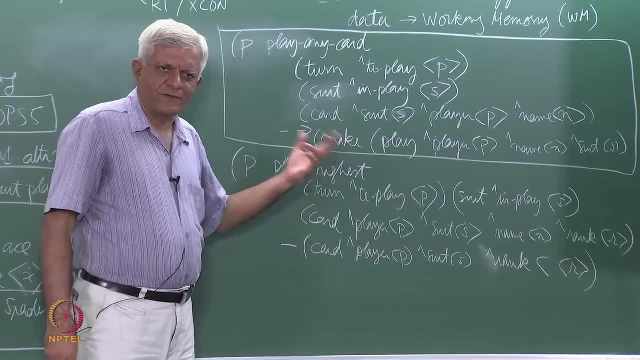 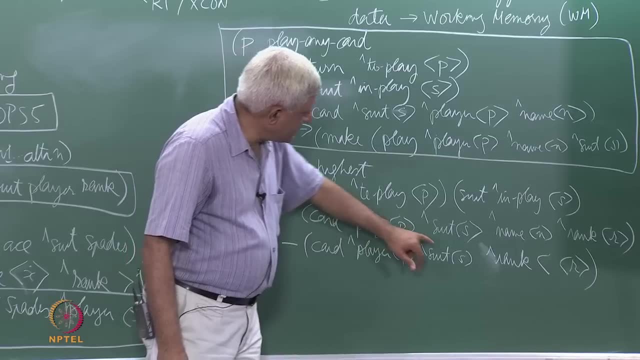 rank, which means the lowest number, rank 1, we want to look at rank 1, we want to look at or rank 2, whichever is the lowest available. So we are saying that card player p suit s name n rank r and there is no card with this player p of this. 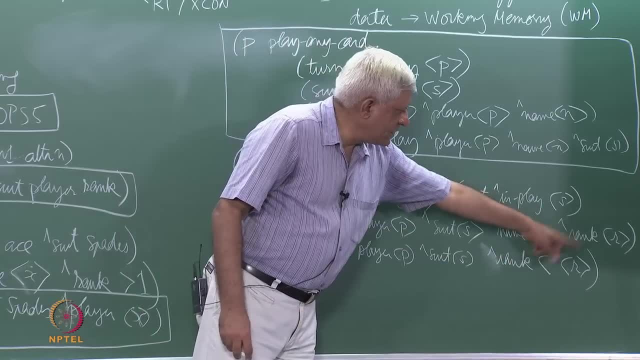 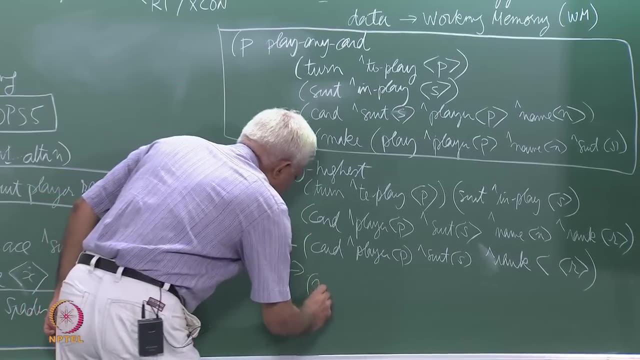 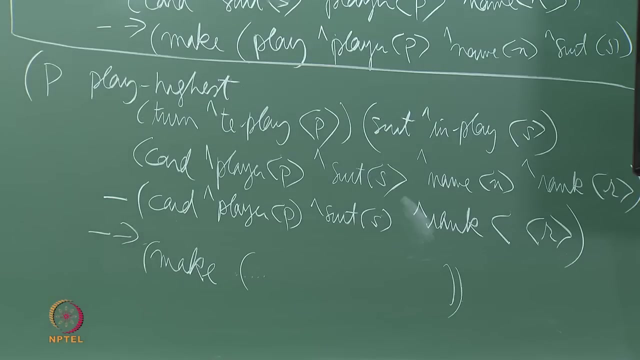 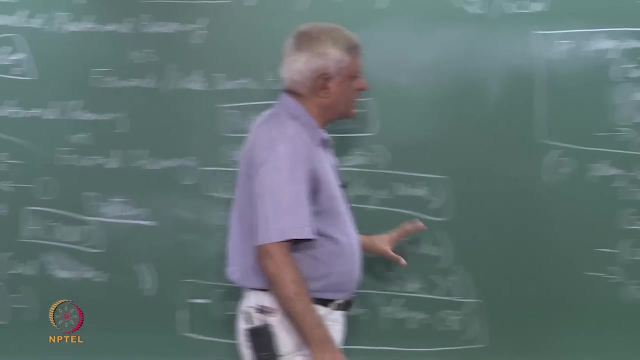 suit, same suit s whose rank is smaller than this r. So obviously this r and this r must match the same value, then the same thing, and you can write more rules depending on you know what kind of game you are playing and what is the strategy you want to adopt. and 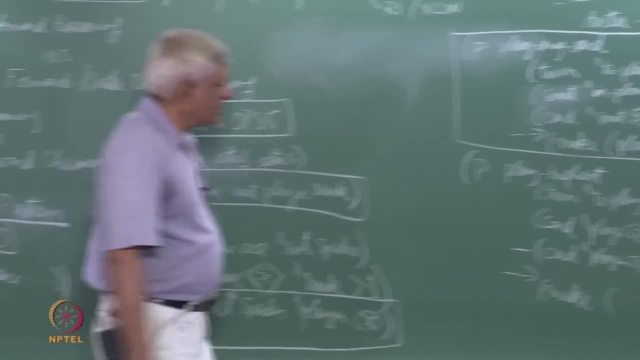 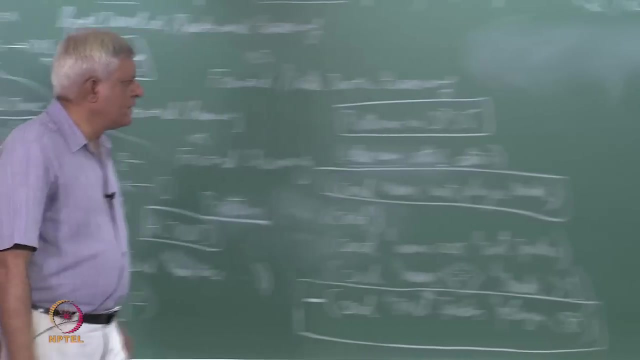 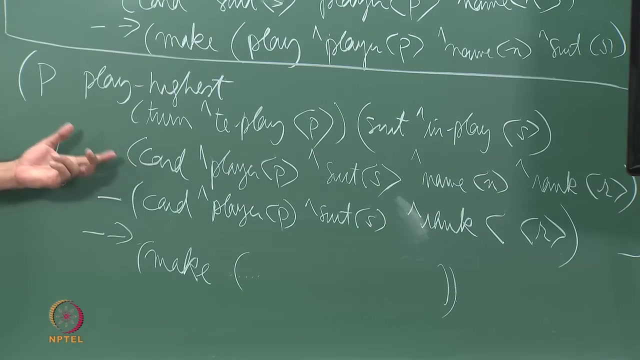 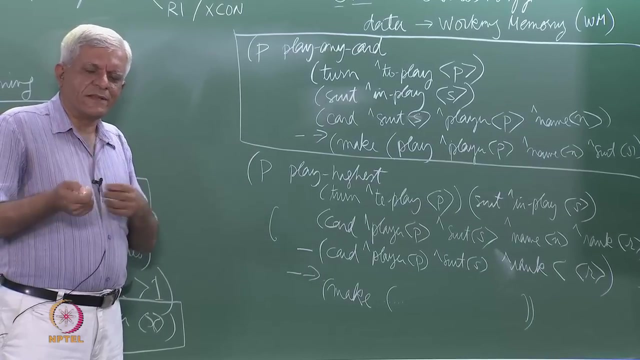 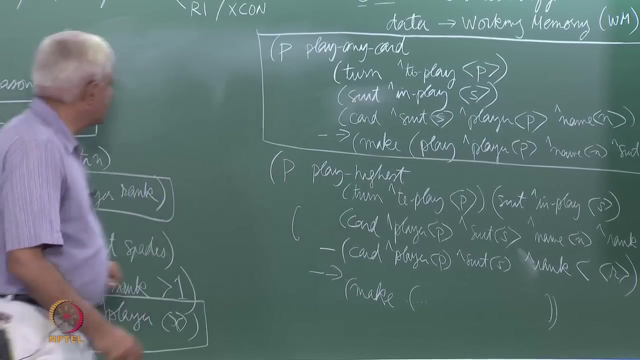 that kind of stuff. but we would not get into those details here essentially. but you should observe that this one 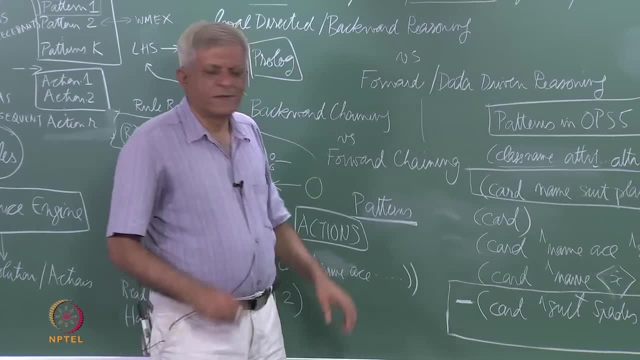 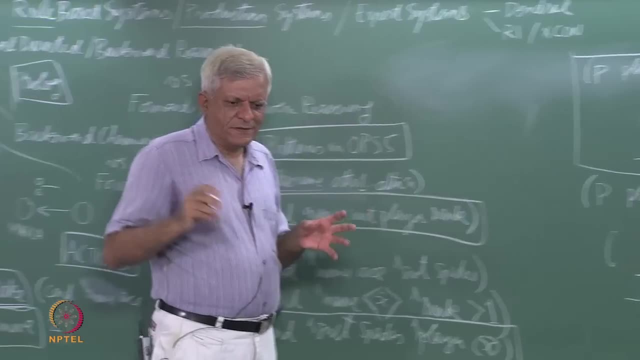 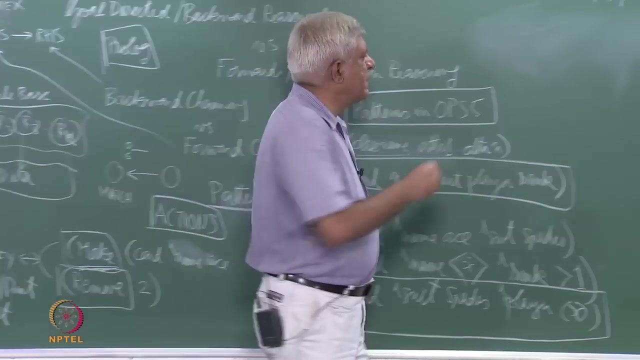 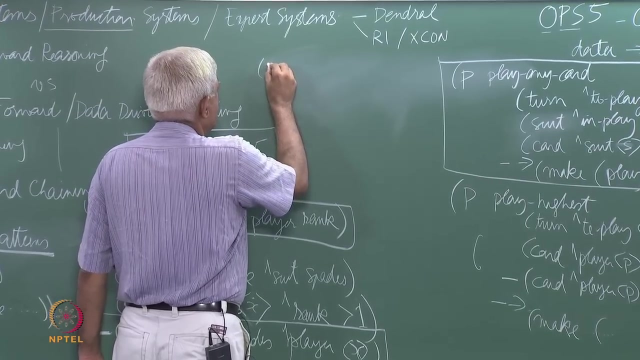 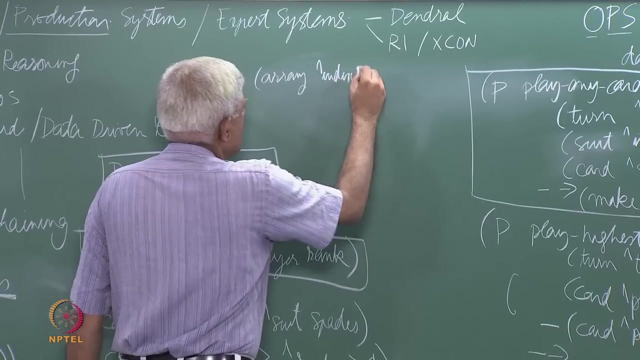 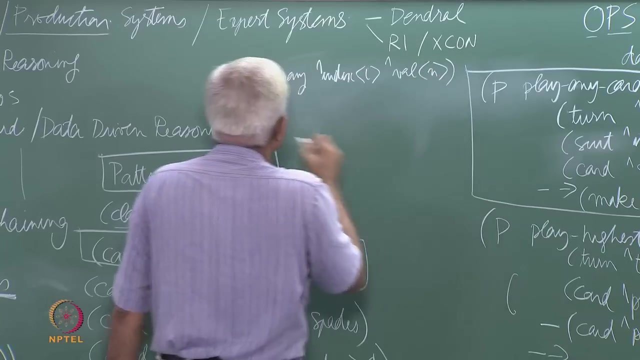 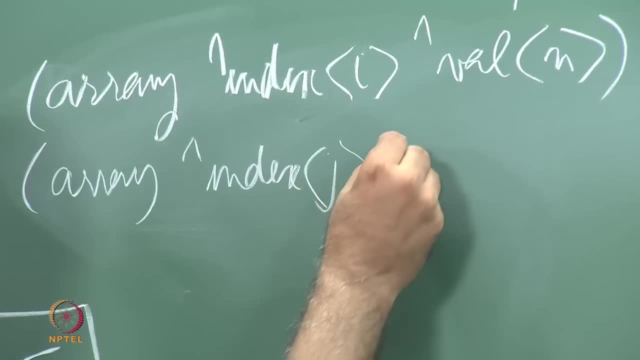 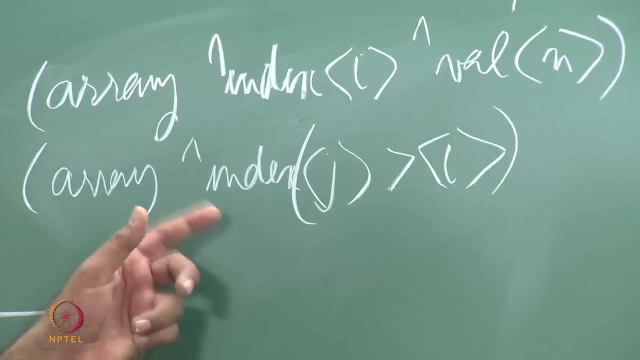 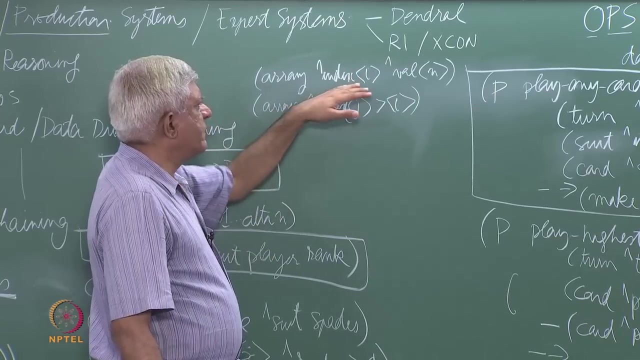 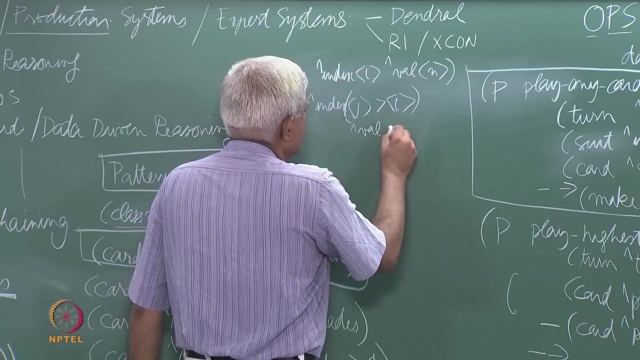 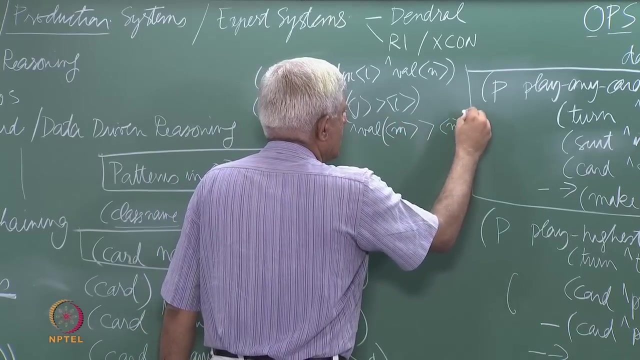 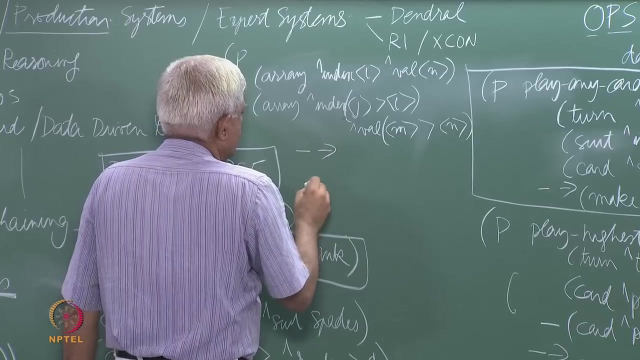 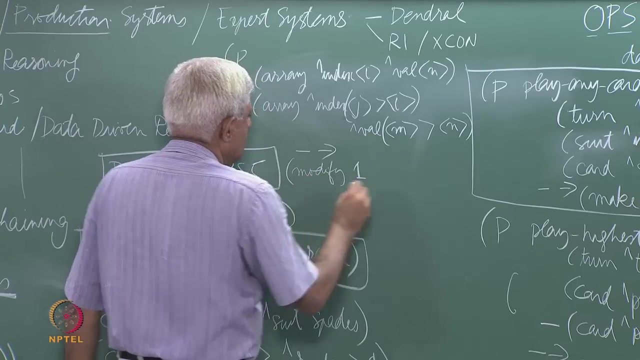 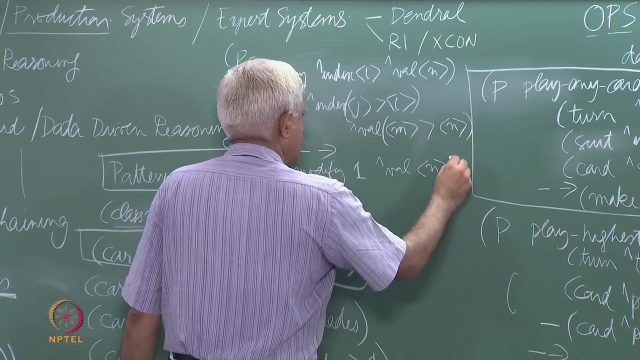 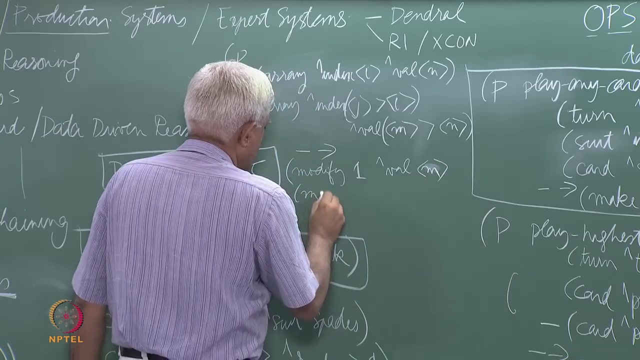 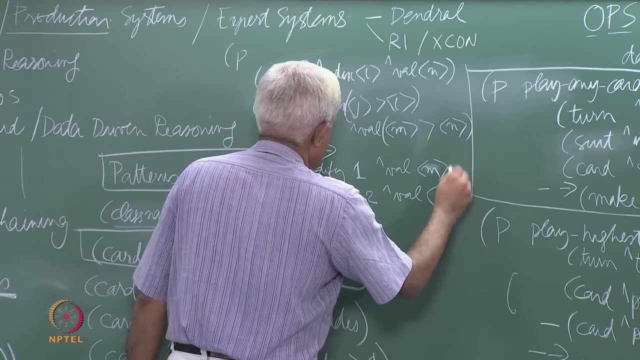 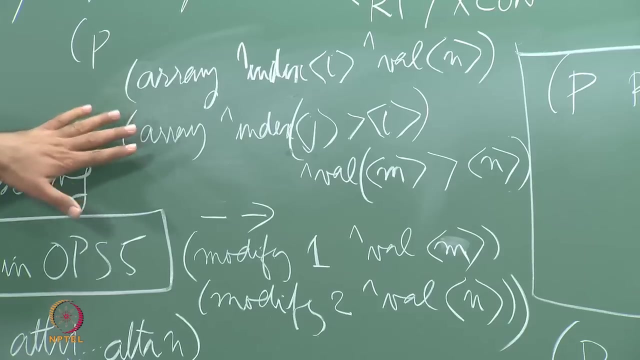 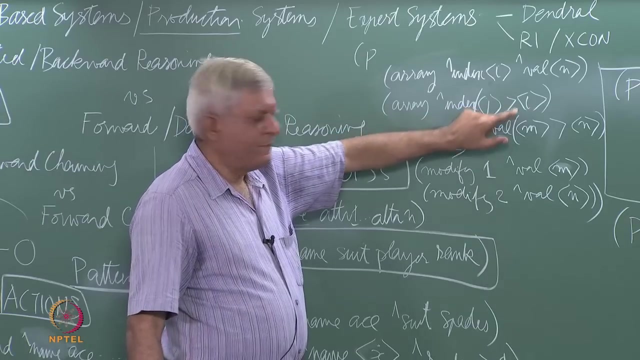 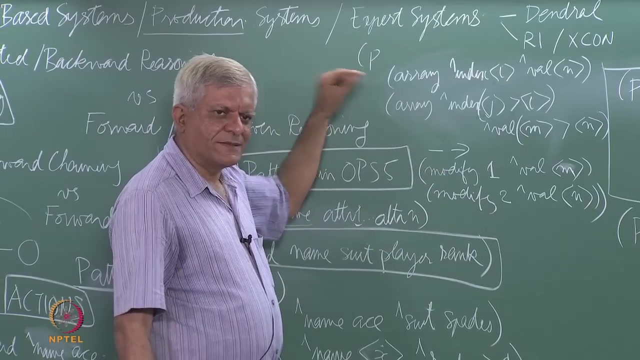 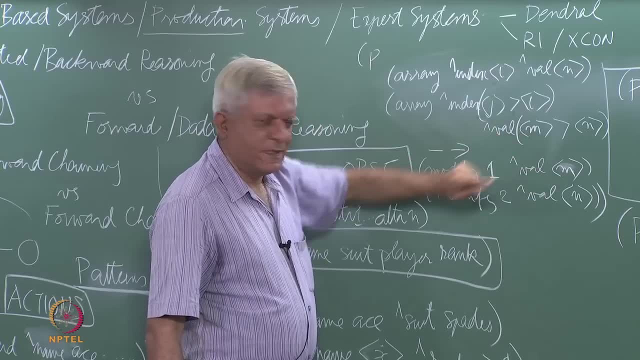 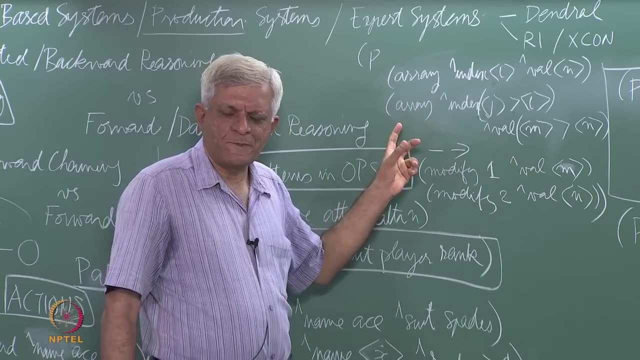 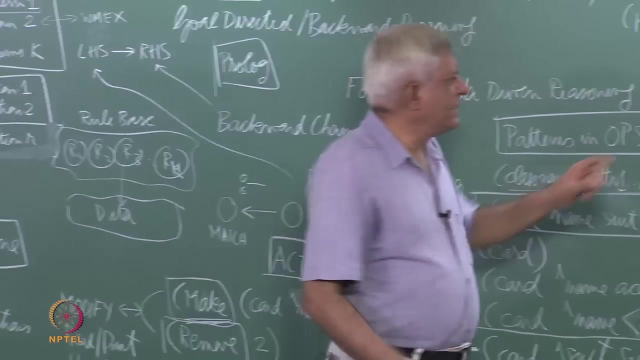 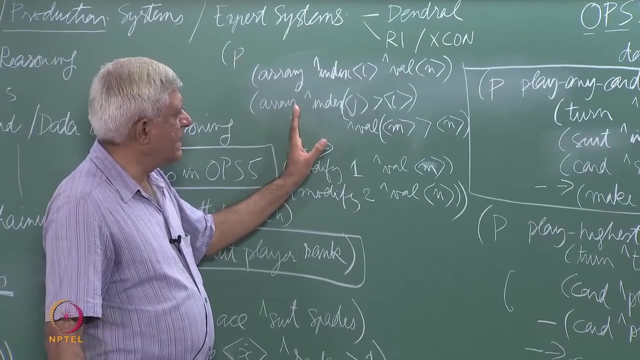 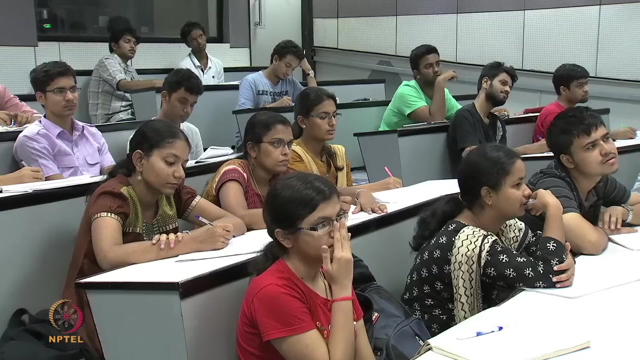 its value attribute to m, which is what I have taken from here, and modify the second pattern and change its value attribute to n, essentially. So what am I doing here? I am swapping two elements. if they satisfy this condition right Now, this single rule, if I let it lose on the data, then it will end. 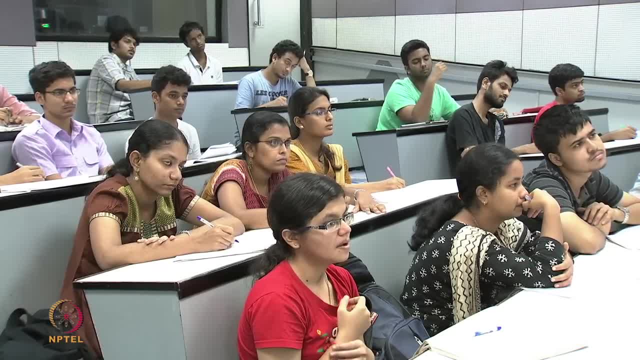 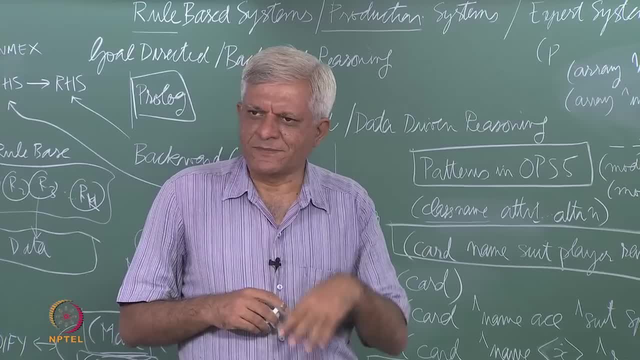 up sorting, as you said, the entire array essentially. So I so just think of you have written an algorithm for sorting elements. you have looked at all kinds of sorting algorithms and you wrote them, but here is one single rule. 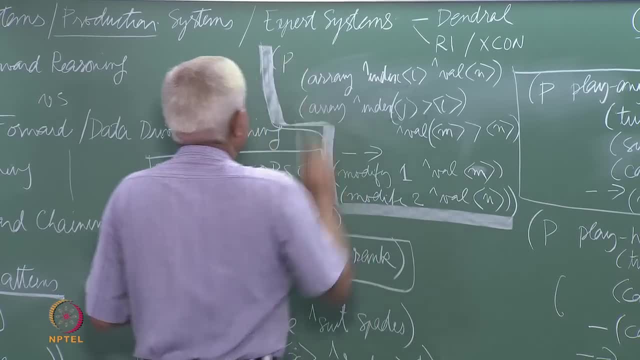 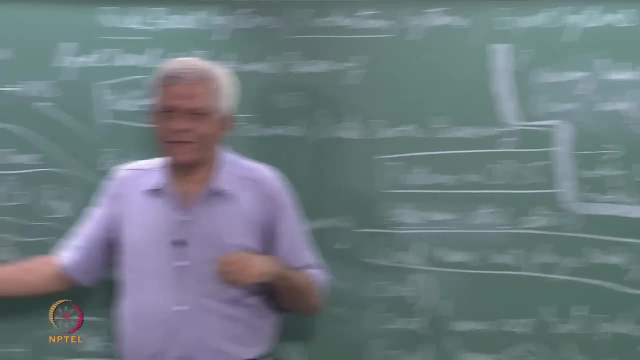 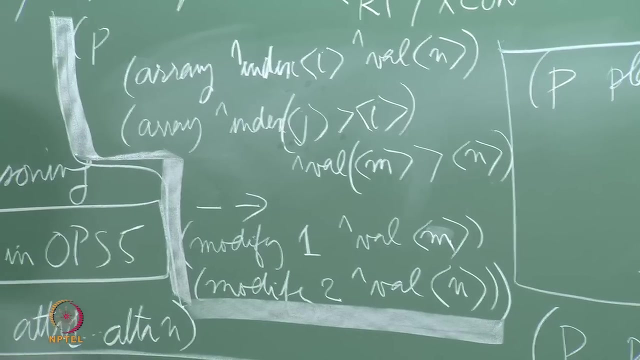 This much and this will do the job of sorting for you. essentially, It will repeatedly apply the rule and we will come to this repetition part in the next class, but it will repeatedly apply to. if it sees any two elements out of place, it will swap them. essentially, 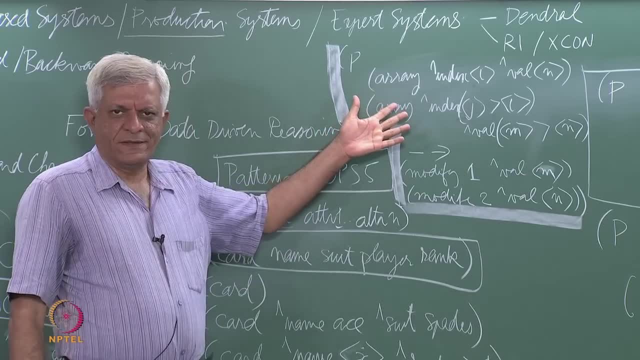 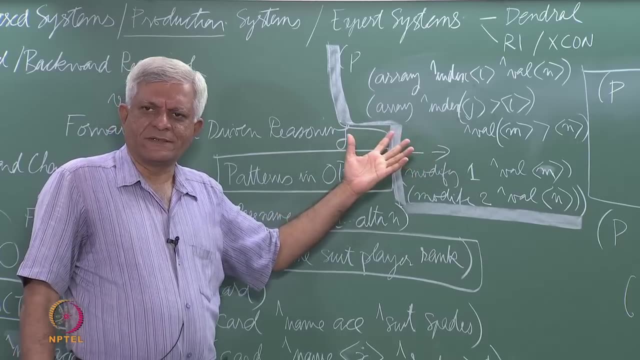 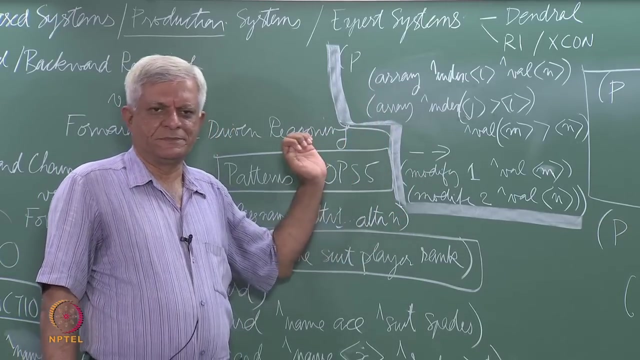 and it will keep doing that till this rule matches and eventually, of course, everything will be in place or sorted, and then this rule will no longer apply and your array would be sorted. So this also gives you something to think about. you can write up program, in fact. 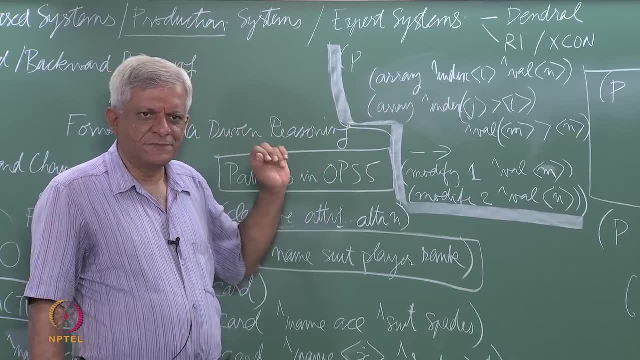 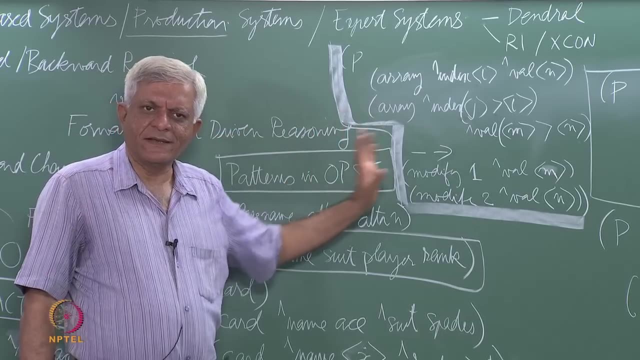 op 5 is a complete programming language like any other programming language, like prolog or C plus plus or Java or python or whatever, and you can write any program in any language. but in some languages some programs are simpler to write, So this program, of course. 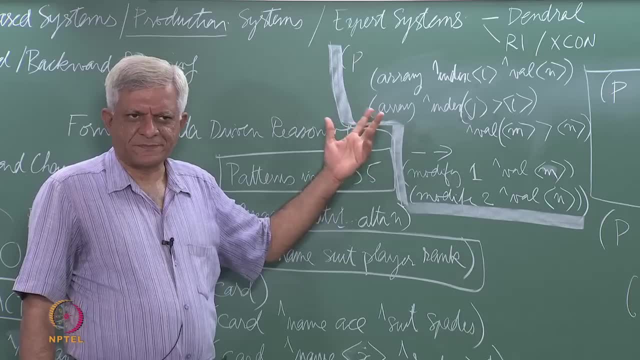 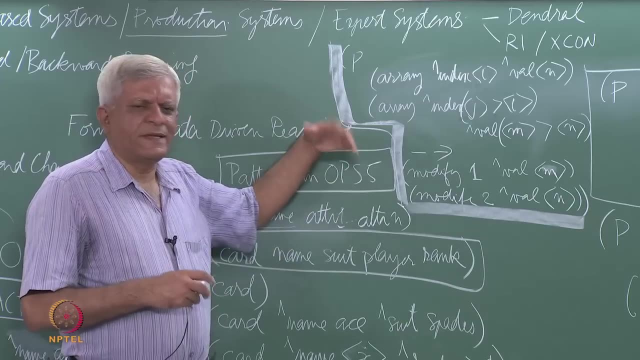 is very easy to write, but what can you say about it's performance? It will depend on so many other things which we will address in the next class. So, supposing you have many elements which are out of place, this influence engine here. 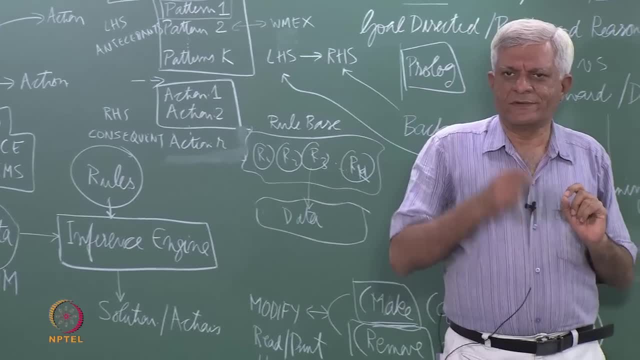 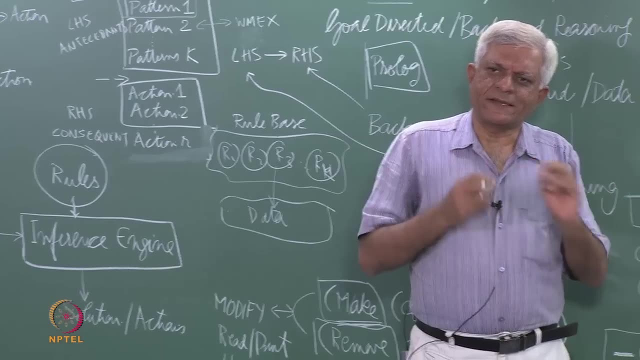 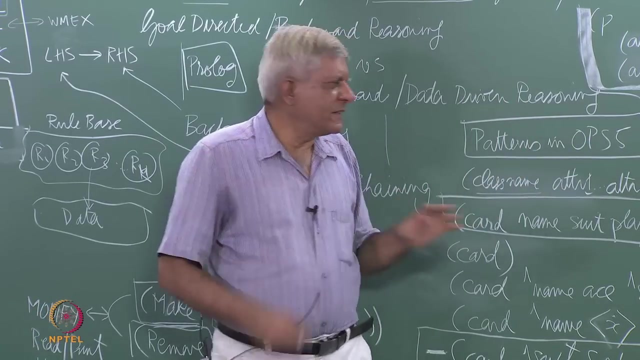 has to decide which instance of the rule to execute next, and therein, of course, lies the key to efficiency. If you exchange the correct elements first, then you will do things faster, and so on and so forth. but of course there is no way of knowing that here, but it is a very simple. 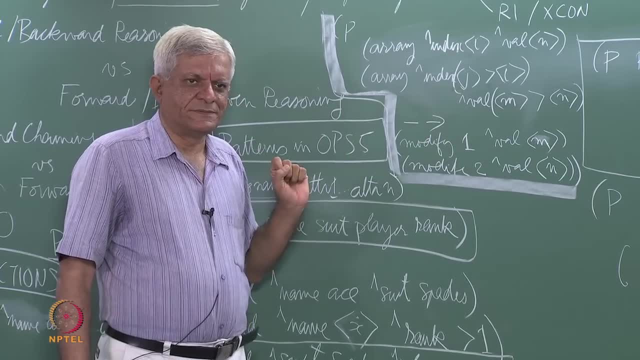 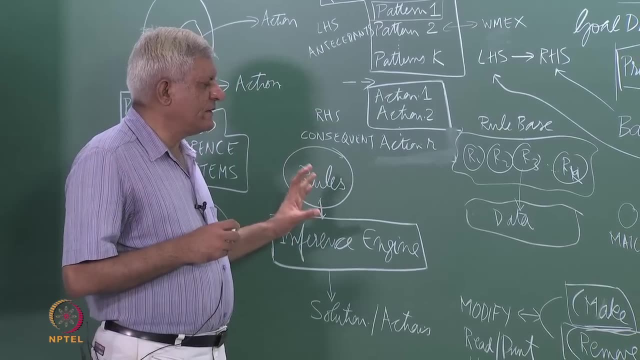 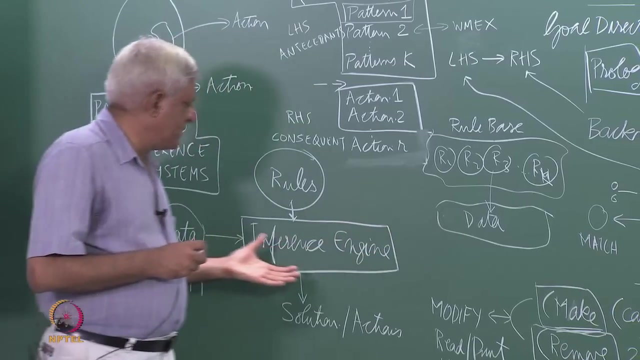 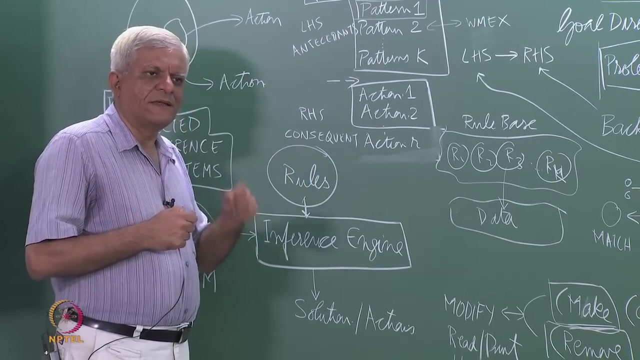 program to sort this. So the idea of rule based systems is that somebody sits and write down these rules in this thing and then we give it to an influence engine which basically does the influencing for us, which means basically it picks a rule, applies it. 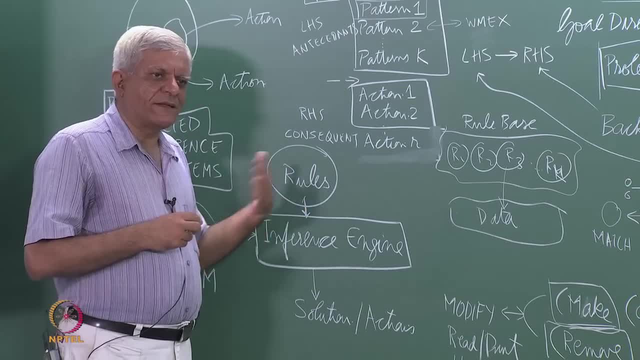 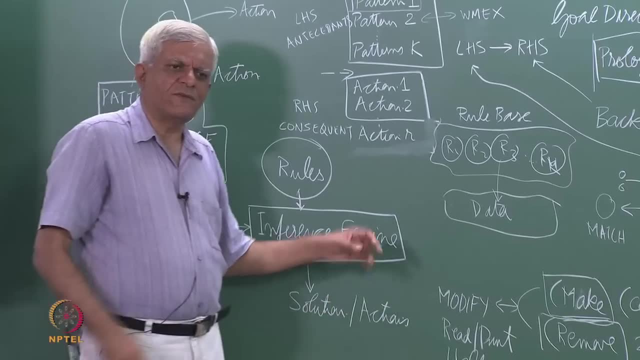 then picks the next rule and applies it and keeps doing that till it either runs out of rules to apply Or it runs into something like a halt. statement here, which you have explicitly given, may be: if you have a certain goal in mind and if that goal is achieved, you will say: if 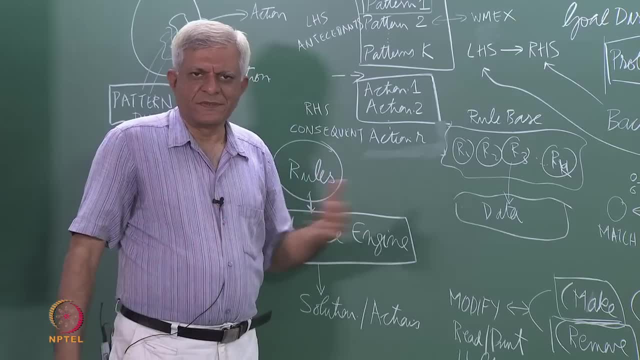 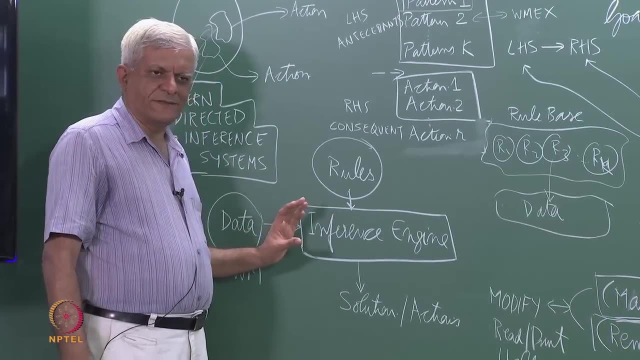 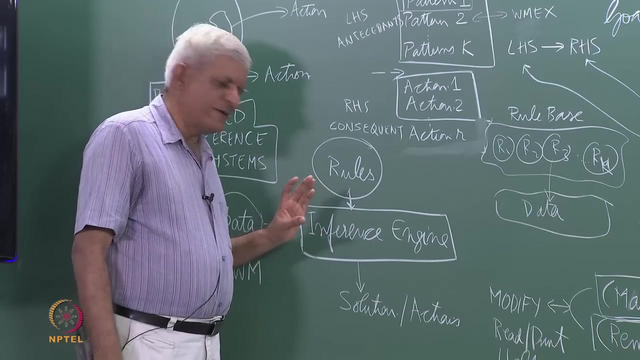 this goal. I can see the goal being achieved. then halt, essentially, you do not have to keep running the program essentially. So in the next class we will look inside this influence engine and it is a very well known algorithm which is very popular and has extensive use in the industry.